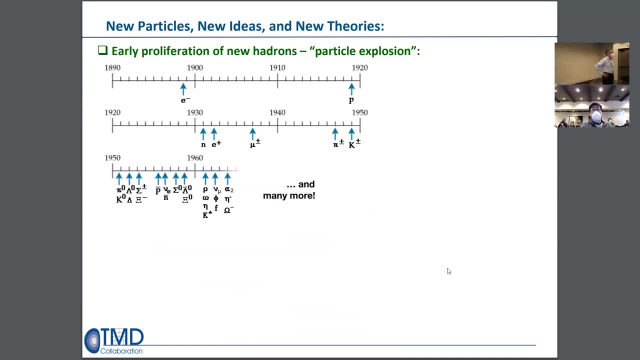 A little bit history of the particle physics, how we end up with QCD as a theory for strong interactions. Strong interaction means we're dealing with the hadrons. Then when was the first time we see the hadrons? Well, if you look at the history, then the way it traces back way before the 1920,. 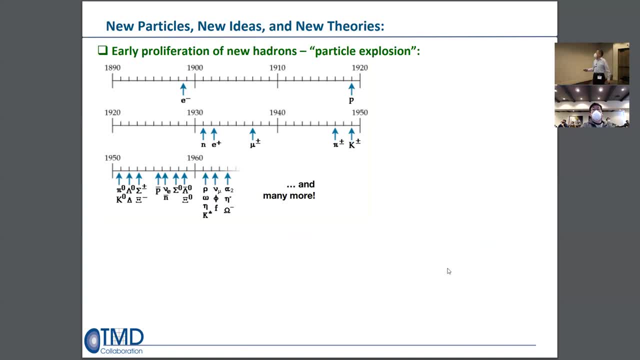 we decided: well, we're going to discover the proton, That's the hadron Right. Then eventually we decide lepton. Then of course we have electrons and all the neutrons, the next one. But what's interesting, in the 1950s, 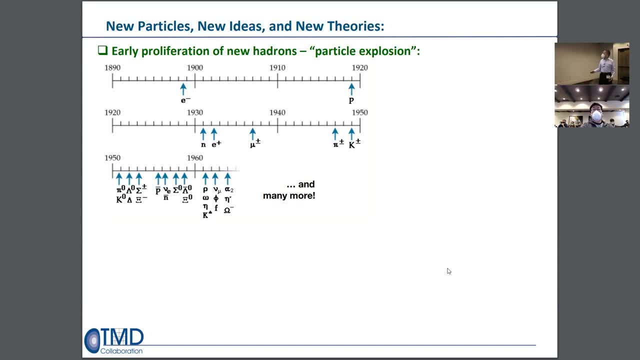 we have a bunch of the particles. So that's a really the sort of I say it's a- particle explosions, that really lots of them. Then a question is in seventies, after 20 years. So then you will find that. then you find a bunch of the more particles. 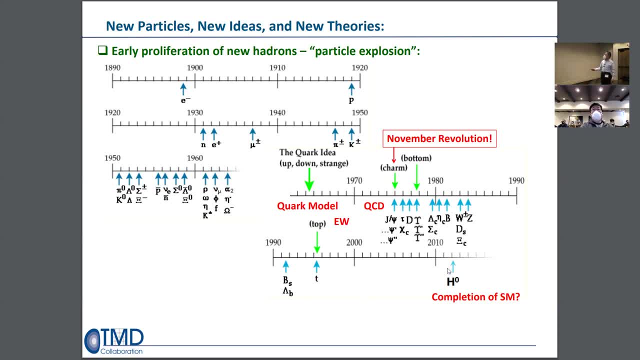 Involving the heavy flavors. I will tell you later. So in this case, after we these particles, the people try to understand how to make this sense of these particles. Then that was a discovery of the quark model. I will tell you in a moment. 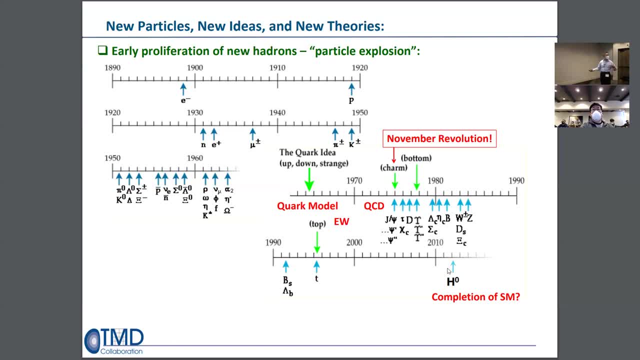 Then, eventually, we find the QCD, because the quark model does not give you any dynamics: how you hold the quark together. So then you discover another level of the particle involving the heavy flavors. That's known as the November revolutions. Well, 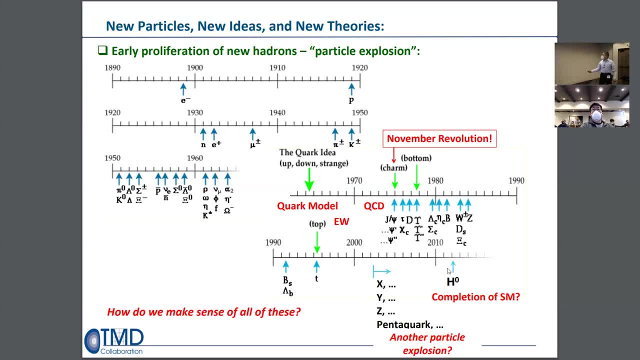 recently in the two. then we have a new set of particle discovered, known as X, Y, Z particles. The question is: should we have another particle explosions? We don't know yet That could be Then. So the question is: 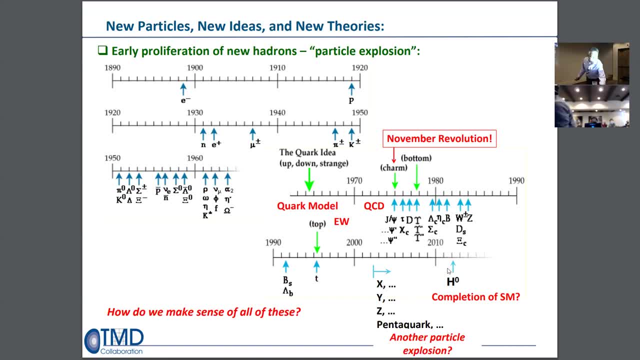 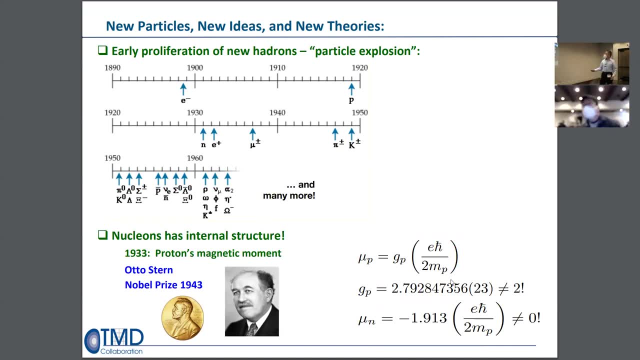 how do we make sense of all of these? So those are the little bit history. So then we back say, okay, theorists never stop. If you have some phenomena, theorists, we work on it. The states, the very early 1933,. 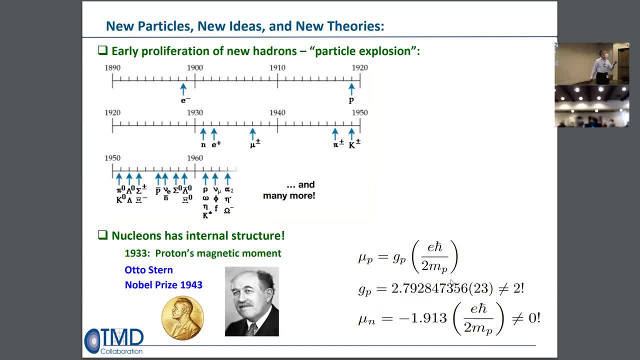 we noticed, the nucleons are not elementary particles. We know the electrons. Neutron is known as elemental particle. Nuclear means the proton Neutron have to have internal structure. How can you tell- Well, that's a lead to Nobel prize- that because they can measure the magnetic moment of proton. 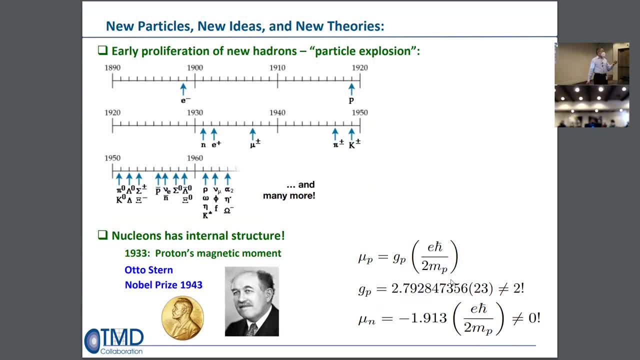 the neutron, as we learned from direct theory that if you spin half particle, if your point like your, this magnetic moment, the G is equal to two. Well, you find the proton is not equal to and a neutral has no charge. 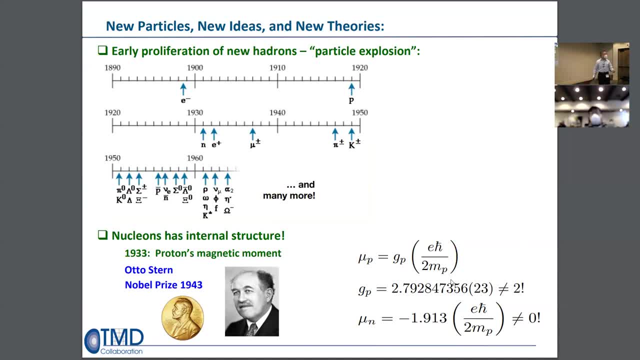 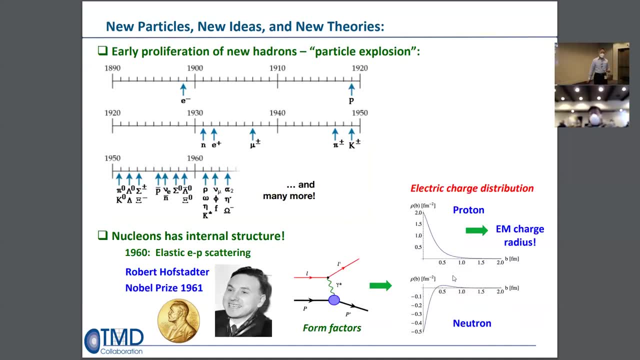 Then there should be zero. Well, it's not zero either. So that means that the proton is composite particles cannot be the point like like electrons. Now, further, we find that there is a nuclear have to have internal structure In addition to just say 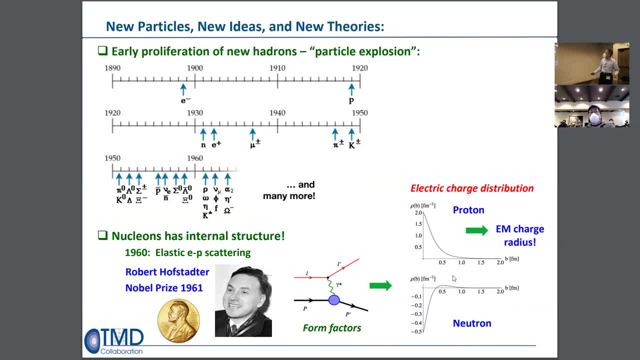 okay, the magnet moment not equal to G, not equal to two. So what I find is they do the elastic scattering electron, a proton. Normally you will measure the form factor, You have a charge distributions. Then you will find that the charge distribution for the neutron 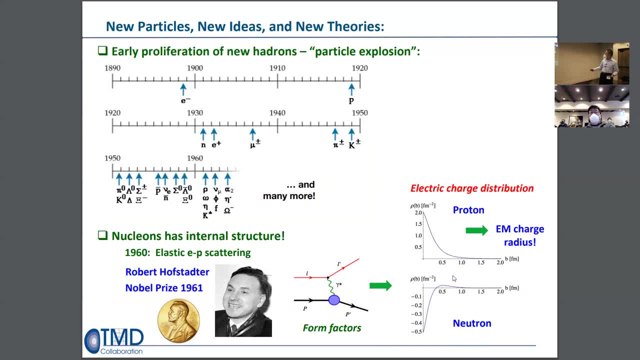 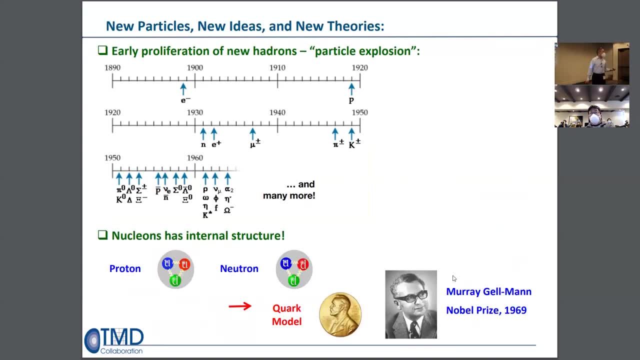 neutron zero right. Well, if you have a very intriguing charging distribution, there must be the internal structures. Then those are the history. Then I'll let you the pork model, which is invented by Gilman in the way in the sixties. 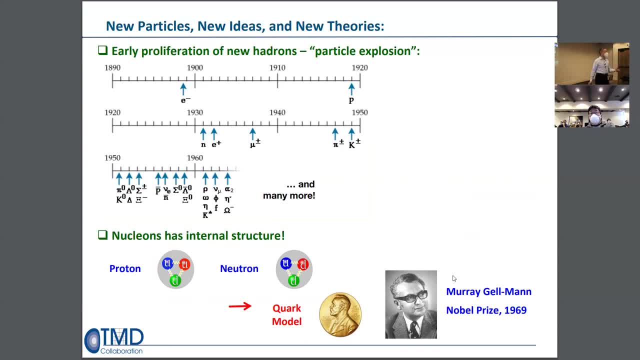 Then what? the idea is a very simple. they say, well, proton, you try not element particles, but they made all of us being half point like particles known as the corks. So that's a model, is a very simple: The proton made of three corks. 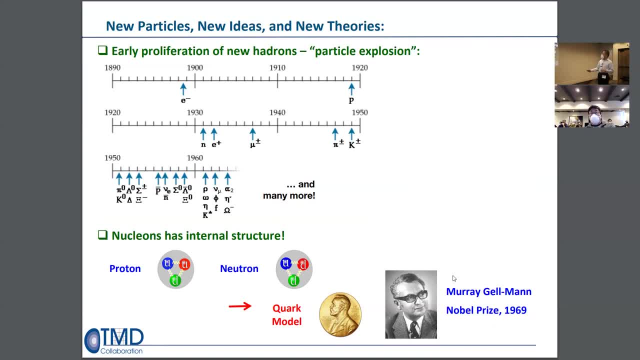 two up, two up cork, one down cork, again three corks, two down corks, one up corks, but the corks spin half particle by with fractional charge. By that time nobody there to say that is fractional charge. 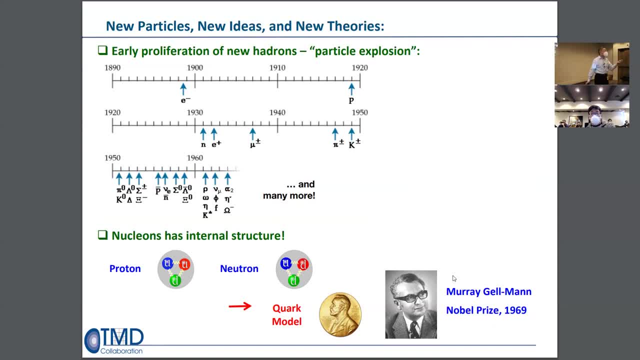 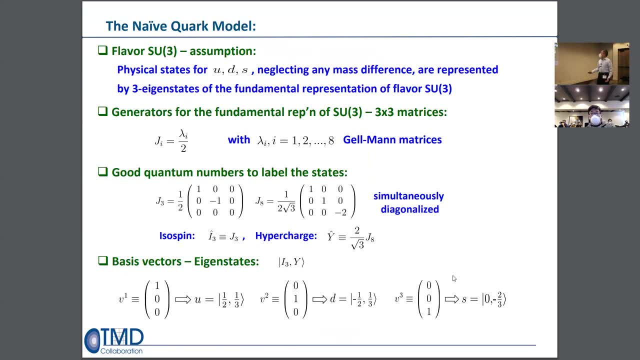 Everything is made measured by electric charge, the charge of electrons in the units of that. Well, okay, I'm going to say they had to be fractional Then. that his idea is a very simple. Ooh, to my grace, the price suddenly worked a little bit. 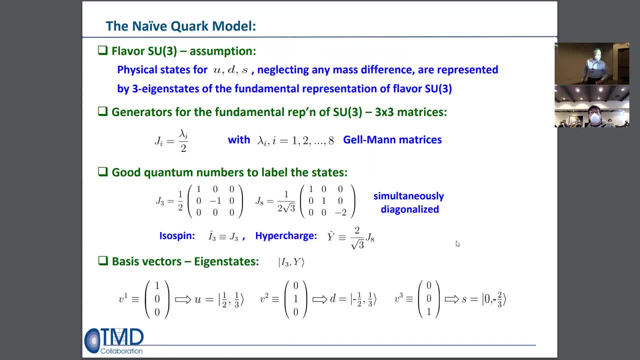 but it doesn't work well. So what idea is to say? well, actually that's three corks up down. strange, They're putting the flavor: different type of the core, different flavor, SU three, symmetry, If you neglect the mass difference between those three corks. 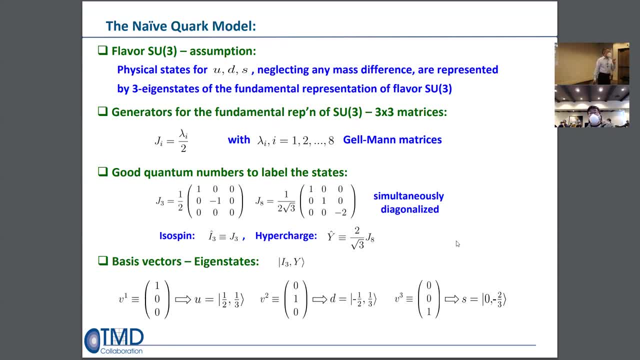 then he say the corks other elements, then the proton neutral composite. they are corresponding to the so-called the eigenstates of the fundamental representation of a three in terms of certain continent. But we know that from SU three most of you probably learned that two. 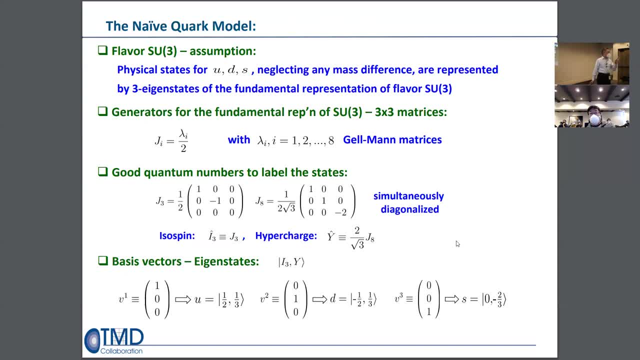 there's eight generators, Two of them can be diagonal simultaneously. That means you can define the state in terms of those two quantum numbers known as isospin and the hypercharge. So you will find that this you can be basic vector for the eigenstate defined in terms of the quantum. 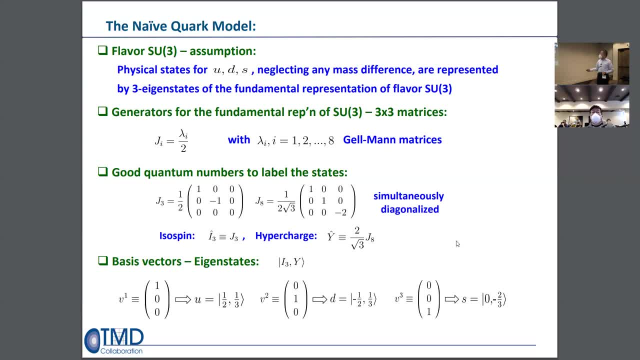 number isospin and the, the, these hypercharges. Now you will find that one is a one, zero, zero. natural is a half, three, one third. Then that's a tongue. Okay, So that's how he started. 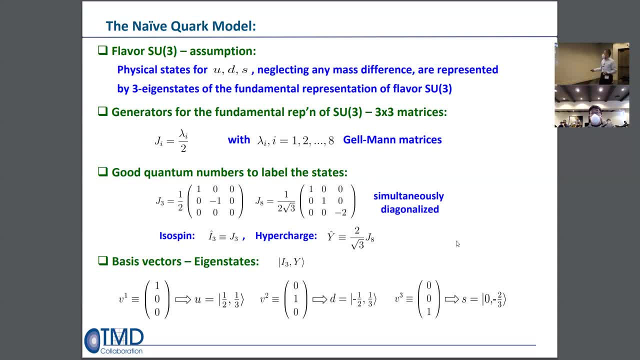 Now you can see from this magic how he built up the proton and neutral in this very simple model. Well, if we now put in this space isospin and the hypercharge, there's three core crystalline, three points on this phase space. 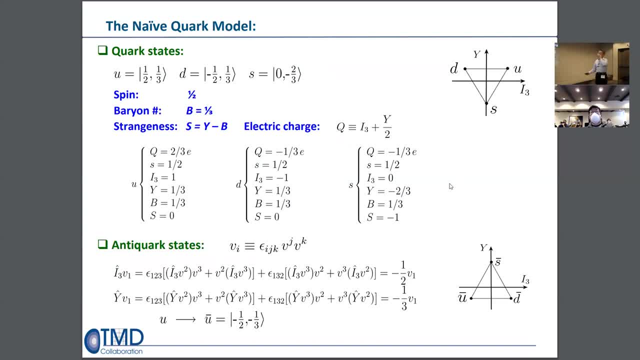 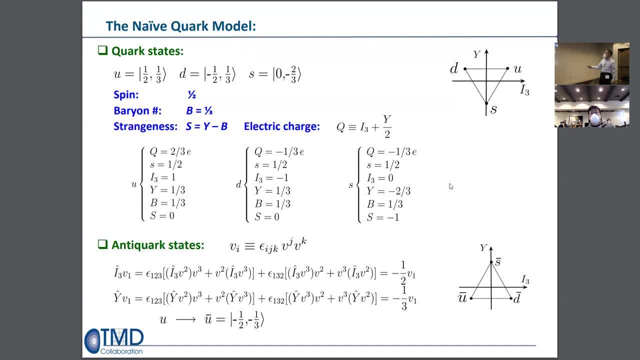 you know you could call this is the hypercharge minus barrel Number- that the electrolyte is defined by the- this is been plus the, the hypercharge to run it to then those that are quantum number, which is exactly for the corpse. 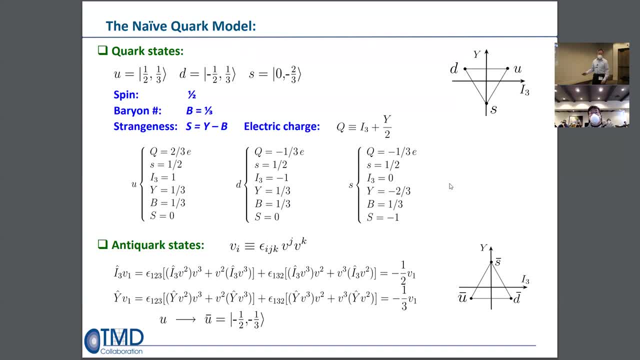 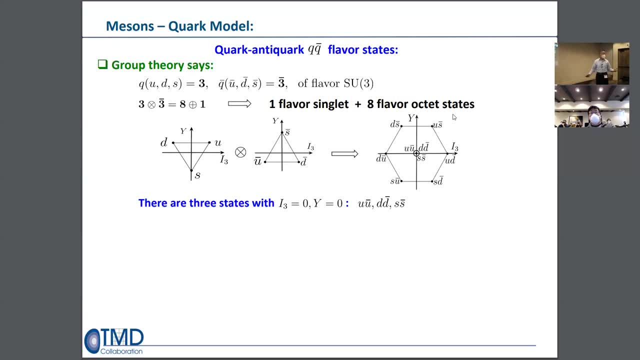 Then the. then you can do that and take quotes from these. You could beat up all the particles. No, At that time. So he said, madam, What's the matter? Samarine, pion, traon, all those metals. 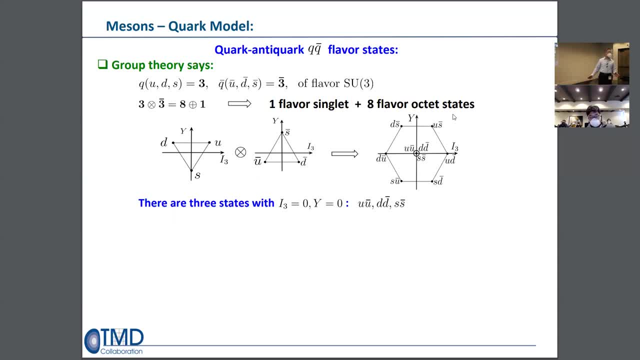 All the matter made of the cork, anti cork flavor stage. so you will have the combine it. so cork have three flavors and tech works, I have an anti. three flavors. We combine two together. you can have, you know, from group theory become the a plus one. so you combine these two triangle together, you will have this state. then the state can be interpreted. this is from a purely from a group theory. 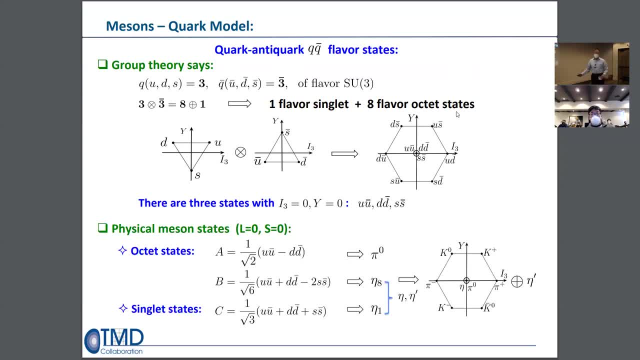 What about corresponding to real physical quantities? you will find, in terms of the optimal interpretation, this eight was known as octet. You have for the corner. if I say l equal to zero, zero state, you will have a. can you have a K zero, K plus neither. where the pioneers say: this is the pion, the pie zero plus the K minus cake, that other states. 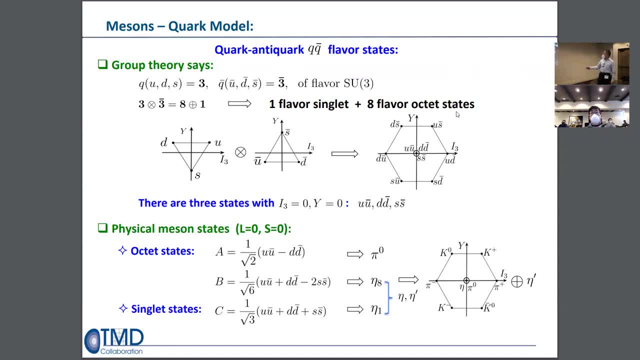 So in the middle you have a three state. they all have a zero. so then you can have A put in octet. there are two version is super position of that can apply zero on the eight, eight. then also that sort of single estate, this little one single estate. 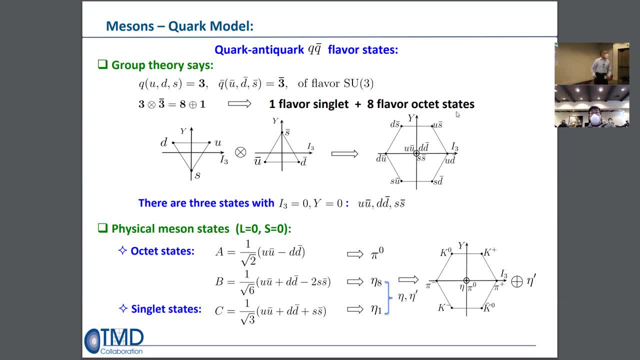 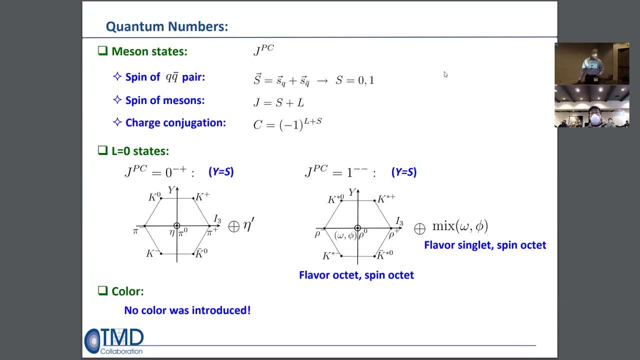 gave it a to one or super position, with that eight, eight apart. so this is a very simple picture. you can build up all the nomads on the time plus many others. I just gave away example Then. then you can see the quantum number for all. the state you can speak is a super position of a quote and quote. 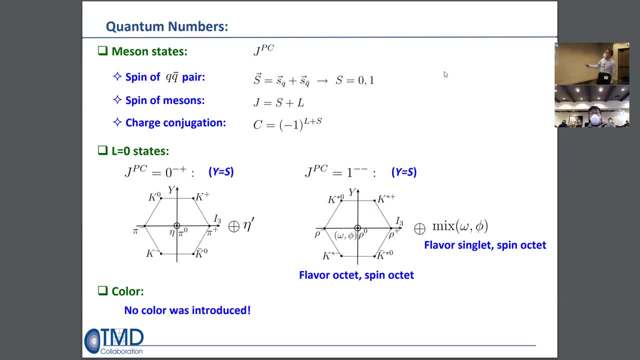 As you know, is the quantum mechanics sq. You can spin 01. then you have spin of the metal, is s plus l, l orbiting and momentum. so the charge is exactly minus the one, The l plus s. then you can have equity zero state, the one I just show you. you can also do the l equal to one state, jpc. they can have other state. you know now that this point there is no, no color yet. 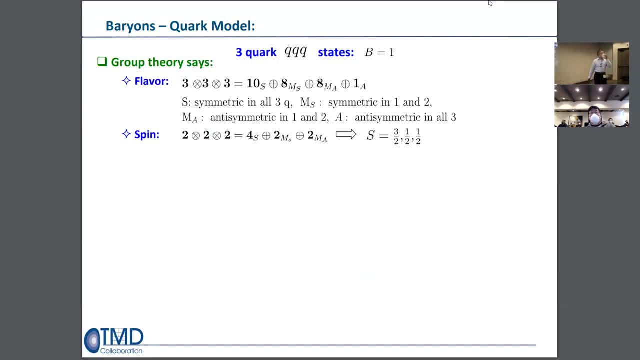 What about barriers? well, he's, that's exactly what he said. The proton neutral middle of a three quarks- that's a better number- is the one third for each quark. so the sequel state from group theory, you know the three together you can have a super, you can have some of the. 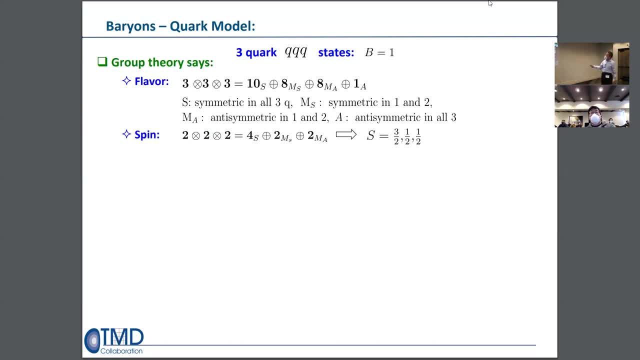 This state. then there's been the same thing to compose. you combine together, you have lots of states. well, let's see what happened Now. you can physical state, for example, the one we familiar ways, the neutron, proton, and also Sigma and a cascade. then this exactly how you combine. 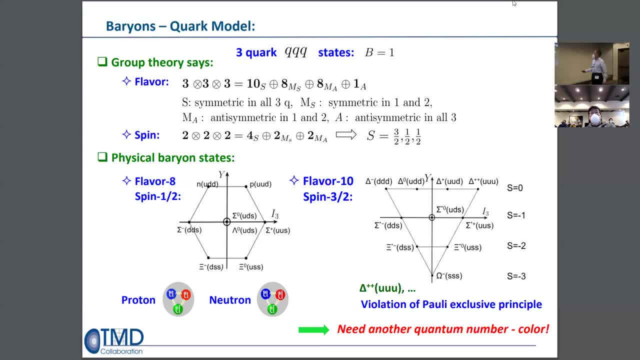 So you can have They. that's been three half state. and this is exactly. you know. they have delta, Sigma, cascade, the omegas. well, here comes the problem. this Sometime problem is a bad problem is very good because there's a challenge. you will have to solve the problem. so in this case you immediately realize if you look at that plus plus, if the ground state there's three, you quarks, quark the declared as being half particle. 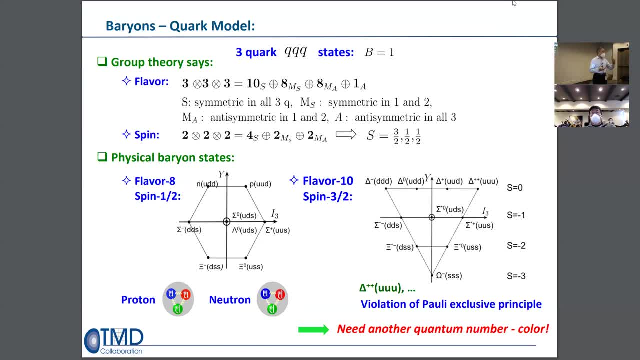 They are all in the ground state. quark have spin half. you only have two states. how can you have three? then the problem, finally the this accrues principle. so then then what happened? we need another quantum number. that's exactly how the color came. 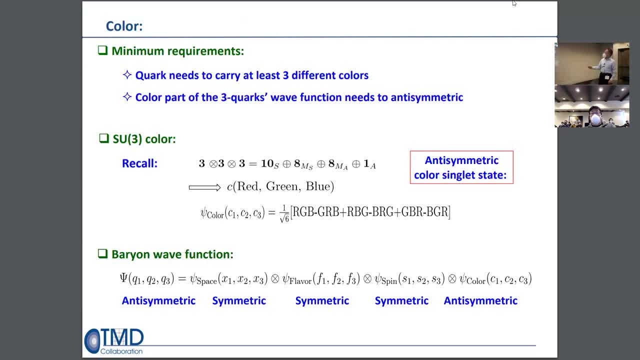 So what is the minimum requirement for the color, the new quantum number? we at least have to have three. that's important because you have a, you call in the same state or make out of three estate, then you also have a color with us record way for how to be a person matter. 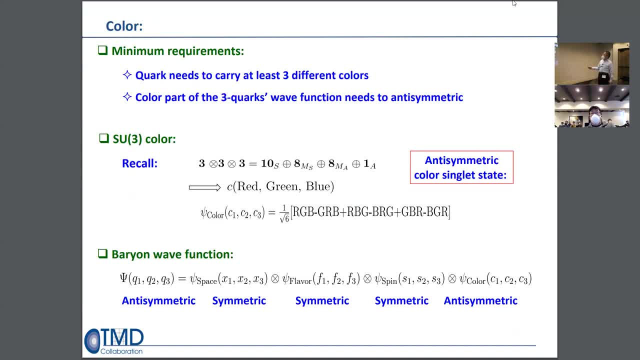 So if I can imagine as you see color, you can put three quality go togethers. if the color the three, again you have this color state That you don't want because we never see any specific color state support. we take a call, a single mistake. then that can be constructed by the anti symmetric pencil so the barrier wave function be constructed as a street core. 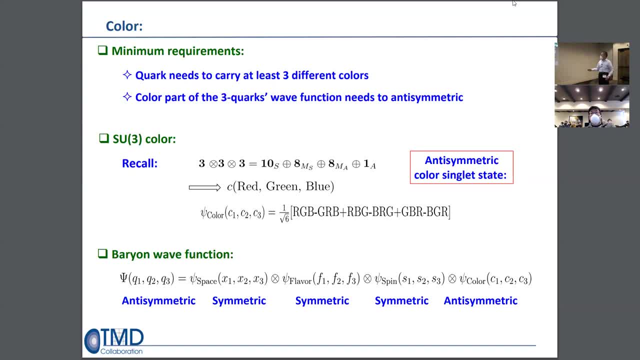 They have a space pop, it's a ground state. okay. symmetric flavor pot: if a three you quark. or equal. symmetric the spin pot, you put the lowest energy state. symmetric: I can get anti symmetry well from color. so that's how you construct the. this very on the wave function at that time in the 16th. 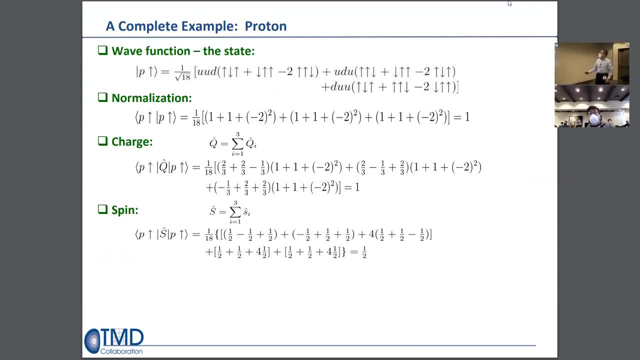 Now I give you a complete example. you can work it out very easily. say the proton, then we function is, you have a spin pot, this is being, we have a flavor pot. you combine together cork is color is at a symmetric, Then you normalize to what? so you check it. well, that's good normally, to what? what's the charge? we know that in the quantum mechanics it's an operator sandwiched between the state. 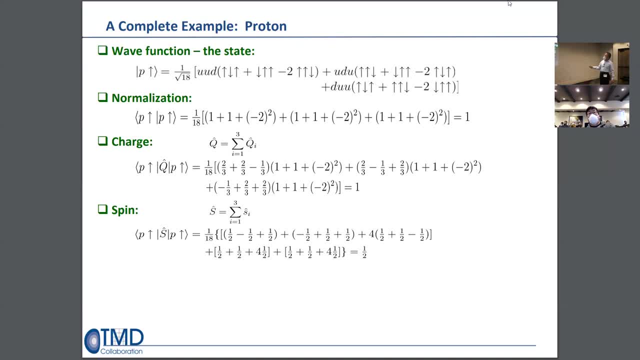 So that's some of the charge of individual cork. you add them to where you go, to what the wonderful. what our Spain you are. same thing, quantum mechanics. you spin operator sandwiched between a proton state, then all the corks that's been have. you do, that is with. you know the wave function, you calculate, everything's been happy, wonderful. 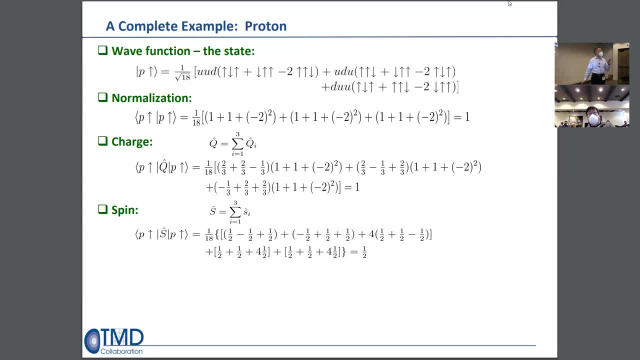 Most of the Challenging part- that's how God we started- is a magnet moment. well, magnet moment, we know again. you use the operator for magnet moment, the individual cork. You have a proton for the proton, then you will have the full magnet for the up cork minus dunk cork. same thing for the neutron. 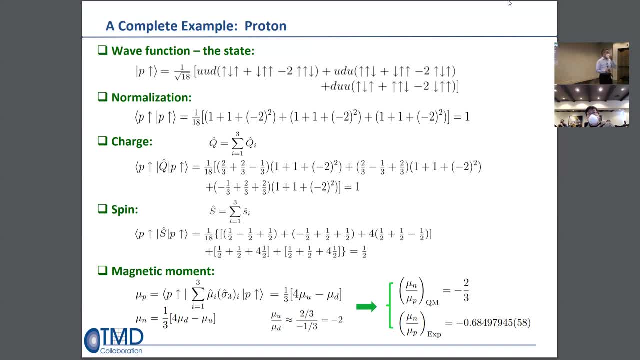 But we don't know what's the magnet moment for individual cork, although we know it's a spin half particle. but at least we know the ratio, The ratio of that theory, because they, they can be kept, this unknown can be canceled, end up with minus two that look at the clock for the content poker model to minus three half. if you do that, then if you think of this point like particle they will find experimentally. 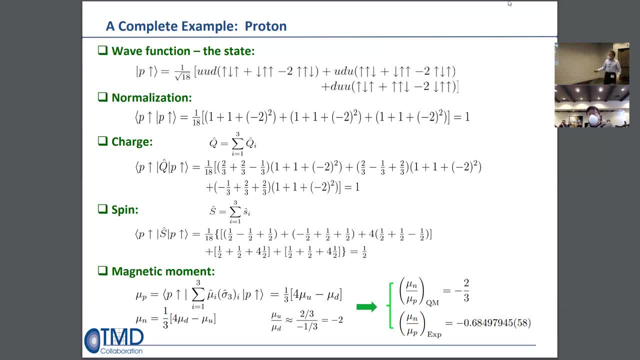 Very, very close. No, it's a, it's a three half. Just second, I only have to- I know you- you up, call you down, yes, then relate to the charge, then. then you end up with this ratio, then you cancel the unknown, then you end up with this number is a very, very consistent. 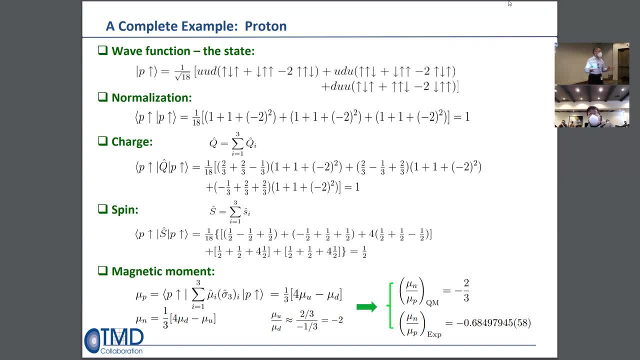 That was a big success. you know, not kill man, receive a Nobel Prize for the Pokemon. but if you think about it, what's the dynamics? you have three cook. what the force to put them together? no answer that time, But Okay, Okay. 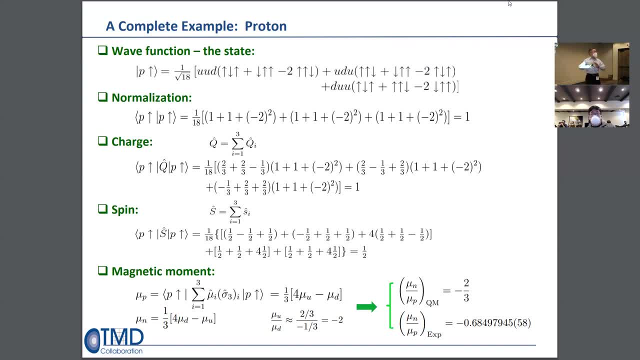 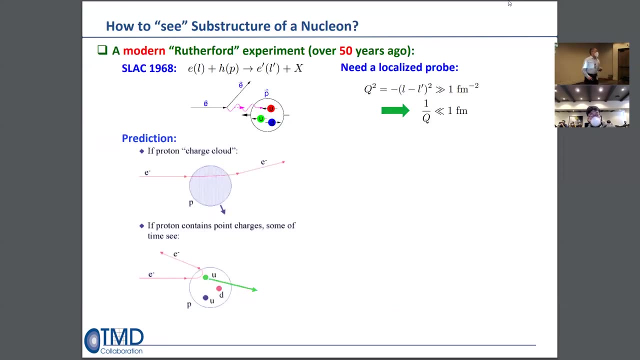 But they. with this simple picture, you explained almost all the quantum composition of the methods, barriers, plus a few. was discovered, like Omega discover later. so that's a wonderful. by the way, the QC car, Well, that's a theory. what about experiment, say? well, you claim proton has internal structure. how can I do the experiment to see them? well, we know the rest of the experiment long time, over 100 years. 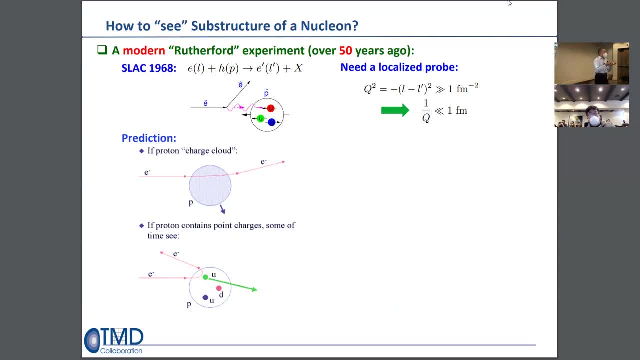 ago. So they say the atoms are made by something with some chart, that maybe that different models and maybe there's a uniform distribute, a sphere or something. But with the roster for experiment you will find a standard of a particle to the Adam ago for you. you see a number of good number of alpha product with with a bounce back with a large angle. 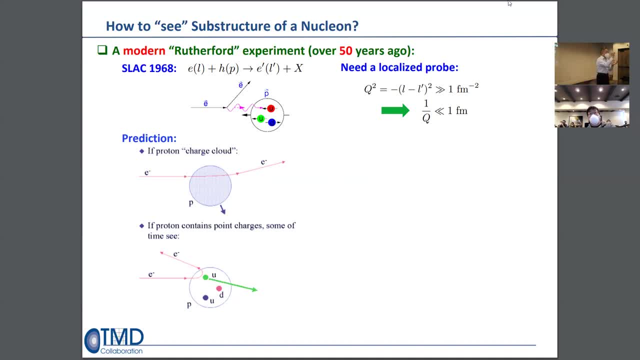 That means inside these Adam, that point like object, so the whatever the particle of a party You come in hit the object so whole they bounce back. imagine you have like a marshmallow type of smooth, uniform ball, The particle coming with energy, with go to fact going through it well as so never really hit the back, so so hard. so there was a discovery in: Adam is not made by uniform distributed metal, rather you have a very, very hardcore know as a nucleus. 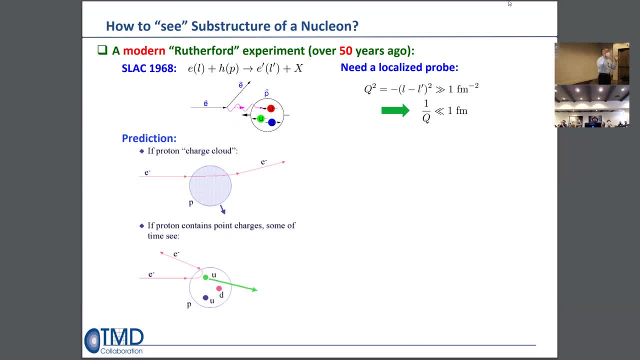 Then with lots, of, lots of empty space The way, the electron floating around. So people try to the same. if you have a charge particle inside the proton spring ham, what can I do? I send a product charge particle a to hit it. that's the exact electron. 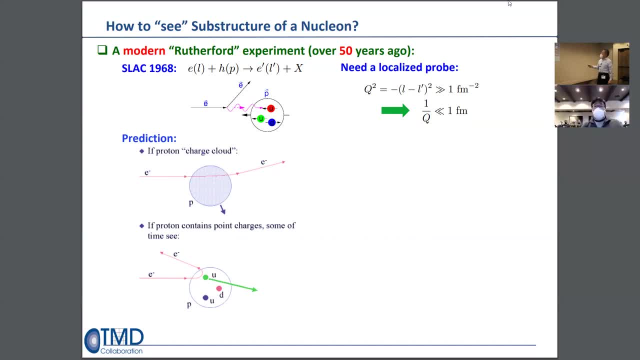 I sent an electronic to hit the proton. then only thing to measure, just a lot of the did measure scale electrons. the scale of half is a very massive momentum transfer known as a Q square. I want to, I want to make the Q square so large, the universe of Q square so much smaller than one for me. side the proton. 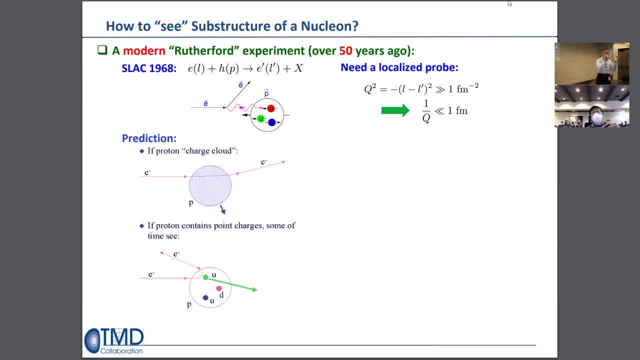 That means I have a pro to see something point like inside a proton. that was. it was a prediction that time. If the plot prototype made off like Adam is a uniformly charged distributed quantities, now you expect electron to go through with some different, you know scary angle that if the 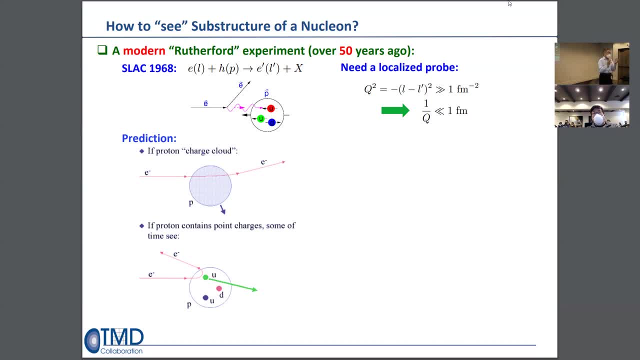 Prototype made by point, like particle, just like Atom. you have a nucleus, then you will see lots of electron going backwards across section with a large momentum transfer will be large, much larger than this one. So that promote the people to do the experiment. no as a slack experiment or modern version of a roster for experiment. 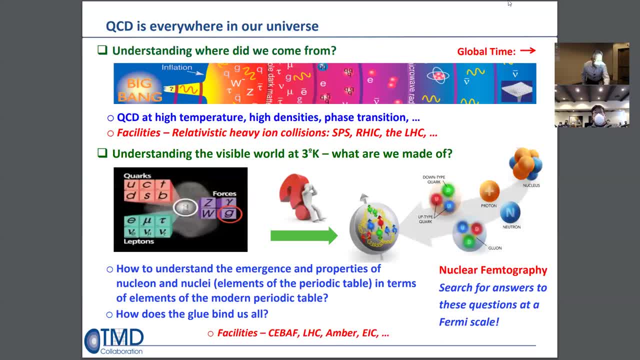 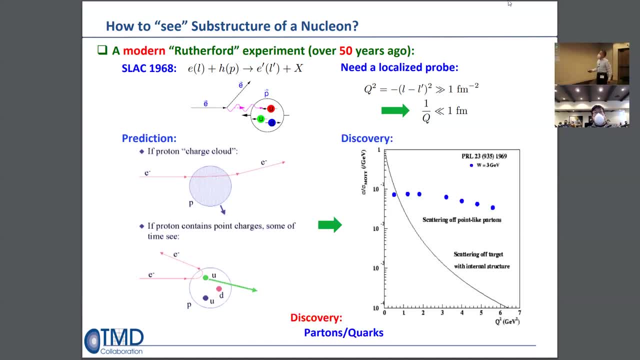 whoops, This thing is so sensitive. what happened? Okay, so here's the discovery. You to the that to the Nobel Prize. then this is a spectrum expected from this kind of distribution. Then what the data shows: when the Q square the law, you expect the distribution falls like a crazy. you will find a crossing so big. 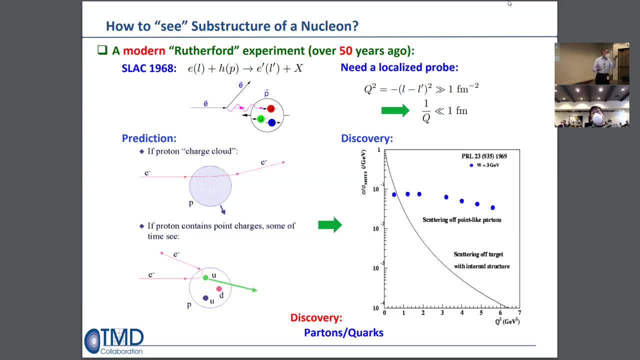 That means just like the rest of a find it there must be pulling like the inside a proton. you hit so hard. you have a large cross sections that led to the discovery of the pattern or cork. you know the history, gal man say. that's a quote. 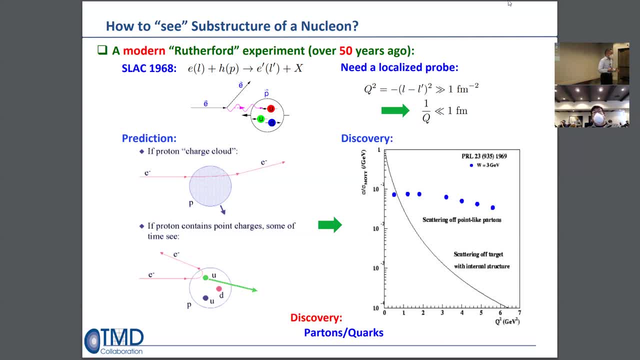 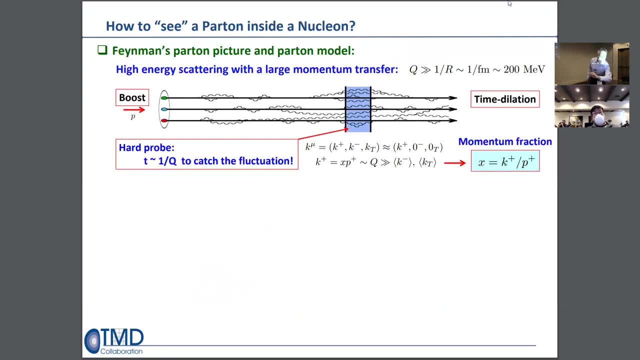 pop fantasy, that's a pop home to have them argue for years, even until they die, then of course. now we we understand better than so. what happened is With these what the famous picture comments, pictures that work with a large momentum transfer. if I stay in the center, my friend, imagine the protocol me very, very fast. 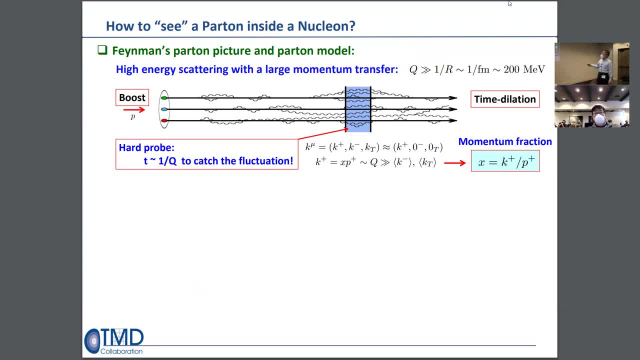 If you come in very fast, they imagine you have a quantum fluctuation. you have, if you have Famities, not say Three corpse basis some patterns inside it, so you have some kind of quantum fluctuation. days in the hub probe had interaction time so short. 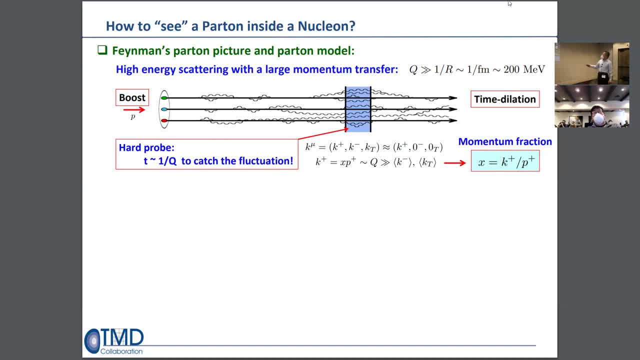 They can effectively catch the fluctuations. you will see the momentum, the partner in this direction, the K, has a possible mentor in the like component Minds, component transfer component. if they move so fast, no typical transfers. momentum is order one for me, now over for me. 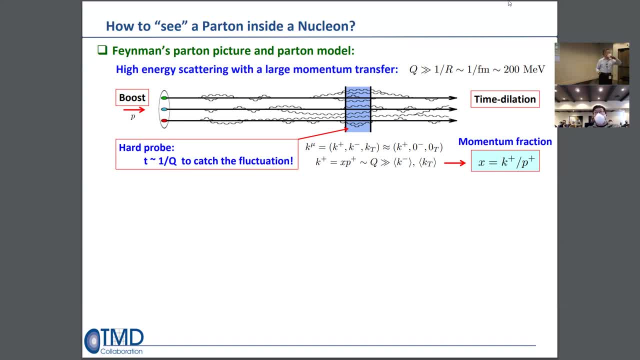 Then then what? the non general mandate, Because that's a moment in transfer you have is so much larger than when for me, so in that case you can make approximation. the patterns of momentum is almost the core linear to initial proton momentum order of a queue, so much larger than transfers momentum as well as a minus component. so can you use a variable known as a momentum fraction X, define the ratio of the largest component, K plus of a P plus, if these things moving that direction. so basically, idea of man has that. 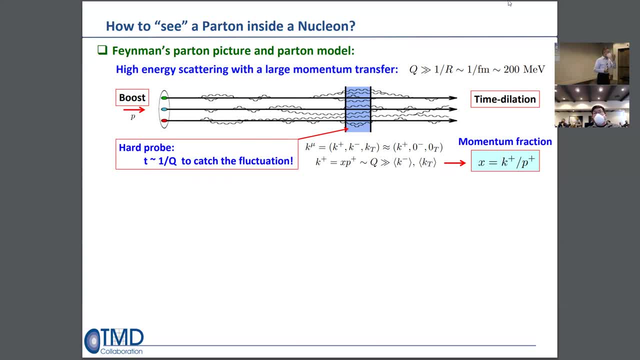 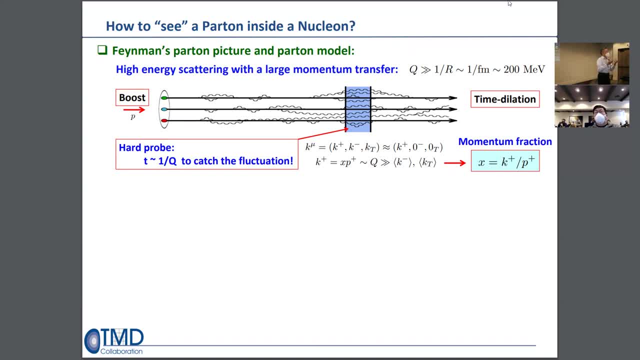 The interaction between them is all the warmer. for me that's the size of a proton. so if the interaction time so much shorter, Then the time at the time for the dynamics of the inside the proton you can imagine. during the interaction time the rest of them effectively flow them. So his picture is the following. 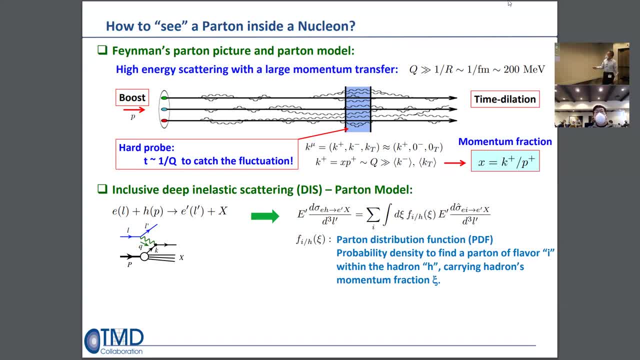 So what really happened for this experiment? he said, instead of hitting the full protein, hit the single wall of them. rest of them effectively flow them. So the cross-section for electron on the hadron is approximately equal to the cross-section electron on an individual. 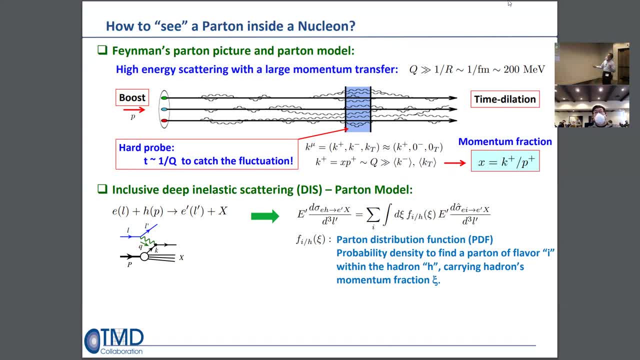 proton, the same invariant cross-section. multiply the probability, density, integral order, whatever momentum fraction, to find this python. So that's his pictures. So what do you measure is effectively equal to the probability to find a single particle. 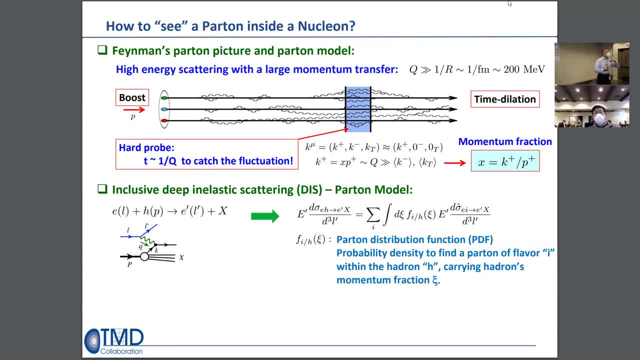 localized, that's probability. multiply the elastic scattering between electrons, that single charged particle. So with this known as this he called as a proton distribution. then you know how to calculate electron scatter of a proton with a charge: elastic scattering. So you can calculate. 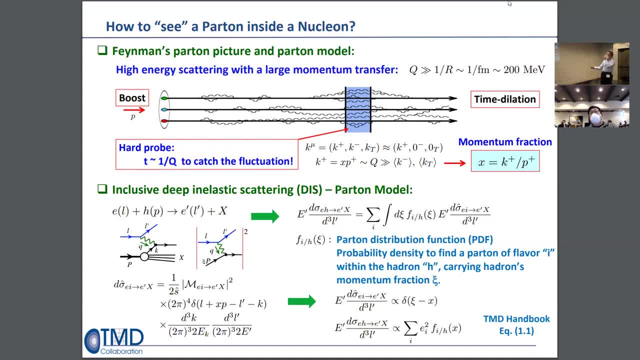 very quickly. So you're going to have to. how to calculate your electron? scatter some proton with some momentum fraction. You square the amplitude, you get a cross-section, you get the wall of the flux. square amplitude, multiply phase space, integral the phase space, you calculate immediately. 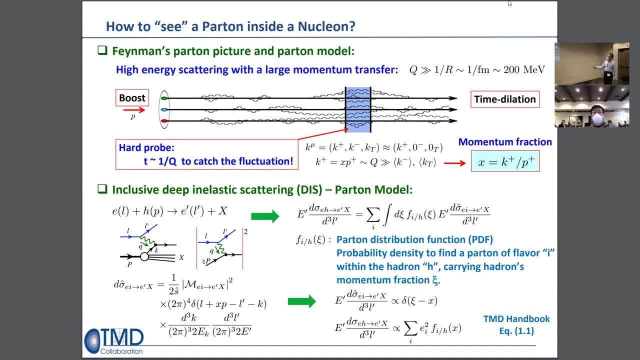 the potonica level in the proportional delta function. So momentum fraction has to be equal to whatever x, then your total cross actually is because delta function fix that convolution, fix this integral. so your cross section, exactly proportional, fractional charge time intensity, probability, to find that pattern. 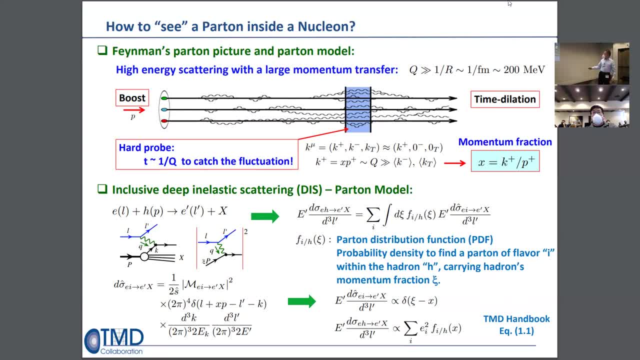 at that momentum fraction. so that's exactly model. the pattern order: it's in the handbook, equation 1.1. so that's the famous pattern model picture. idea is very simple. you have a very hard collision. rest of things. say: the hydrant is effectively frozen, you pick up the one have. 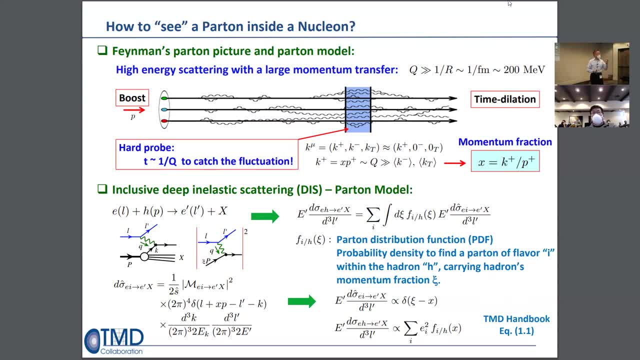 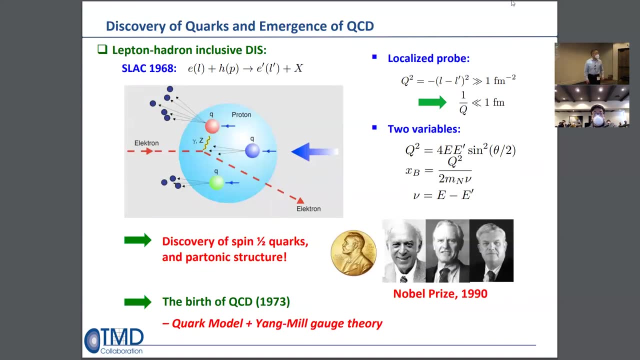 hard collision. then you calculate the scale in between your probe and to the heart pattern, then immediately get your cross section. multiply probability density to go to all the phase space. you get the physical cross sections. so that was a very, very successful. to explain it theorists, explain it nobody. the experiment of the experiment then receive a nobel price. then 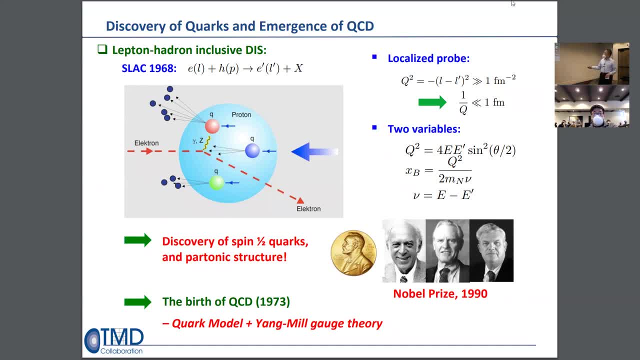 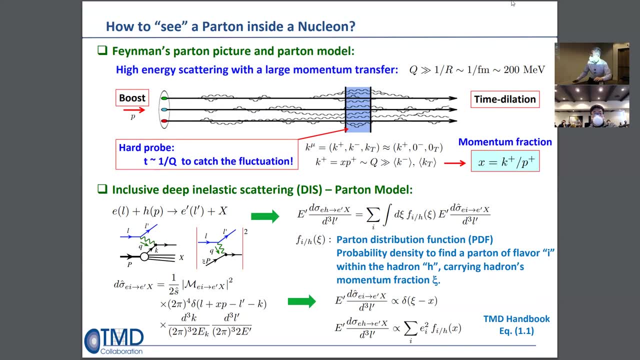 also. you can tell you a little bit later they can. theorists can show exchange particles. you, that calculation depend on the spin. if you do this calculation, you, you, it's a sensitive spin of this particle. that's a homework. you can do this scary cross-section. assume this is a spin half. 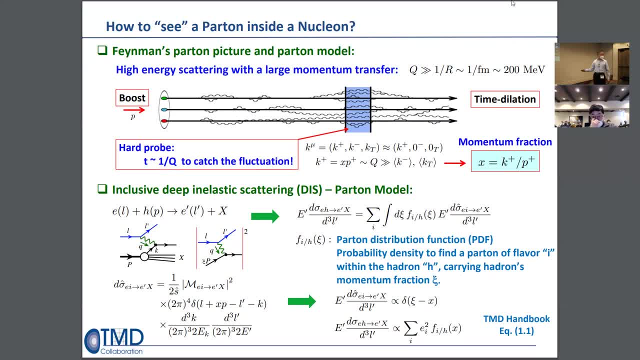 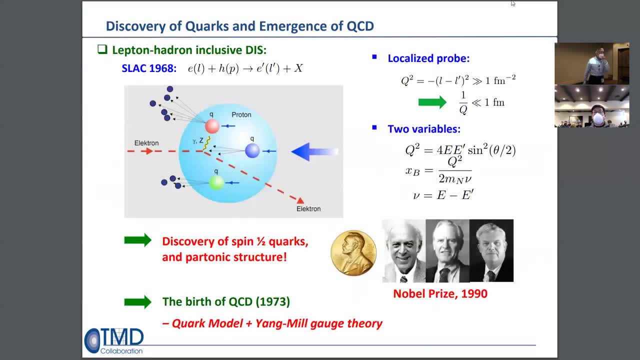 also you can assume this is spins zero scalar. now you immediately derive this to a slight difference. so you do immediately. you can compare with experiment. then people find it: well, it's a spin half. so by that time it's discovered spin half corks. then you have a platonic structure. does the? 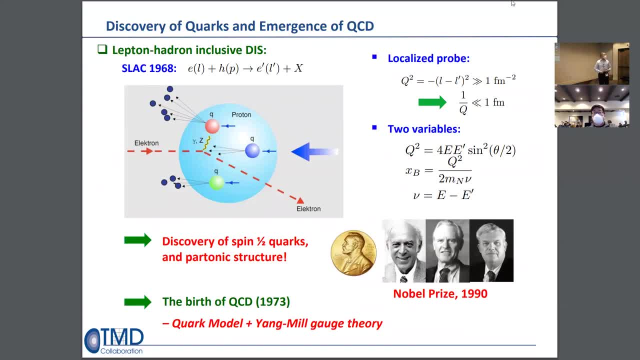 proton have a platonic structure, then of course the immediate people ask they have to get what's the force behind it to hold this together? that led to the discovery of birth of a qcd, which is factory combination of the cork model plus yamil gauge theory. so there was a little bit history. 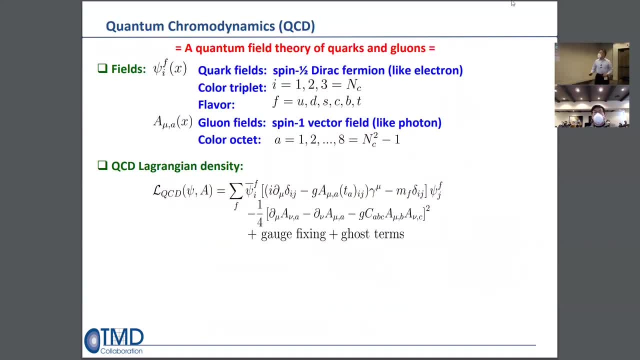 lead to the qcd. so now here is a qcd, qcd that made of the gauge theory, made of a core field, spin, half field, with a different flavor, so far we know as six and also color. so in the fundamental mean the three colors, you have a gruans grew on category eight colors, then you lagrangian look. 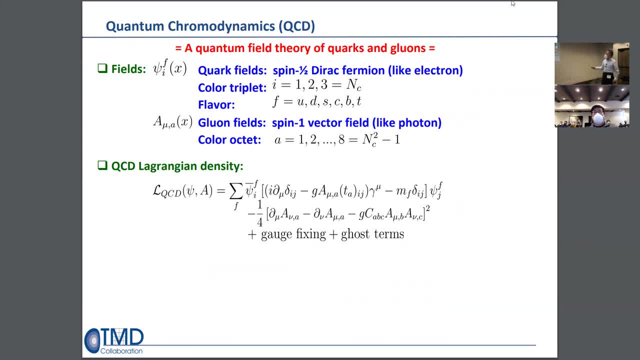 very simple. you have a kinetic term, mass turn, and the ground interaction term, actually ground kinetic chain as well. the interaction term will mix things together. so i want to compare the qcd. You know, the key is almost look similar than this: the kinetic turn, kinetic turn, then the group is a very different from photon. 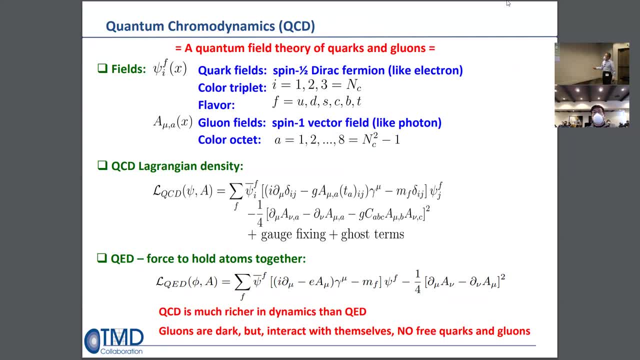 This is a formula we all know me for the electron mechanism but grew on in truck. there's additional term. we expand these. you will find a growing in track among themselves. You all know photon does not interact with photo. that's why the inside Adam you can have a lot of empty space. you can have, you know, photon floating around. but you can define this quantum orbits of photon because photo doesn't interact themselves. they have to go through the charge. 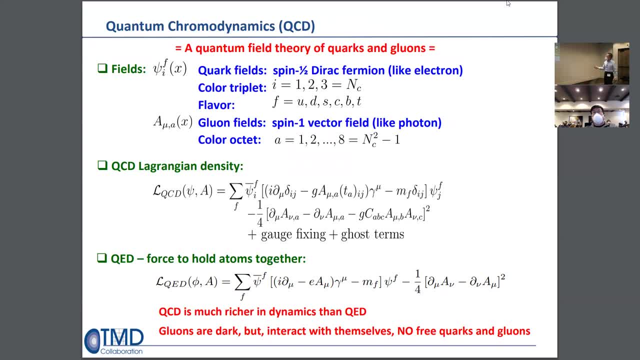 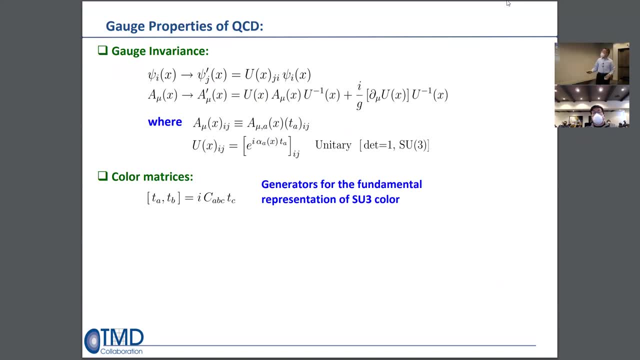 But gruel is different. it is. this difference leads to tremendous difference. so let me quickly go through. there's some basic is- i'm not going to spend much time on this, But On it, this gauge of theory, if you make a transformation, then the like PC, like Ronnie, invariant. 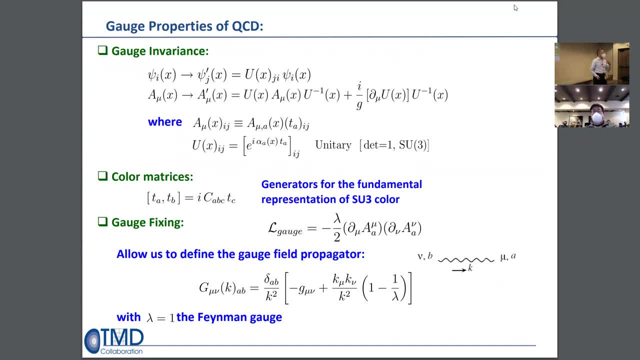 And also you will find that because the gauge sensitivity, you have to fix the gauge, The power, how you do it you can get you fixing the covariant way that lead to the gauge a propagator wrong, propagator dependent choice of a gauge. so this will cover, in the fall lambda, equal one is a circle famine gauge. 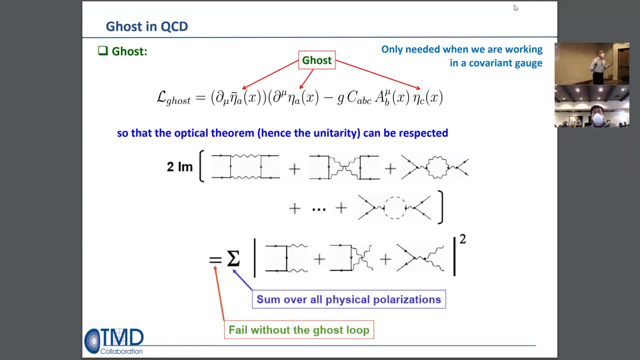 So now one thing is important then: a free lunch. as said earlier, you can. You can choose the gauge whatever you want to. physical quantity should not depend on the choice of a gauge, But if you to the coven gauge, it's very easy to do the calculation. well, you will find that your leader into the extra degree freedom. that's a requirement of the ghost. 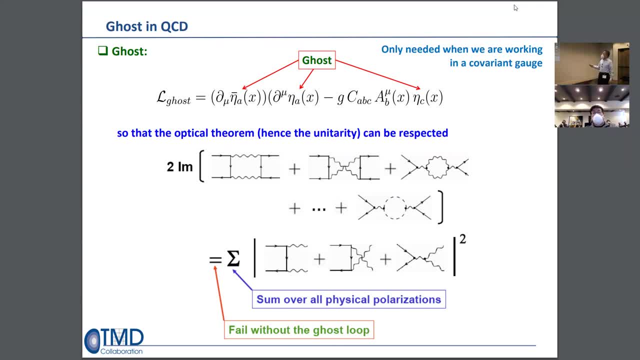 What's the ghost? is the needed when you walk in the covariant gauge. so this is the ghost, like running pot why we need that. well, I gave you a simple example where no, the optical theory you have a. You know that. Imagine part of full scale and put you can be retained from the amplitude square some over the state. 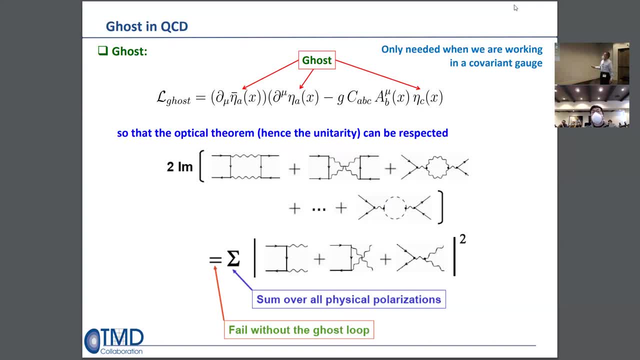 That's optical theory. well, because if you do the coven gauge you realize if you expand the square we're not exactly equal to these. because this has a virtual state, Then because the virtual line- so you have to include this- grew on virtual in the aptitude form you have to have, a gauge goes. 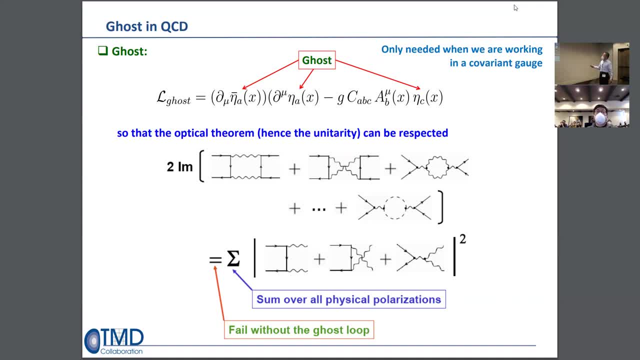 Introduction: the goes to to cancel the physical degree of this grew on so that the imagine part of the force can amplitude equal to the square of the scary up Square. so that's a need of goes to the be careful: if you do the calculation of covering gauge, make sure you go the ghost. 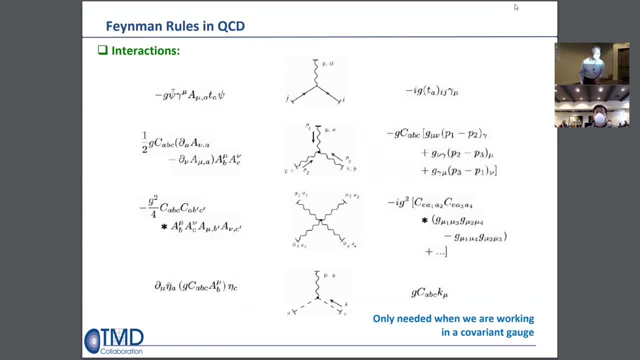 So then the family rule the propagator, then also the, because the ground have self interaction. you have a three growing traction for growing traction And the weather goes. this will lead to the tremendous. This will lead to the tremendous difference between QC, the community. 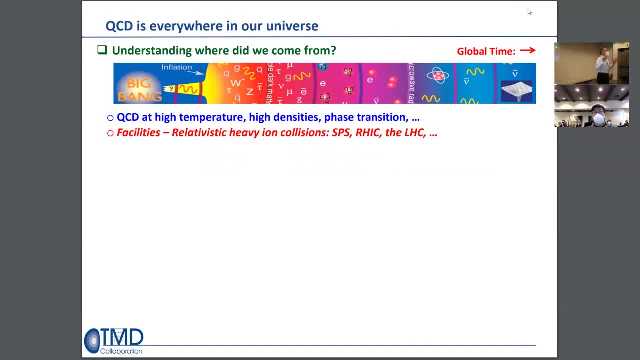 So that here we have QCD. Well, next thing I'll say QCD, the everyone They imagine. we ask a question where we do we come from. we often ask that when the universe started, big band, there is no proton. you know neutral, know people. 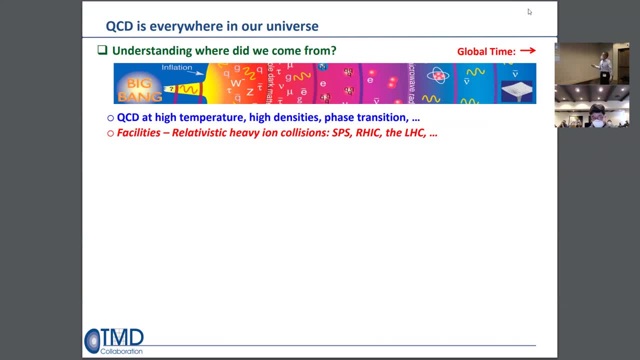 Only thing may have is from the element of particle called screw on. But how the QCD Tells you when the unit for the cool down, How the proton neutral Emerge, They eventually, how the people showed up- We know the later part, biology- people told us 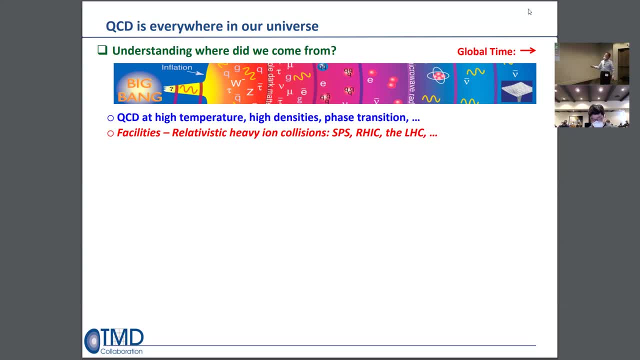 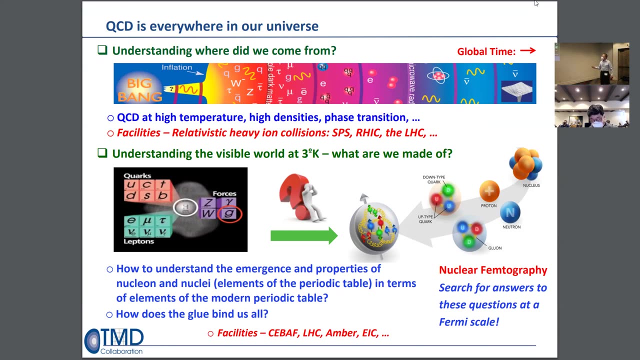 But what about original part, early part? we don't know. That's the motivate, our to do the red, high, heavy and collision to study early universe. Therefore, us for this TMD, we conscious second questions. So suppose that we know, we all what we met off that way. 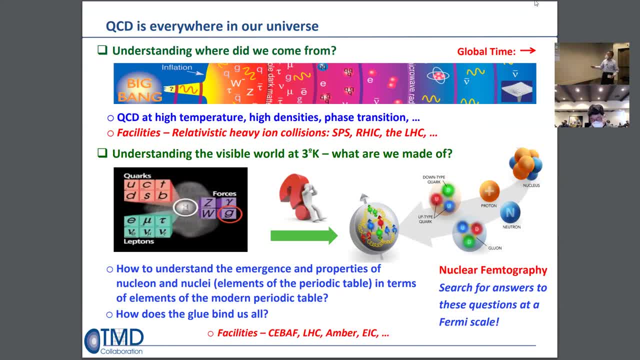 If you look at the new periodic table for particle physics- Here is a periodic table, Here the way are everything, the neutron that start from the. you know the, the question of how to connect this together, How to understand emergence and the property of the nuclear nuclei in terms of the elements of the modern periodic tables. 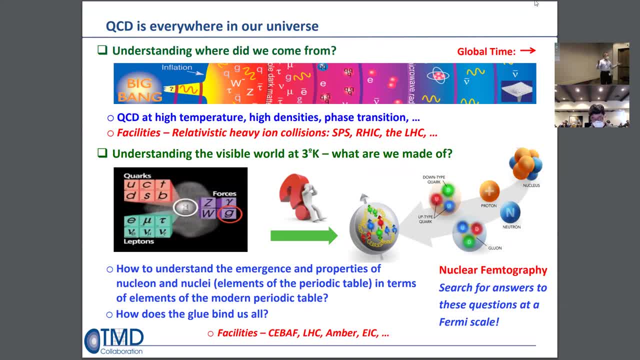 How the grew on the little one here grew everything together. Those are the really difficult questions. Most interesting question was showing directions. Now we have facilities. You see, I'm going to try to study that. There's a new term has been used in last ten years. 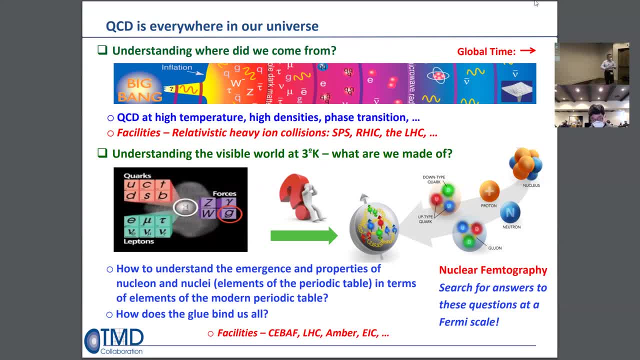 Knows that nuclear photography is, in the sense that branch of the strong traction to search for answers to these questions after the Fermi scale, at the scale of the hydrons. So then the question is: the color? color is a very different from electromagnetic charge. 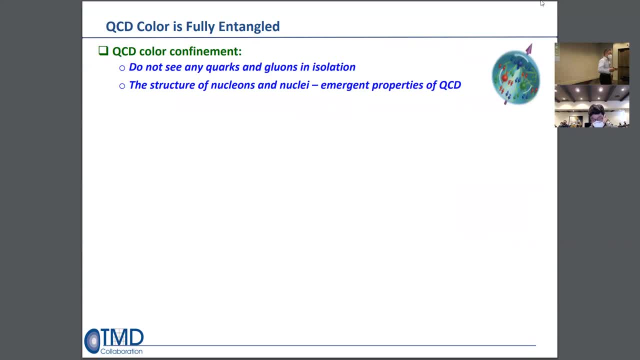 Although it's in some sense similar to just quantum number, represent the strength of interaction, Or the strong interactions. Well, color is confined, Unlike the electron photon. They, because the count that we don't see any corpse growing. isolation. The structure of nuclear. nuclear emerging property of QCD. 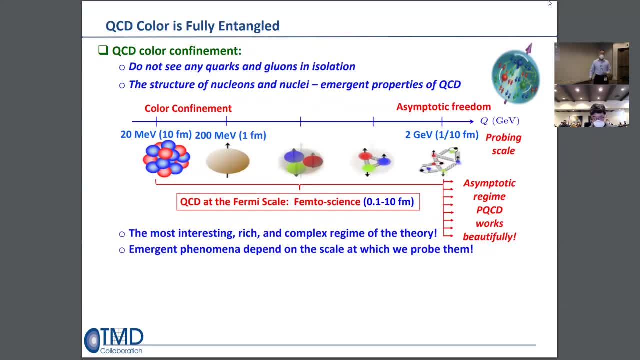 There were even more consequence If you look at the spec landscape of the QCD interaction. This is the area where the nuclei and the nuclear- This is the area we studied in the LTC in the asymptotic region- Then the QCD works well. 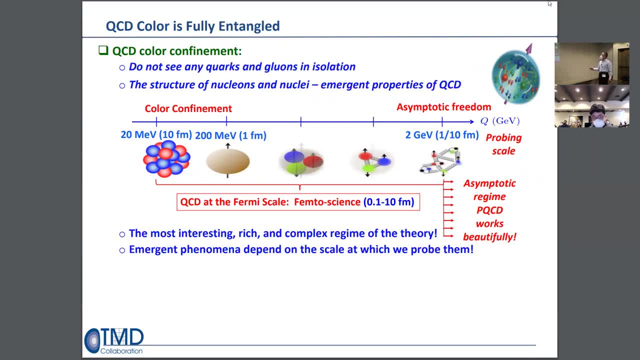 But this is the most rich part of the QCD. We tried to understand the structure of a nuclear nuclear, How they emerge from crazy dynamics. Then one thing I want to bring your attention. We all know these atomic structure. Lots of photographs. 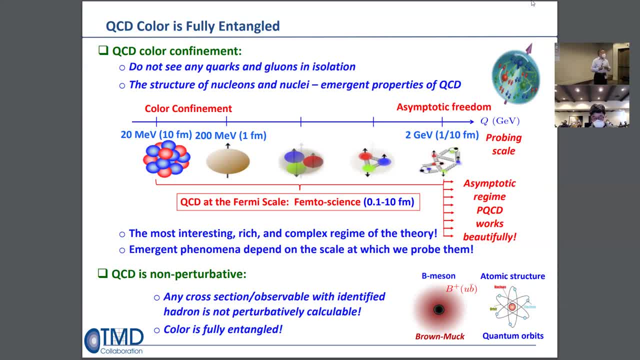 They either call the distance size of the nucleus, Is that kind of the fifth power smaller The size of Adam. So lots, lots of empty space Electron floating around. You have a quantum orbit. You don't have this in QCD. 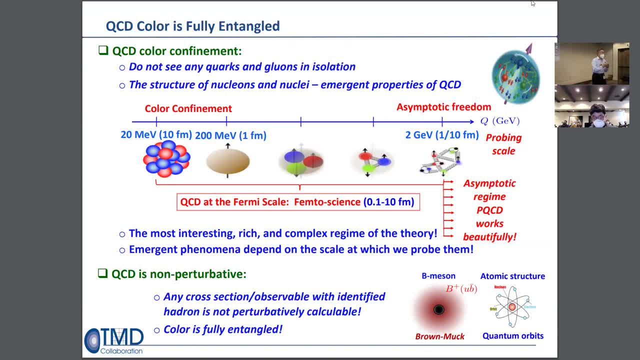 Because the ground carry color. I take the most close example, The beam add-on. You may have a heavy quark or anti-quark, Have a light quark floating around Sounds like a hydrogen atom. No, you don't have this quantum orbit. 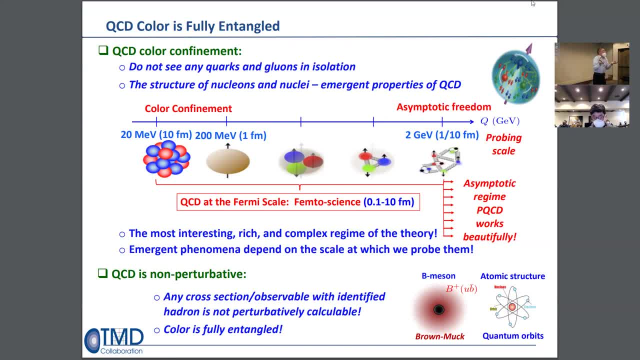 Because they exchange the force, The ground, ground carry color, Ground can flag into the two ground, The pickup pair or the thing, So it's a brown mark. So the structure of the hydron Is very different from the structure of Adam. 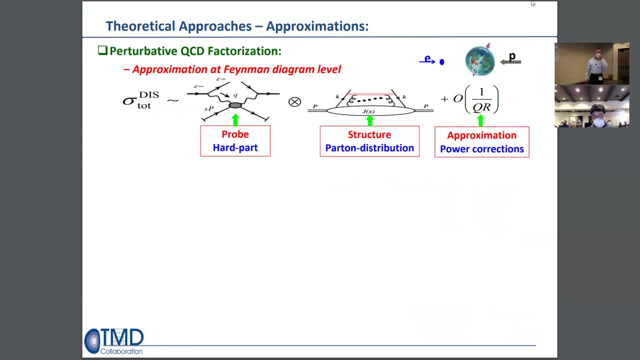 So those are things It's challenging for us to study. So how can we study them? Strong traction is so strong. When the theory was proposed in 1973. Or the end of 1972. Not many people paid too much attention. 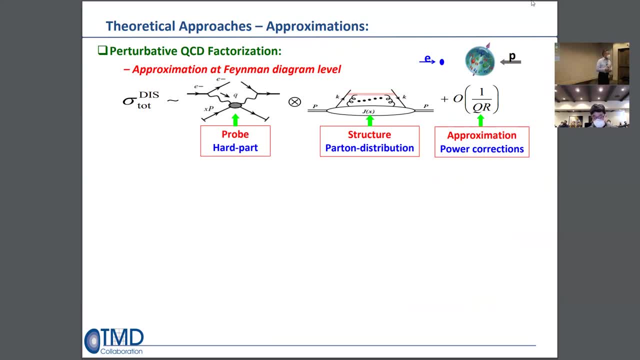 Except the- you know This is a guy, Frank Wichak- As a student. Then David Gross Gave him the problem And David Paul at MIT got a problem. Try to study how the interaction vary At the scale you probe them. 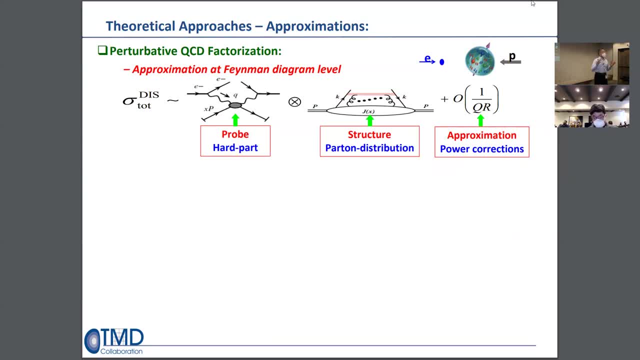 We know in the quantum theory The strong, The strength of interaction is not fixed. Depends on how you probe them. So they studied evolution, Eventually discovered asymptotic freedom. So that means the interaction can be very weak At the shorter and shorter distance. 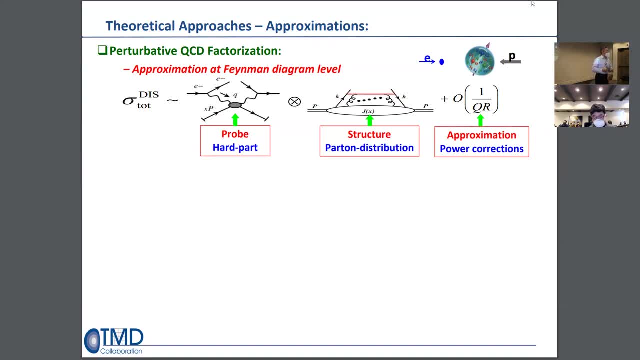 So theory approach to strong traction- That can be debriefing to several things- Approaches Way is known as a perturb QCD function And it's a very interesting theory Because You know Part of the approach. Why do you talk about the perturb QCD factorization? 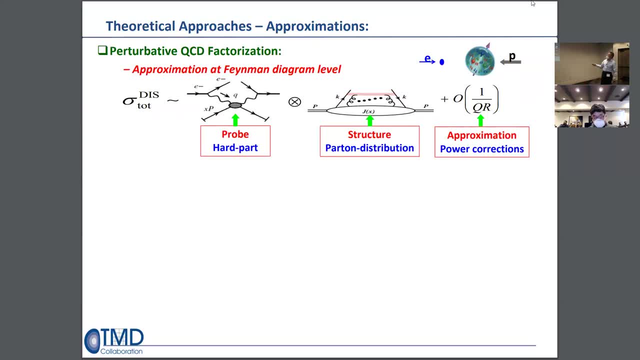 Approach. I factorize the physical Quantity, say electron, the proton, In to some show distance probe. I can category, Multiply some distribution like a part-time model, But in QCD I'll tell you how the definition Then multiply some corrections. 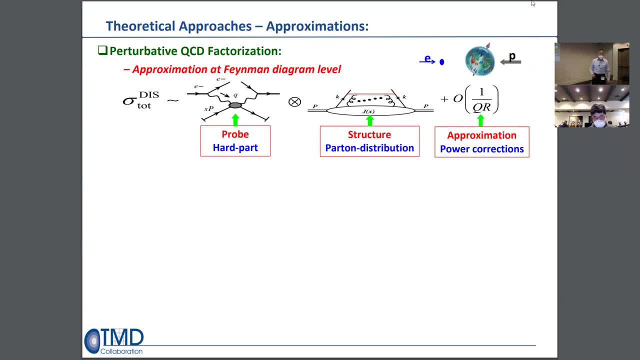 So this one approaches, make them approximation: The family diagram, That's what we spend most most of time Last 40 years. Then also the effective field, The approach, For example, Level Non-soft correct Solution in your factory and PCD or many other effective theory, our power provision theory, so you expand. 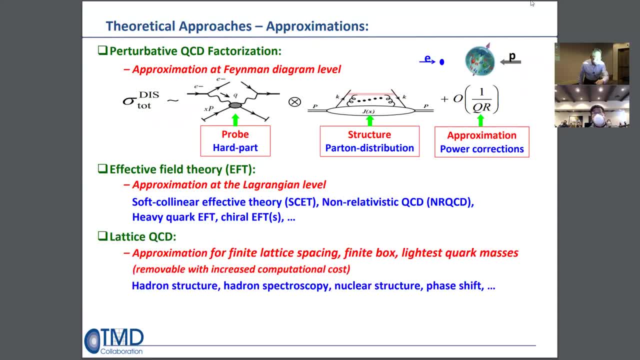 your theory at the level of Lagrangian, Then also that QCD, that QCD in the sense I make a proximational spacing instead of I have an infinite universe, I break it into the grid, then they some side, then I can calculate upon the computer. so the only remove, so this constraint, approximation, is the computing. 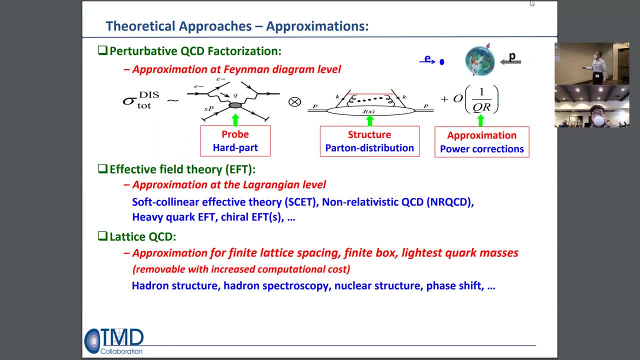 power. but this can be do the very sort of was principle, the sort of non perturbation calculation, Then also their model of the many, many other approaches. so this is a major approach to study QCD, all of them involved in perturbation. that's what I want to say. so now we will concentrate. 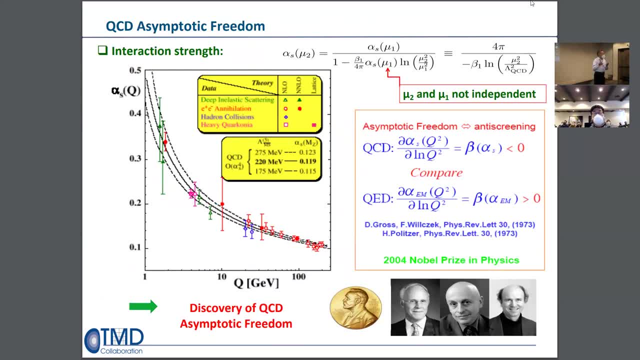 on the perturbative approach because we can control, we can calculate them, So that the reason behind it because asymptotic freedom, They discovered that The strength of interaction actually going down as a function of the momentum transfer, the number they can go to the 10 minus one. 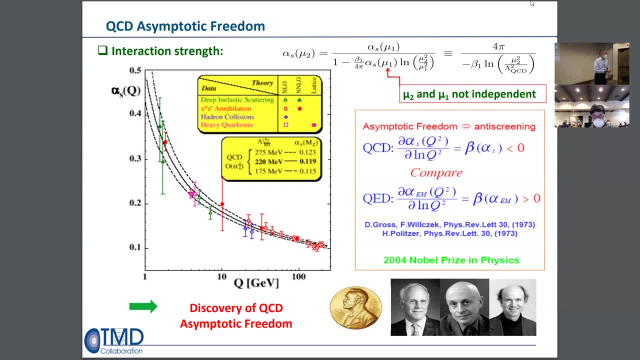 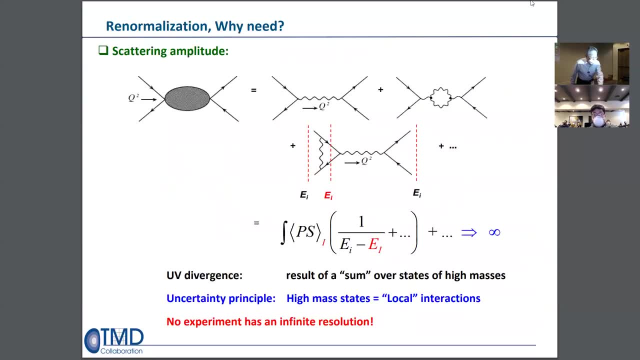 Although it's not the 10 minus two like 137 for the five structure constant, but at least this is sufficient small, we can do the perturbation theory. So now, while we do the perturbations- here is not a category diagram- you run their few- 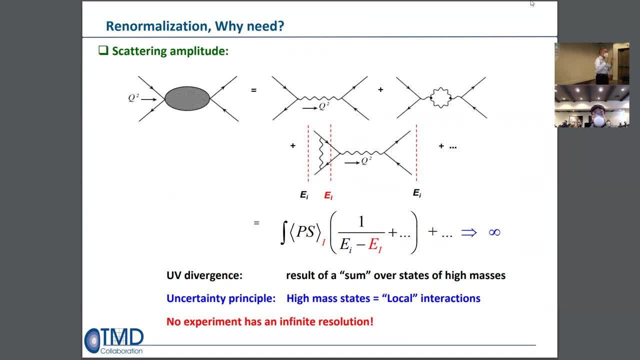 concept. I will use a few slides to summarize them. those are very, very important. concept Number one is the renomination. you heard about it. when we calculate diagram immediately find it. if we pass minus to Exchange a photon or grew up, then go to a plus, minus or the cork and tech work they. 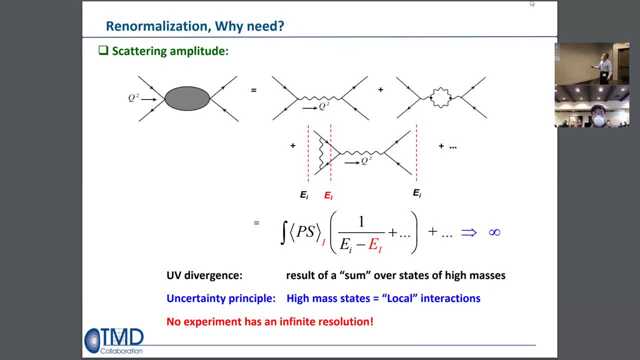 immediately realize you have this kind of loop diagram. You have this loop correction. now, if you need to go over this rubric at infinity, what's going on? I tried to do the perturbation. I end up with the infinity, Even though I claim my coupling constant small. 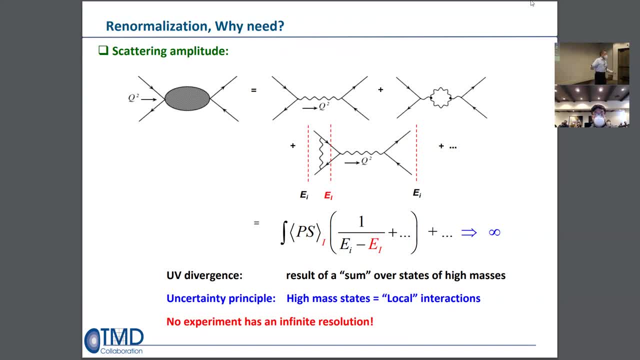 Plus The constant time, the infinity, forget it. I can do, cannot do the provision here so well, the idea of the exam where the infinity come from, The very comfortable we go over this phase. you have a high momentum state, there's any just date, so that means you some over the state of a high mass, large and very much well. 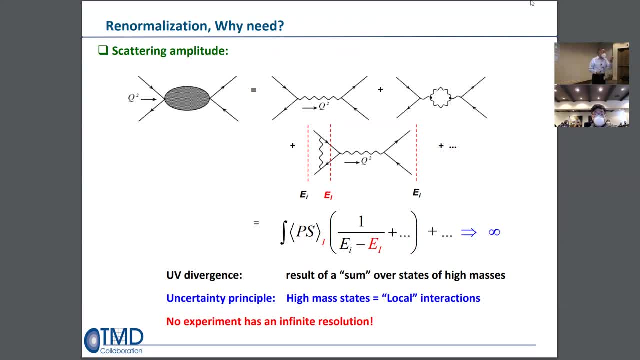 those contribution correspond to very, very local behavior of the theory. but we know any experiment you have more many transfer, You cannot see anything smaller distant than the wall of a moment in transport to never receive this state. So that led to the idea of the renomination, ideas that well, if this is local, I put them. 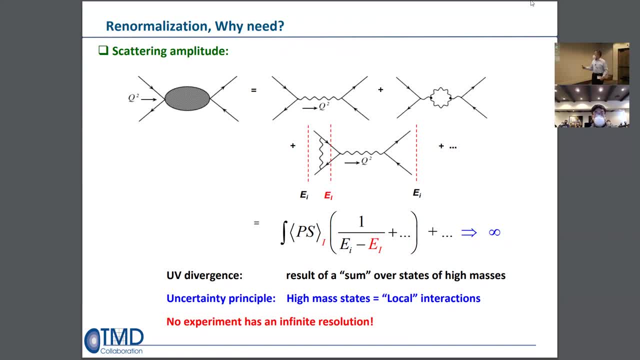 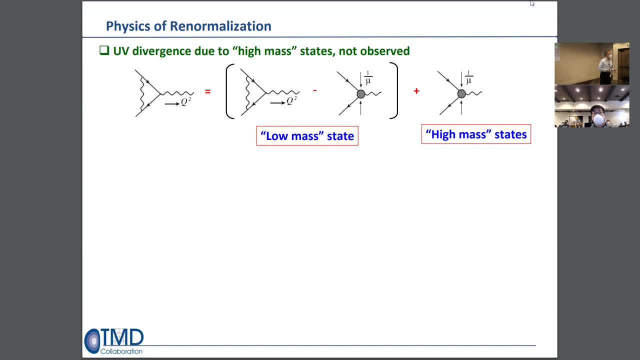 into the local, into effect local interactions. so I gave you example. So what the renomination do? renomination is effectively organization of your perturbed expansion. So this is a diagram, if I integrate the loop of divergence. so what do we do? i'm just subtracted. 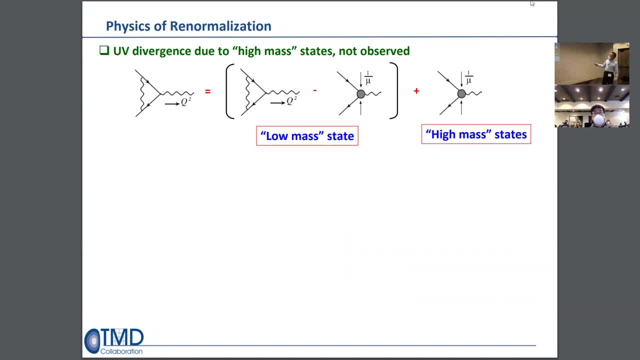 off the term local. so This is a high mass state, because the meal is some logic beyond what I can pull from experiment. so I add a subtract So that after subtracting that this part no longer have divergence when the momentum transfer between, because momentum is bounded by this value. 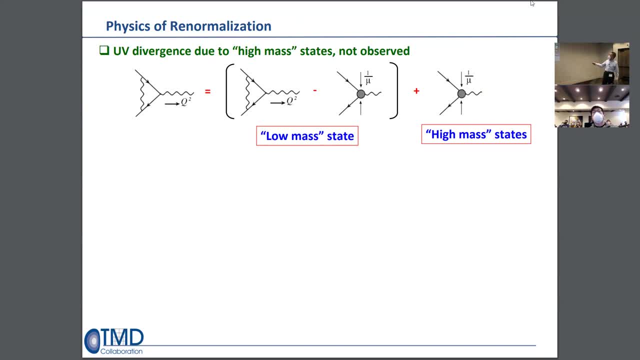 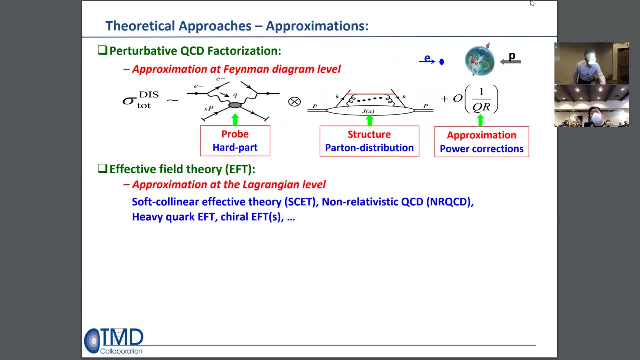 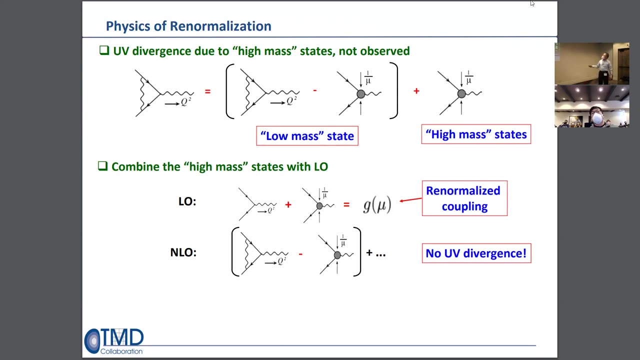 Now everything else sounds like a paternity divergent, but they're local. the point like: So now what we need to do for physical observable? ups For physical observable. you all know how to cackle from left hand side: yeah, famine diagram, leading order, next to the order, but next we know and divergence. 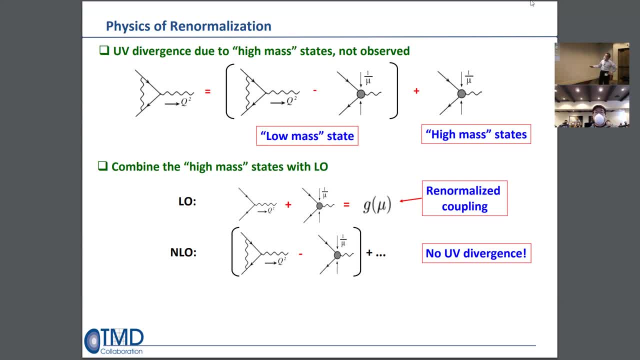 So what i'm going to do. I need to add the subtract subtract, a high mass state, here for next leading order, but I cannot shoot them away. it's a part of a theory. I include them into local Now then, in a sense, effect interaction now depend on skill. you probe them, so we combine. 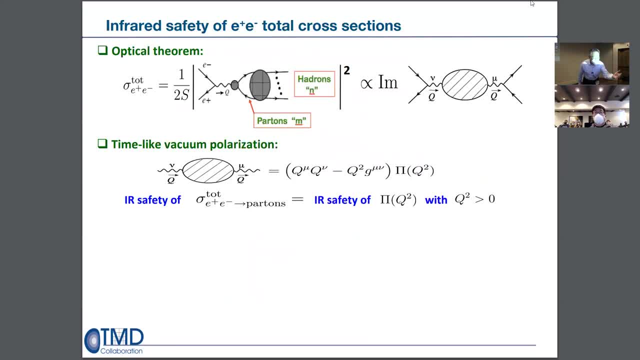 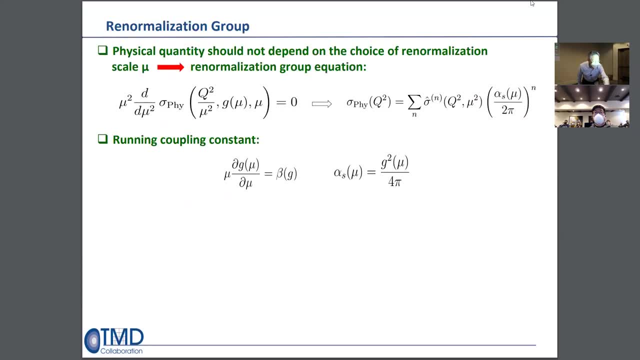 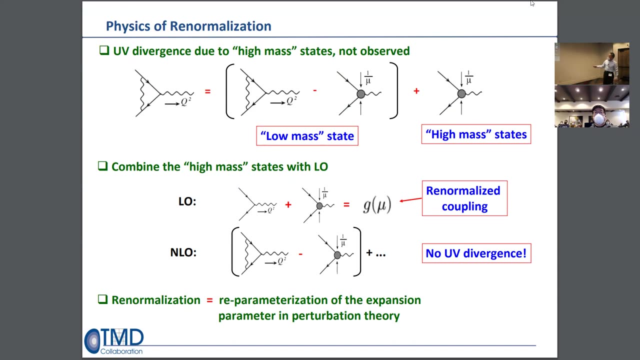 this together, So sensitive my hands is, just See something. I have some kind of magic here. So what happened? is that then? the new perturbed expansion is not expansion this way, rather, expansion this combination of the leading order, this fashion. next meeting order. 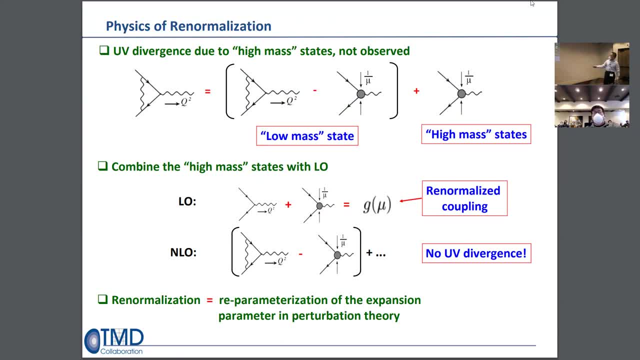 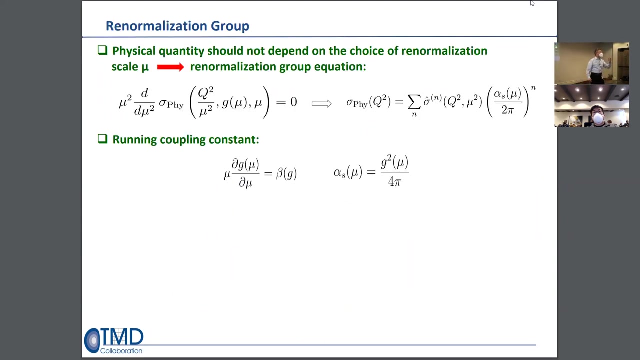 So it's a So, in this case the federation theory. So So. but physical quantity, you do the experiment. Experiment does not know how you expand it in the theory. So that physical quantity cross-section should not depend on whatever the scale introduced. 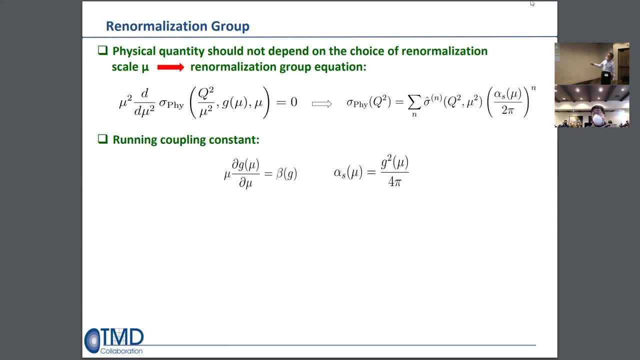 to separate your perturbation theory. So in that case then they have to be zero. So you lead to the physical quantity will be expanded in terms of the coupling constant where R fast, the immediate derived R fast, have to depend on scale your probe. 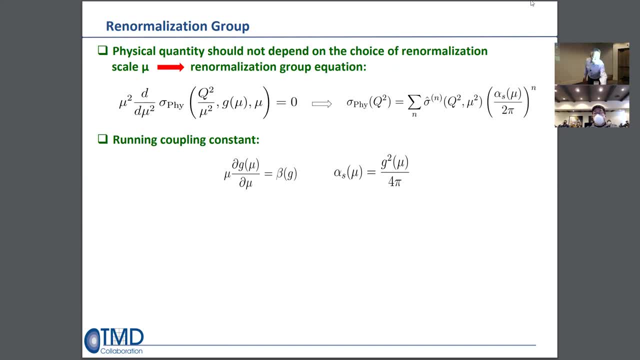 That's exactly the renomination group equation that tells you the strength of interaction depend on the scale of your probe. They can calculate this beta function perturbatively. you will immediately find that this beta function lead worth the Nobel price because it's different from the beta function of QED. 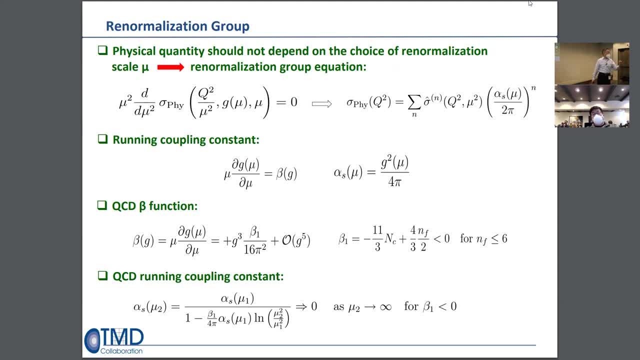 When the QED happen. we all know when you go to short and a short distance the interaction getting stronger and stronger. But in the QCD, because this beta function, you find it when you go to short and a short distance. 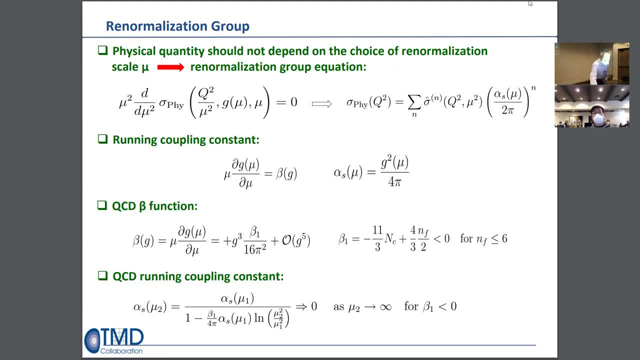 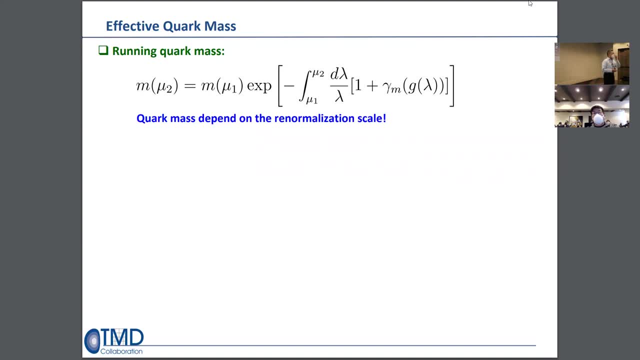 strong traction, getting weaker, weaker and weaker. So they also that. well, you just told me that a quantity you measure, like coupling constant or strength of interaction, depend on scale, your probe. What about quark mass? What about all the things? Well, in the quantum field theory, 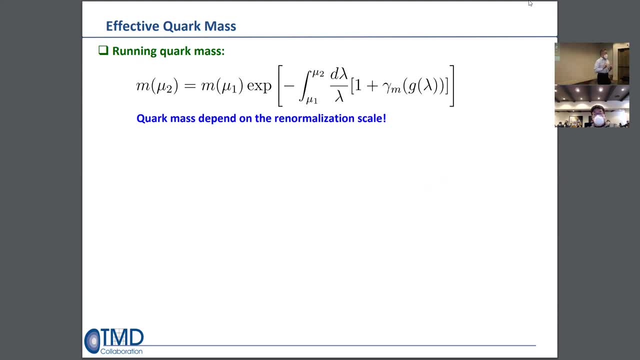 all this quantity depend on the scale, your probe. So if you the quark mass will also have. this is the relate, the renomination group equation. You find a dependent, anonymous dimension. You can calculate here. It tells you. But the bottom line is: 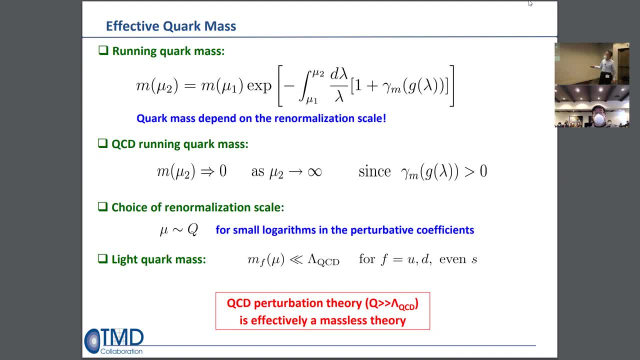 you will find that you can calculate that when the scale go to infinity, actual mass is asymptotically equal to zero. That means for light quark mass is much less than on the QCD. If you're dealing with a physical observable at the order of GV or the thing. 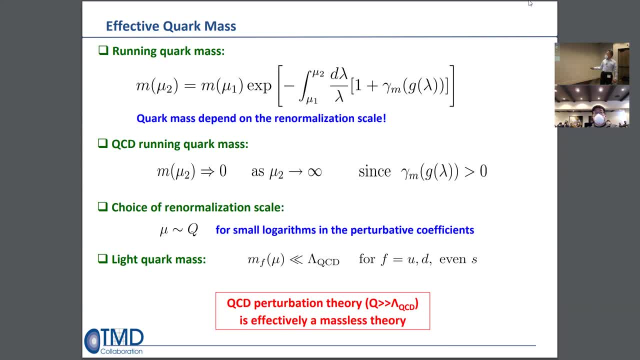 not to go to infinity, then you can treat a QCD. perturbation theory is effectively a massless theory for light quarks, So that's a message For when you're dealing with a QCD. if you're dealing with a light quark, 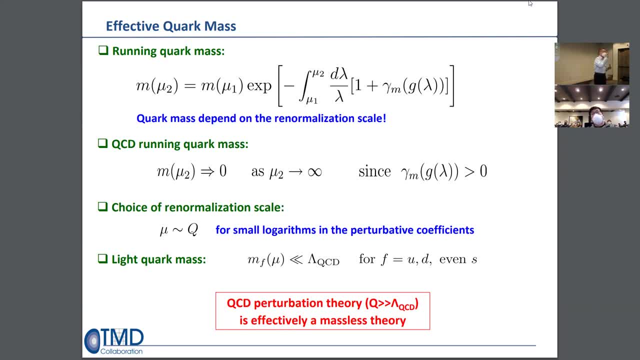 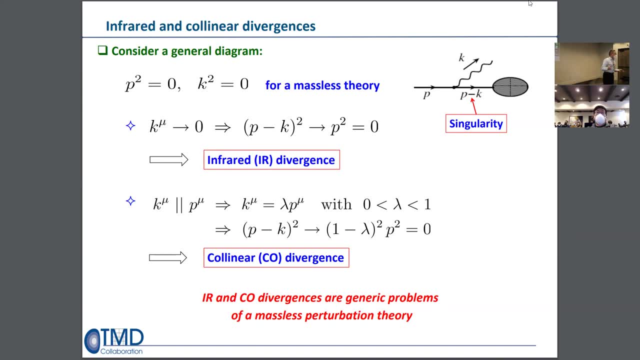 you can at a high energy experiment. you effectively treat light quark as massless. Well, if you do that, there is no free lunch. If you do something, something will come back to hurt you. So if you step to the, say, theory effect of the massless 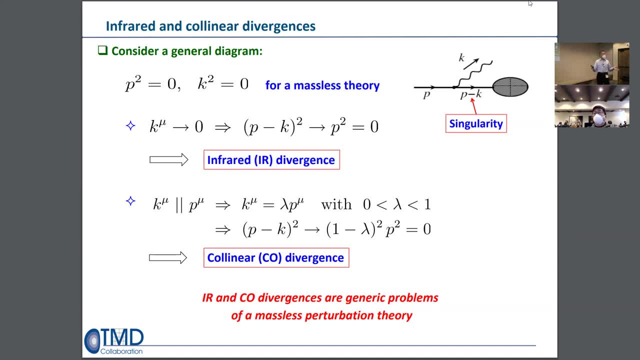 if you try to calculate diagram, you learn how to handle the ultraviolet divergence. Well, come with a massless theory. you have two more divergence you have to deal with. One is known as the infrared divergence, one is the collinear divergence. 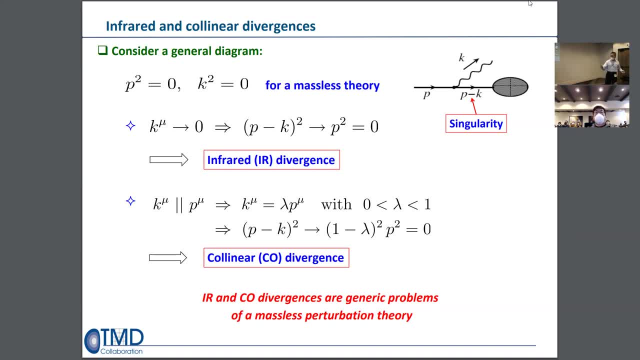 I give you a sink because you will hear a lot about this. It's really this week, So you take a simple example. I have a say quark interacting with something hot, but due to the hot interaction, or particle interact, you radiate, right? 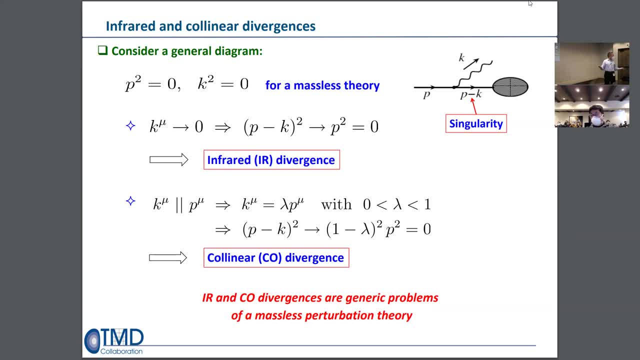 Radiate the ground, but you never observe the ground. You have to go over the ground. Then what happened to this propagator? You will find that if this particle you observed, they treat it as a massless P square, k square equal to zero. 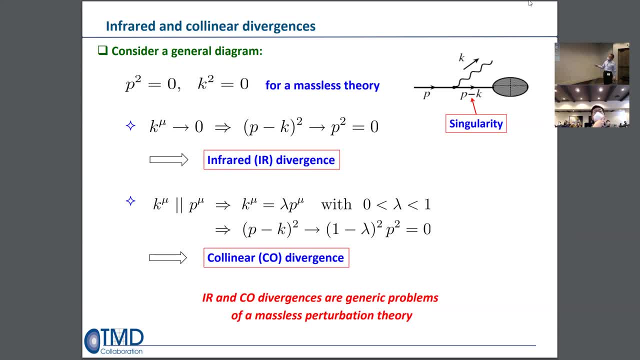 Then if you do look at this momentum, you will find that if you do look at this momentum, you will find that if you do look at this momentum of this propagator, you'll find a P minus k square. actual approach to the P square approaches zero. 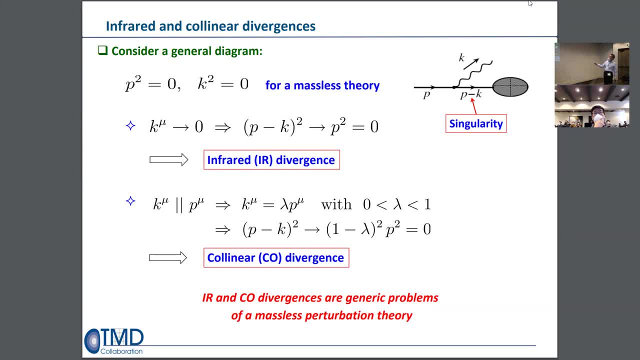 you'll lead to so-called infrared divergence. If you all, the component of the k goes to zero. If the radiation getting smaller and smaller, you get infinity. Something's wrong, Yeah, go ahead. What if the initial particle is not on the shell? 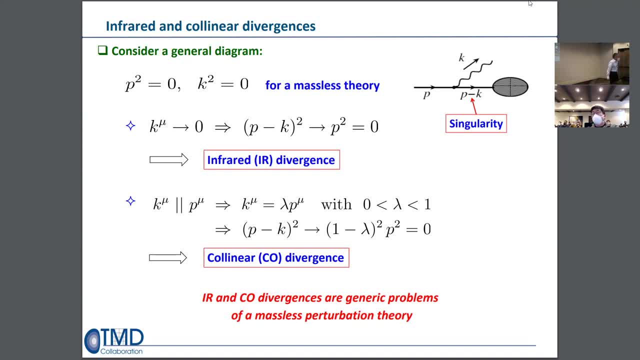 What if the initial particle is not on the shell? Are you saying, simply, the heat is virtual because the mass is small? I tell you, here we're dealing with the calculation asymptotically. It's treated the asymptotic state. We define the scalar amplitude. 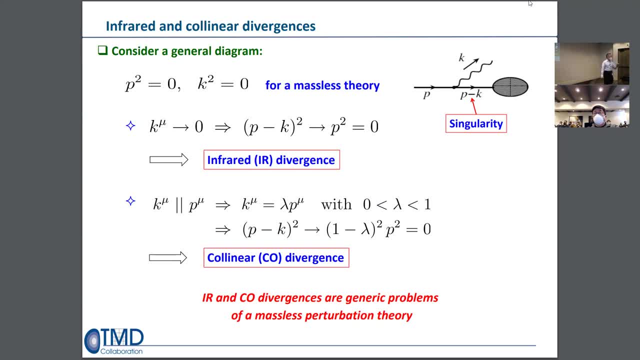 the on-shell particle. If you treat the off-shell I can tell you anyone interested. you have to be extremely careful, that number of the famous mistake by famous people. because they treat the part-time off-shell, especially Goulang, you break the gauge inverse. 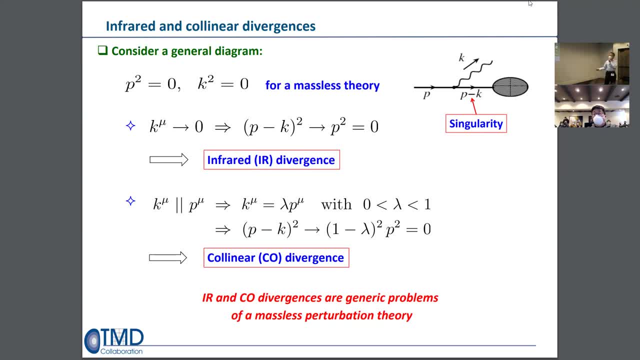 You have to be extremely careful. But anyway here, let's stop here. So this is the one possibility When the Goulang momentum go to zero sounds like a system, no radiation, but if you calculate you will find this contribution is a much bigger. 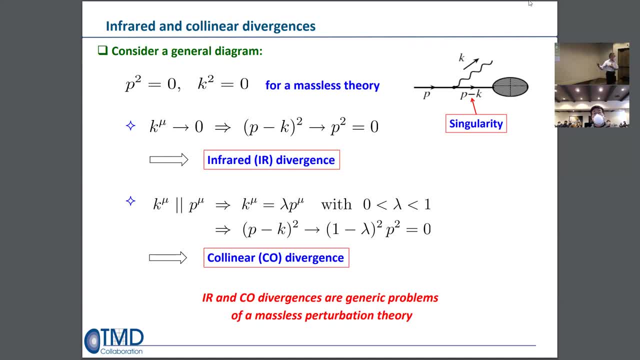 than one. you start with without radiation, because this is infinity, Just like the ultraviolet divergence right. You choose the lowest order, the finite, next leaving order, you calculate, you'll find an infinity. That's a problem. So this is a problem we have to deal with. 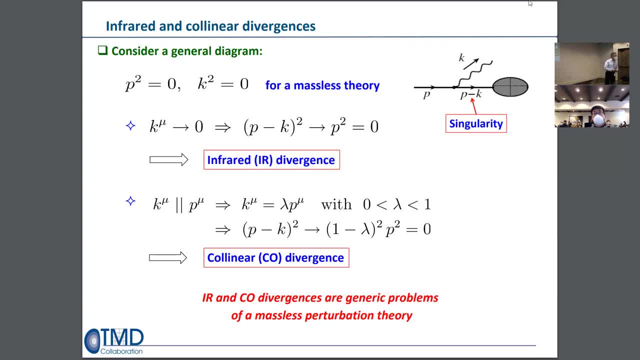 I'll tell you how to deal with it. Another problem for the mass list: a K does not have to be zero If the K is a parallel to P, so the Goulang is around this direction. even the Goulang momentum is not equal to zero. 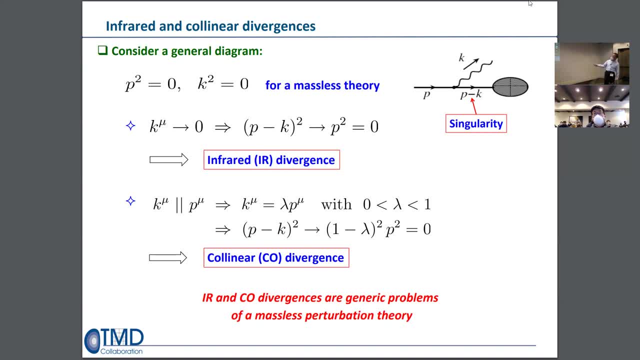 you'll realize that I take the K as the Lambda times the P. the Lambda is a constant. that P minus K squared is proportional to zero again, This divergence known as the collinear divergence, when the K is a parallel to the P. 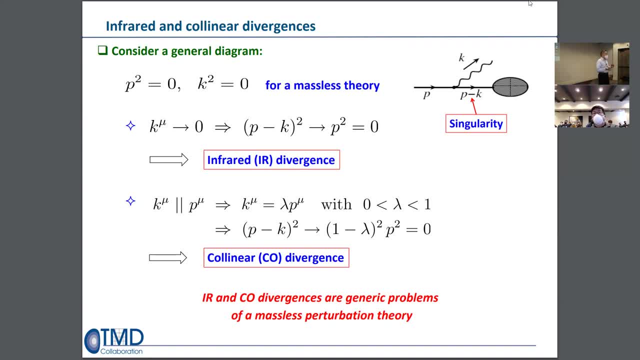 That's another problem we have to deal with. You'll hear a lot of factors: factorization. Factorization is exactly the origin of that. is that collinear divergence, The infrared divergence taken care by the theory itself, if you're including everything at any given order? 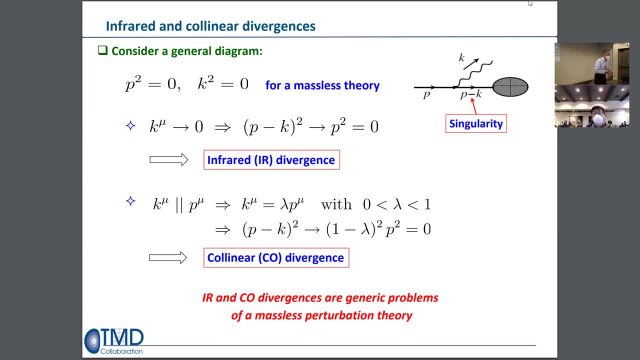 for physical below quantity. you can prove the infrared divergence, have the cancel among themselves, But collinear divergence. if you observe a particle, that means you know that momentum. So any radiation, the parallel to that give you collinear divergence. That's the one give you all the trouble. 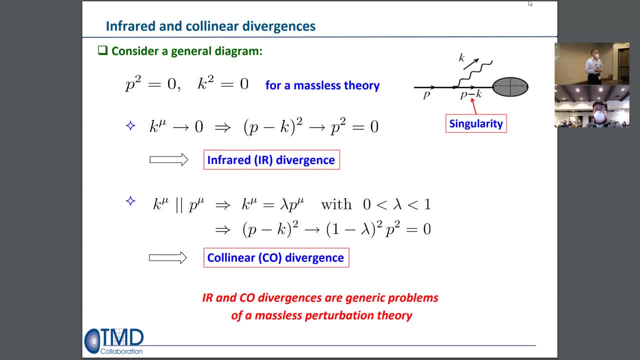 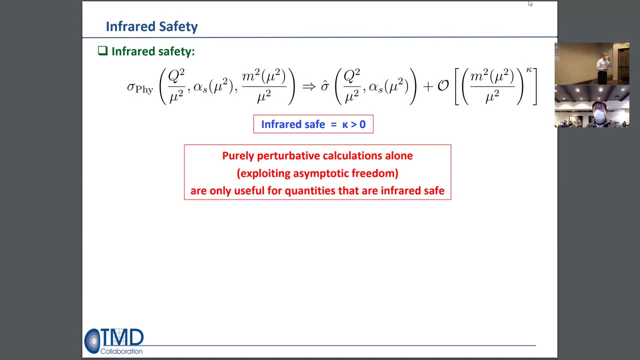 That's the one require the factorization. That's the exact essence you'll hear a lot about this week. So next one is what the PCD can actually calculate. special perturbed PCD. So the idea is that any physical cross-section. 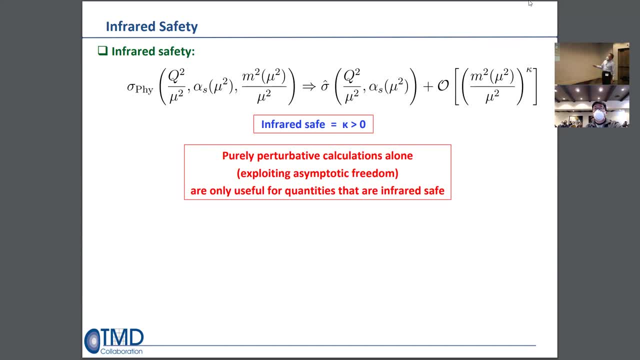 you have mass scale and a whole scale and factorization or denomination scale in this case. Now, if you do this expansion, say when the mass scale go to zero- because I say it's a, you know we can treat it as a massive theory- then the expansion. 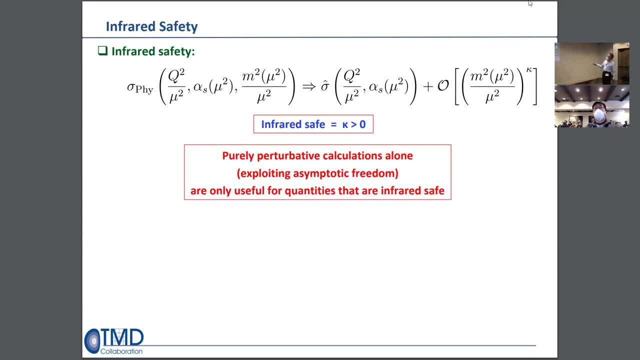 you can say: imagine, through the mass reading term, then the correction term and all the mass of these over the whole scale, where the parameters, This expansion, is only convergent or valid when the copper is positive. So we define the quantity known as infrared state. 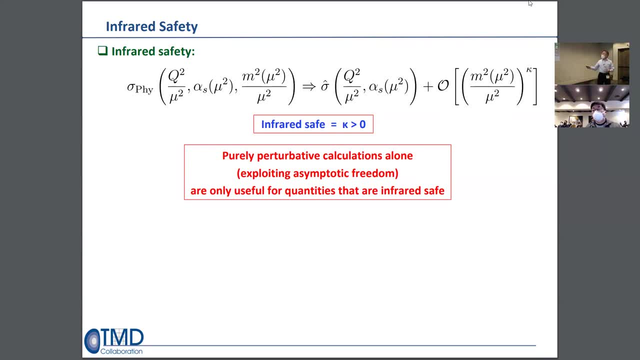 That means you can apply perturbation theory to calculate corresponding to this copper is positive. So the conclusion: that purely perturbation calculation alone, if we try to take advantage of asymptotic freedom- are only useful for quantities that are infrared safe. Now I will tell you a lot in my lectures. 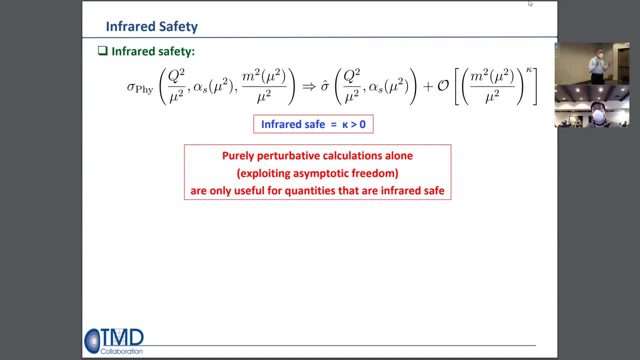 and you hear a lot in the whole week. a physical quantity with identifying hadron is not infrared safe. So how can you dealing with, let's say, deep enough, scale and cross-section hadron, hadron, cross-section, scattering cross-section people doing all the time? 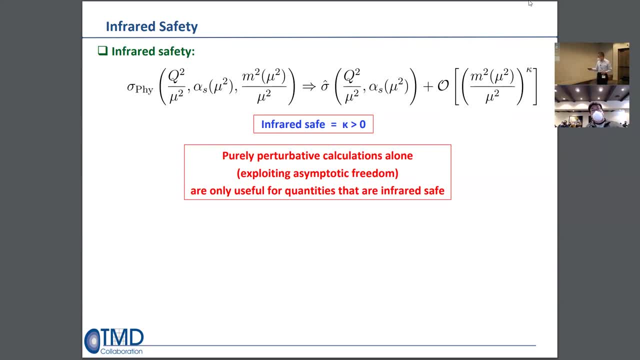 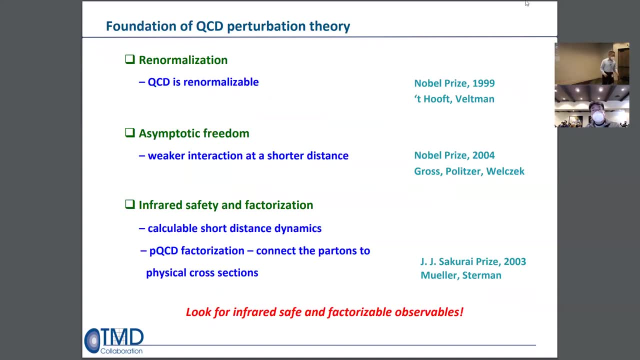 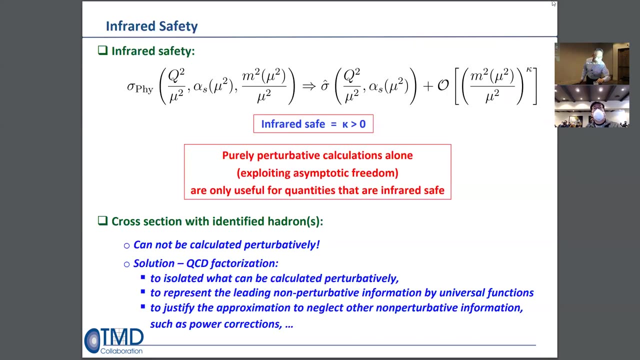 they are. you see, that's what you need to know, learn. So the solution to that, so that's a quantity, so that what I tried to summarize so far, solution to that: if you have identified hadron, they are not perturbative. calculable solution, the QCD. 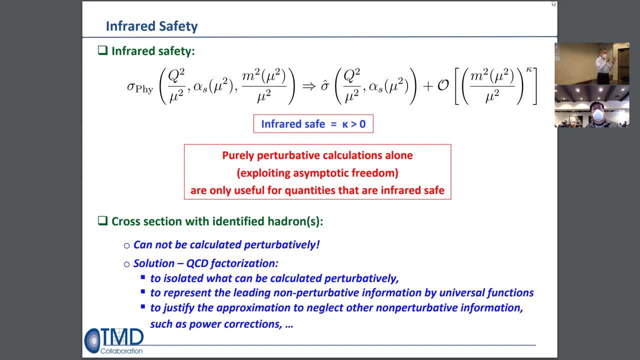 factorization. What are the QCD factorization? I said in words, I'm going to give you a very intuitive form example at the beginning of the next lectures: Words that you have different scale involving the collision. You have a hard momentum transfer, like Feynman did. 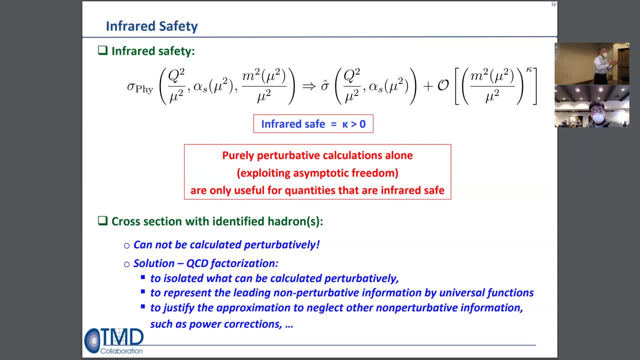 There is a scale of the hadron itself, order of Fermi. You have a momentum transfer, order of GeV. So the factorization is that I'm going to separate the physics between the different scale. Then you make you have to prove the quantum difference. 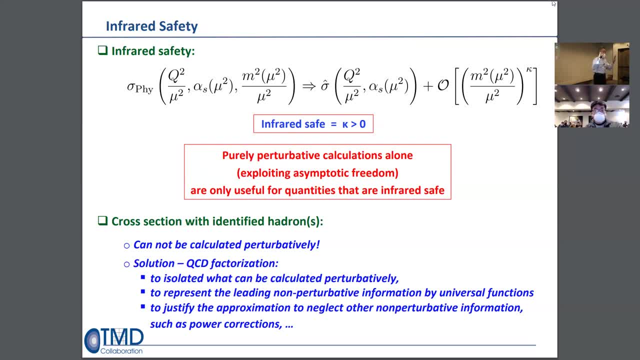 between these two scale is suppressed, So you can neglect them. Cross-section, the probability, your factorization factor right. one probability in turn, the product of two probability: One probability at happening at the short distance with large scale. Another probability is a happening at distance scale. 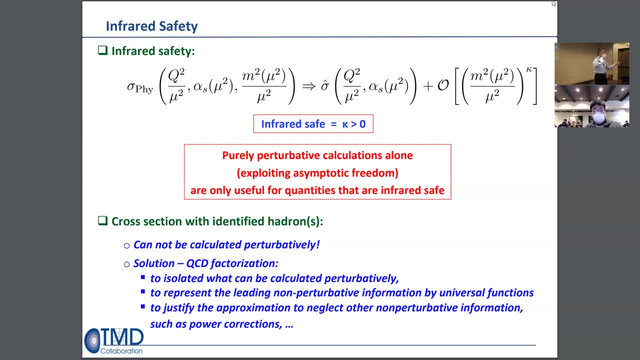 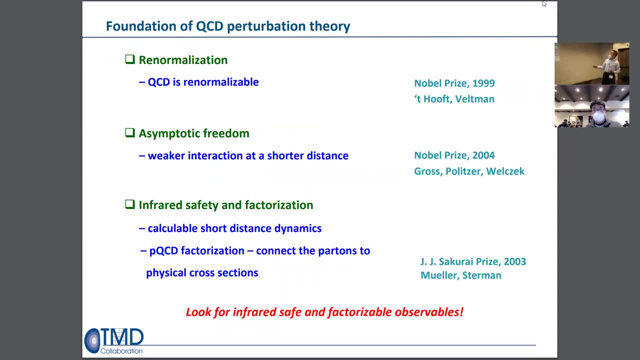 of the soft scale, non perturbative scale, The correction between them can be power suppressed. That's a statement I will prove to you. So then, summarize all the perturbative approach to these, There are three key fundamentals. One is that the renomination, as we said, 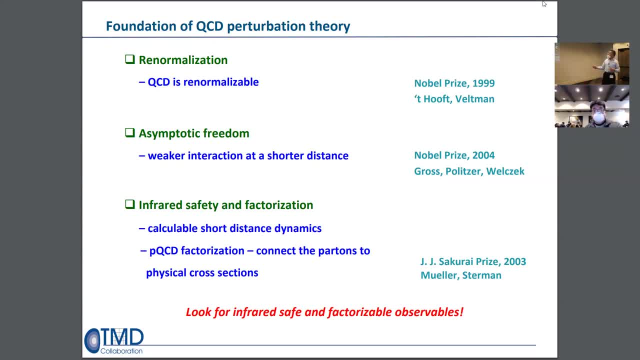 which led to Nobel Prize in the four-gauge theory. Then also asymptotic freedom, because you can go to short distance. strong traction can be effective, weak You can calculate. That led to Nobel Prize. That's very important. Third point: 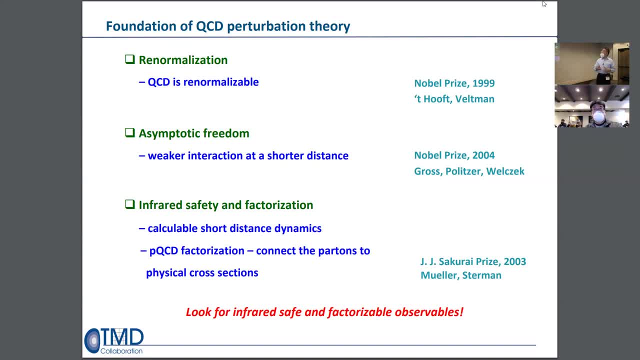 Part if you're dealing with identified hydron is known as the infrared safety and the factorization. The calculation will show distance and the factorization. They can connect the proton to physically observe the cross-section. They led to this APS, the highest theory prize. 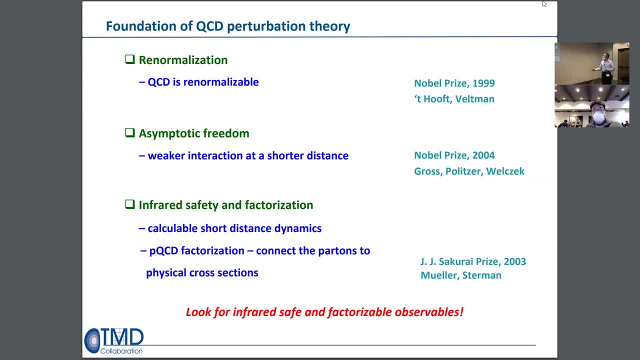 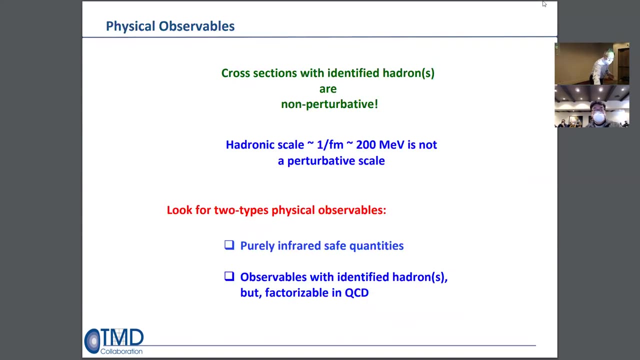 This is a Sakura Prize by Miller and Listerman, So what we try to do is look for infrared, safe and factorable quantities. So that's a first part of the really important introduction: how we end up with the QCD and how we could deal with it. 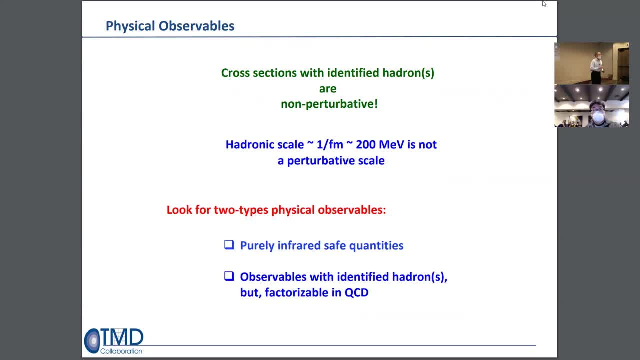 So now I'll give you an example before I finish this lecture. I'll start with example. don't identify your hydrons. I said earlier, if you have an identified hydron, you cannot calculate It's infrared divergent quantities. 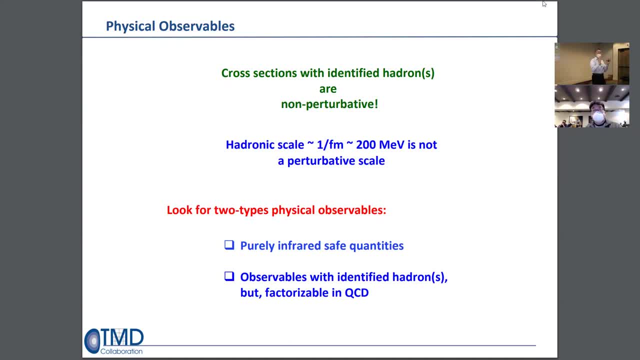 Well, what is the possible? There is observable involving hydron, but without the exact identified hydrons. Well, in that, because you don't identify hydrons, you can't calculate it. Well, in that, because you don't identify hydrons, you cannot calculate it. 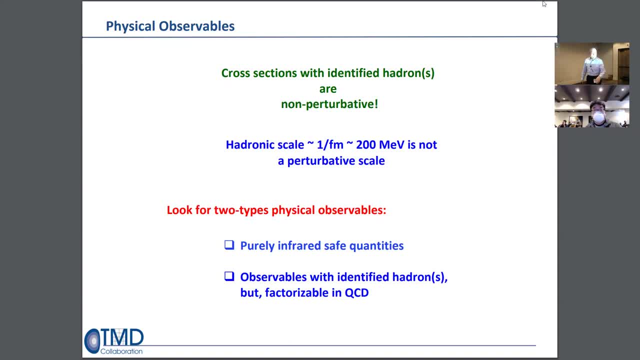 Well, in that, because you don't identify hydrons, you can't calculate it. So if I identify them, unitary help you. So I start with observable cross-section, with a look for two types of physical observables. One is look for pure infrared safe quantities. 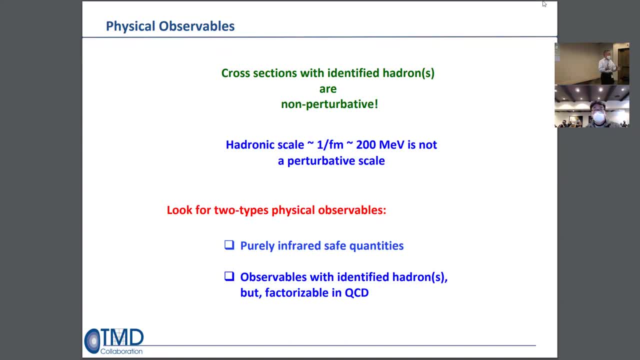 That means I can apply perturbation theory right away from beginning Another type of observable, the way to identify a hydron. that means I have to find the factorization. I have to prove the factorization to separate the physics at different scale. 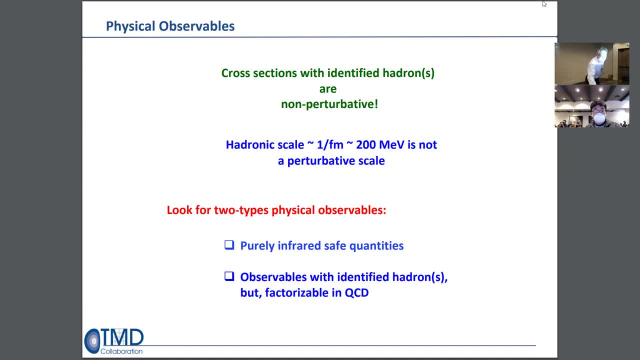 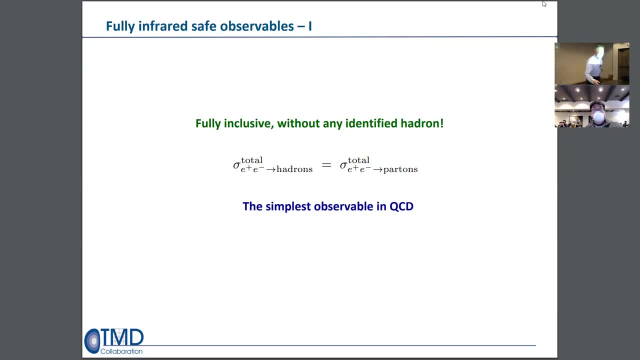 So this is the whole bottom line of our approach. It lasted really 40 years efforts. so start with something simple in this end up rest of my lectures. here you look for this. The observable, the fully inclusive, without any identified hadron, is known as E plus minus. 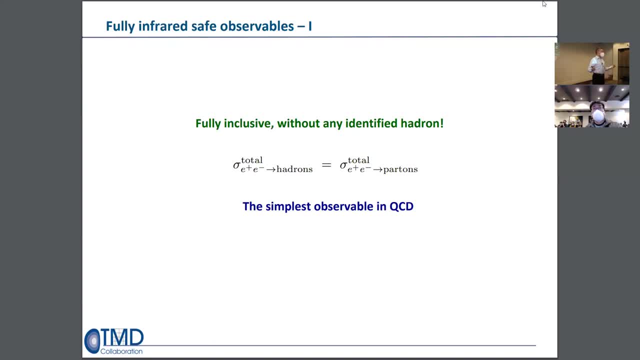 two hadron total cross section. That means you have a you know lap. did that best read now the running in the Beijing E plus minus client. look for the all the particle in the final state you without specifically tag any one of them. then the lap of the number of years ago. they did not have much higher. 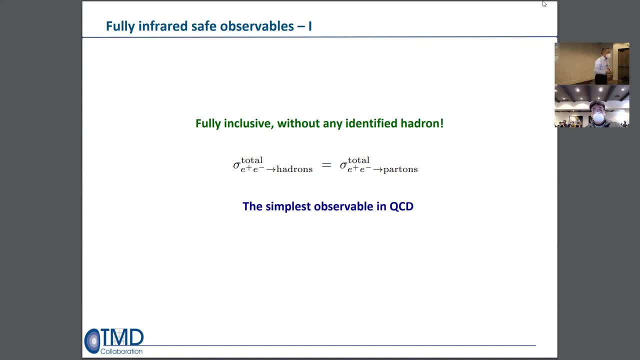 energy and also now in Japan, the bell to. they do expand with the plus minus at the end of the beam as well. What the best in the Beijing, the energy of the charm as well. so those are the E plus minus process, but you can produce had during the final state. 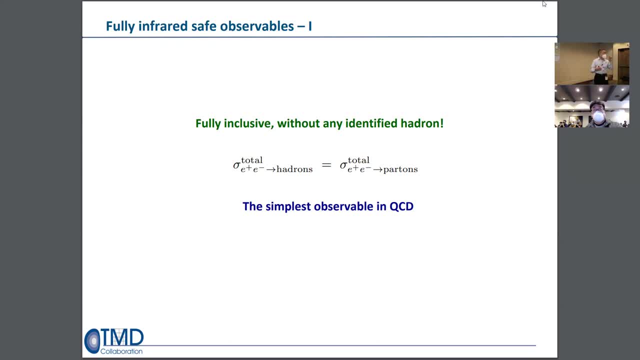 So what I define observables. i'm not going to tag any specific pattern, but I just integral for all All the possible- had, whatever event you find it have, one had joined it- okay, that's part of my event- and a two and three. I include all of them. 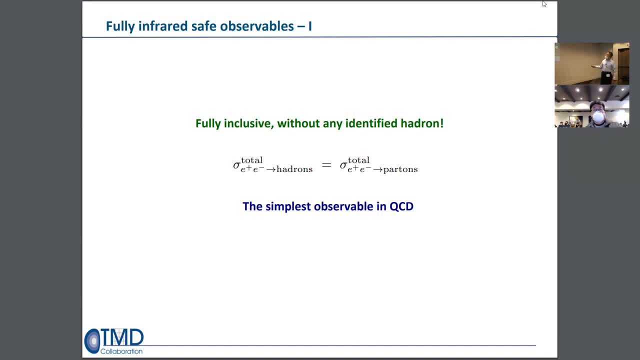 In that case I can show you the cross section to E plus my total hadron is same as total cross that he passed, minus two patterns or corpse belongs. because you eventually prove this quantity, you can capture increasing probation theory. I start with a simple, intuitive argument. 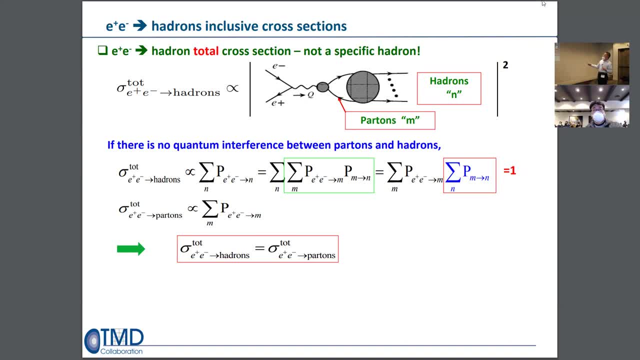 I have a scary up with you: E plus minus exchange of photon. you know cause my virtual photo or Z have some kind of short distance hawk collision controlled by the momentum transfer queue. Then they produce a bunch of a particle that have a state at a label of the end of a platonic 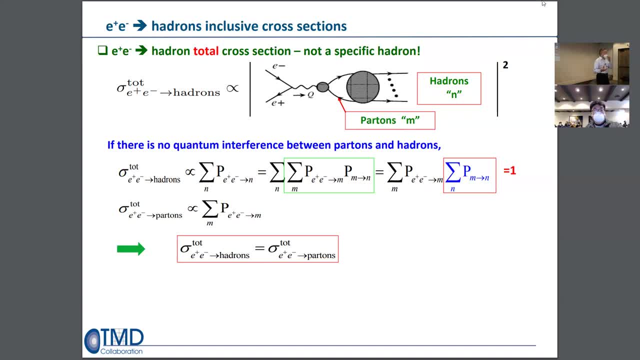 state but confinement, it tells you, never can have a pattern enter in your detector. The partner have to, eventually emerging to hydra. so at an empathy level there is a broad. they go and have had your detector. I call stay in. So in terms of cross section, the probability I can imagine, the cross section proportion. 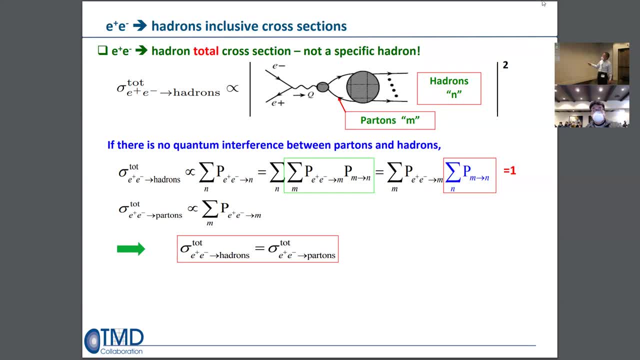 some of the probability plus minus to the, the older hadron. I can write them into the two step: the sum of the end in the middle part the probability is equal to the product of E plus minus to all the intermediate partners. that and then 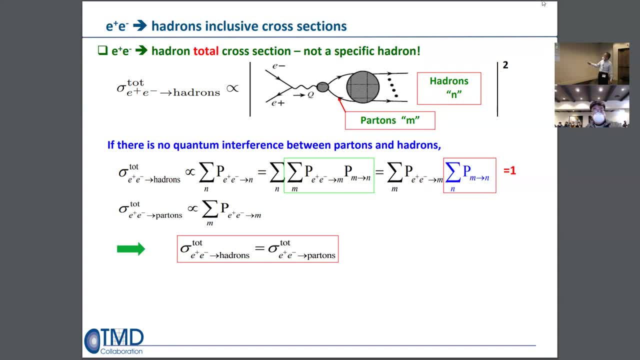 multiply the probability and goes to am, and So then I switch to the order of integration. Let me say: Whatever have stayed am, with a part of the have to become the hydron. So I write in some of the aim, the probability plus minus the part time. there's some of the 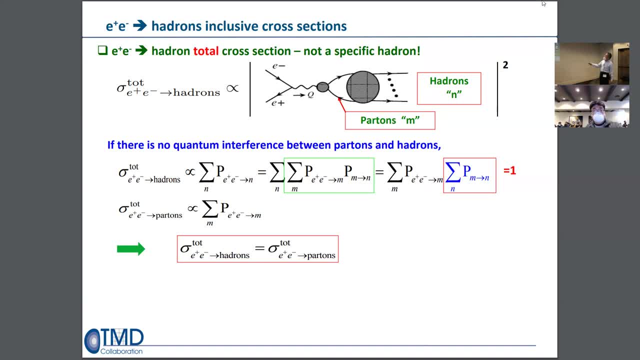 older. probability for m goes to the end. You know this had to be equal to one, This guy. because confinement, you never see a free call to the grower in your detector. If we produce a cork, You produce a grower. They cannot go anywhere but become the hydron in your detector. 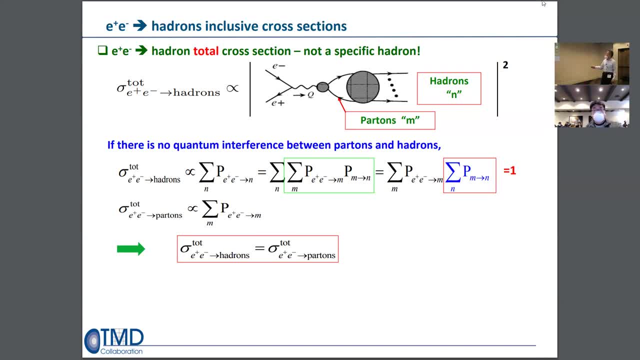 So if you take this as a one, you realize this is a probability. plus minus. hadron is proportional, the total probability to all the public state. So in that case the cross section to produce all the hydron is equivalent to the cross section to produce all the part time. 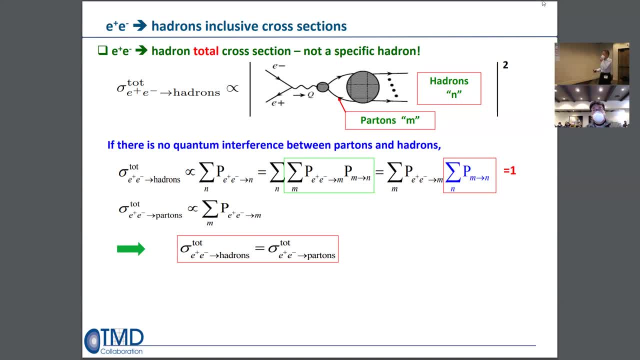 That's a very intuitive argument. I can give you a number of approval more rigorous. So then, with that, I didn't identify any hydron. you start with a cross segment hydron. You end up on the character, something to the pattern. 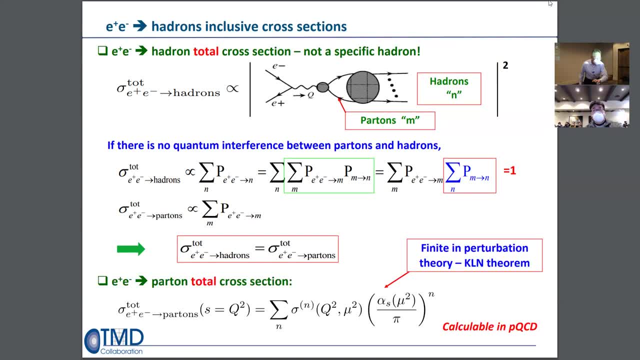 I don't ask any hydra Well. so the total cross-section to the proton in a QCD perturbation theory can be expanded as a power series of alpha S and a power series of alpha S with the larger momentum denomination scale of mu. 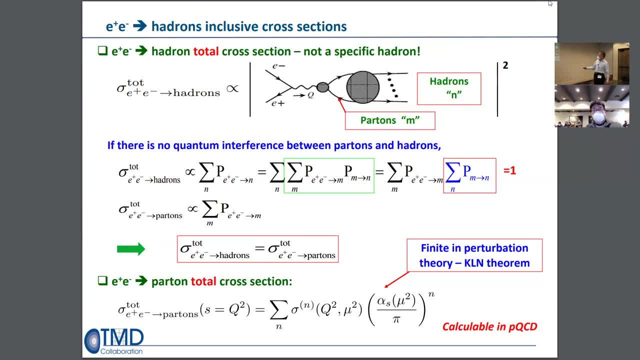 Mu is the order of a cube, that's only the larger scale sum over all the orders. So this quantity is completely perturbatively calculable in QCD perturbation theory If the cube is so much larger than this, whatever number of the scale. 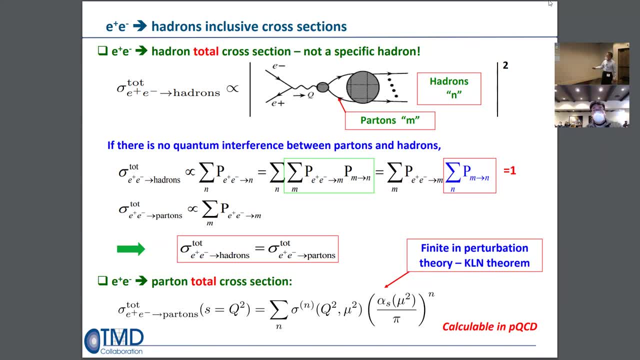 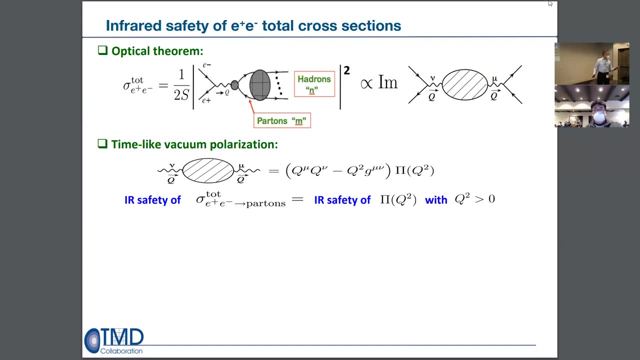 you will find that this is the quantity, the coefficient you can calculate. it's a completely finite to all order in QCD perturbation theory. People have calculated too many loops for this, So let me give you another, better proof. So well, I take advantage of optical theory. 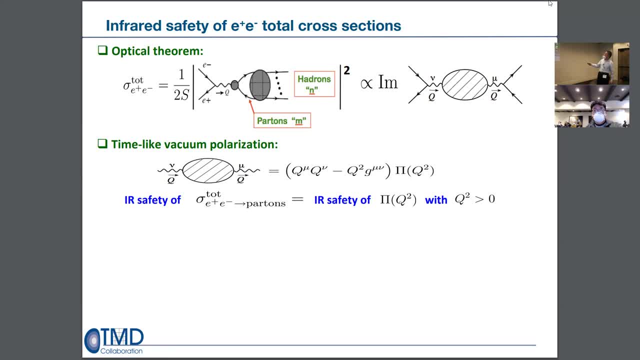 What you really have. E plus minus two, hydra, intermediate state M, Whatever it is. if the optical theorem is true, this is just the imagine proportion. imagine a part of force getting up to E plus minus two. E plus minus When all the interaction in the QCD. 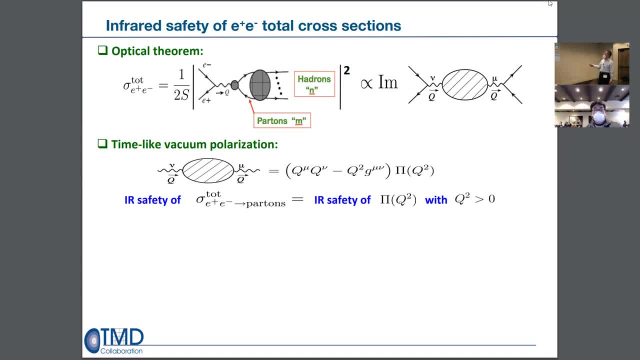 well, that's a broad, it's a time-like vacuum polarization. So then, from a current conservation, QED, current conservation. you have all the equally, equally weak. in triangle Z, you will have a Q, that's current conservation factor. you have, multiply the constant factor, a scalar factor. 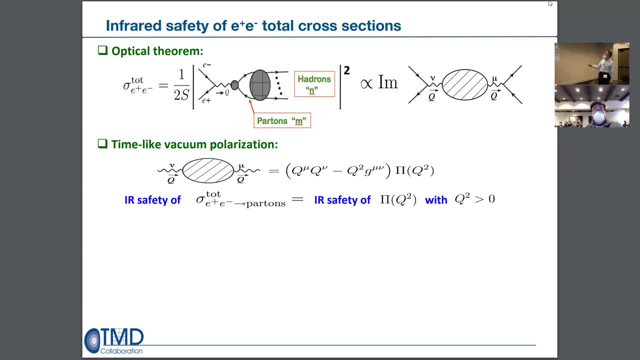 So then the question if this whole thing can be calculated. perturbation theory: it's infrasave. I mean the sigma. this, almost a big pie- has to be infrasave, Although there are lots of hydra in it. Well, how can we prove this is infrasave? 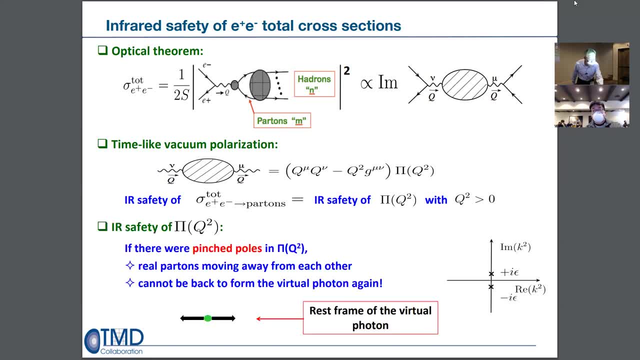 This, actually, you can think. I'll give you a very intuitive model. What's the infrasafety? Infrasafety of this big pie, in the sense there was no pinched pole in the pie. So you have physical quantities, you have divergence. 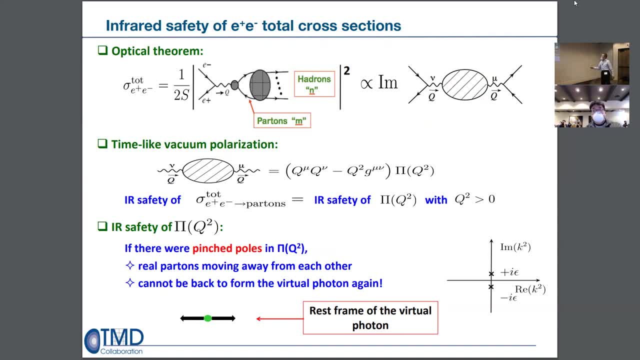 What the pinched pole means. imagine you have a phase space of any part-time in this phase, in this loop. inside it as momentum K. you have a K square is a virtual part-time. momentum is all over the virtual. you never see them real. 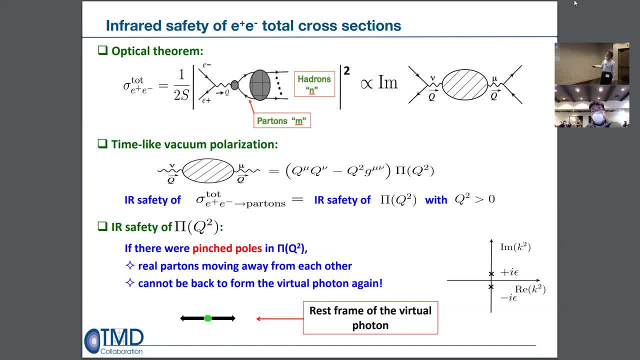 So imagine you integral the phase space. you end up with, say, there is a pole, you have the upper half plane, lower half plane. that means no matter how you deform, contour, you end up with infinity. So that's bad. 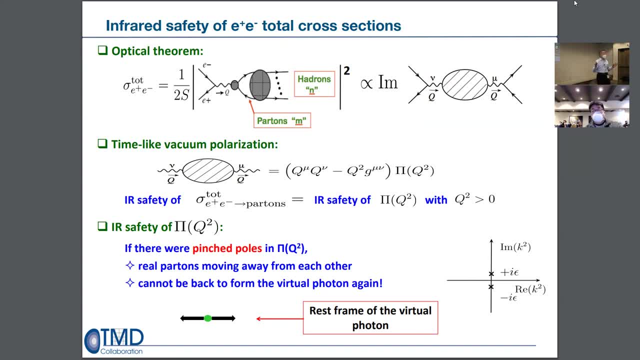 If you happen that way, that means that quantity can not be calculated in the QCD. So that's bad. If you happen that way, that means that quantity can not be calculated in the QCD. So that's bad. If you happen that way, that means that quantity can not be calculated in the QCD. 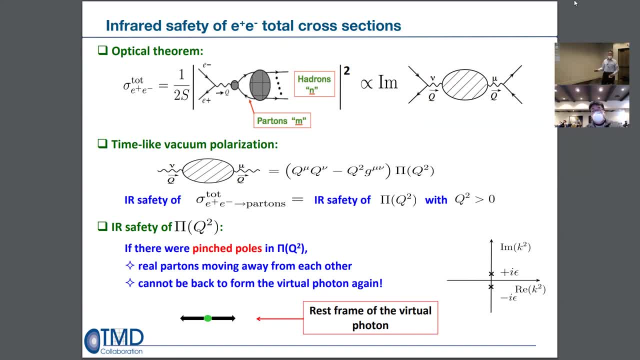 So you try to avoid the pinched singularities. Well, I tried to give a very intuitive argument. There is no pinched singularity. You cannot have pinched singularity inside this block, no matter how complicated. What's the pinched singularity? 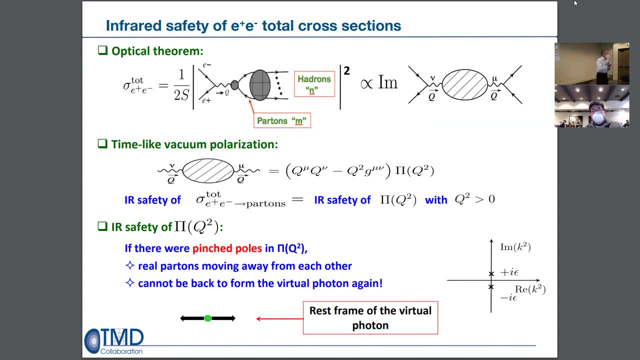 Pinched singularity when the K square go to zero means the part-time, like a classic unmasked shown flying away Because that's time-like. you stay in the standard mass frame of that virtual photon. you stay in the standard mass frame of that virtual photon. 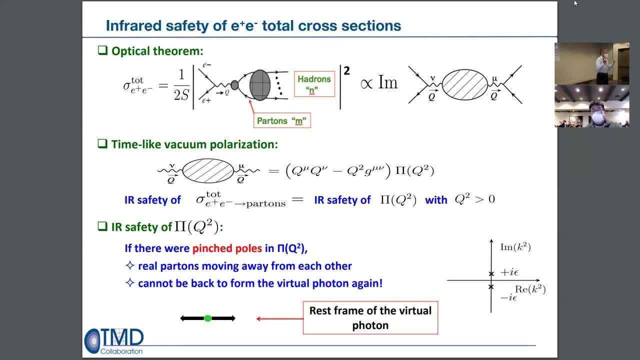 you stay in the standard mass frame of that virtual photon, you have an invariant mass Q. If you have two particles they pinch because momentum conservation have to back-to-back right. They have to fly away If they're pinched like a real particle. 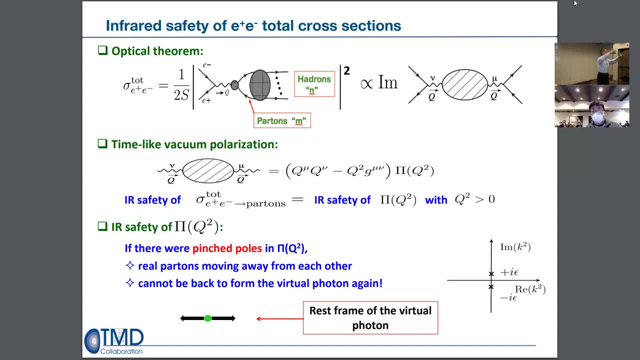 they fly away, what's the chance for them to come back and meet together? Because this vacuum polarization means two particles in, then two particles out, So you have to merge back. If they're really pinched, there's no chance for them to come back to merge together. 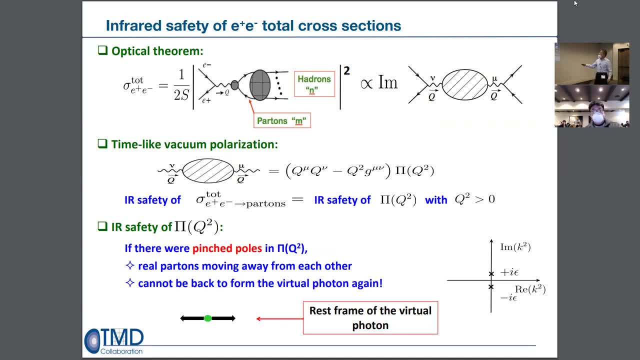 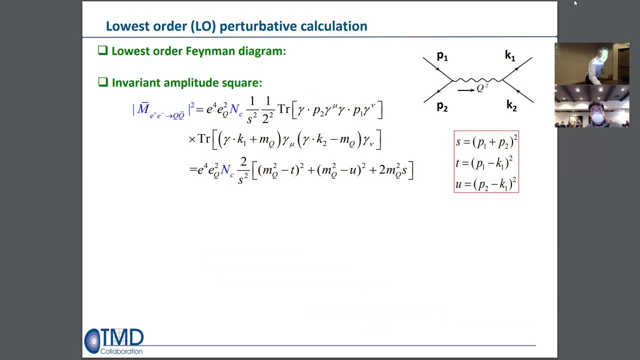 So that's exactly. intuitive picture tells you this block cannot have pinched singularity. I'm going to give you an example: how to show that. I'll start with the lowest order diagram. I have every single step. Say I have E plus minus two photon. 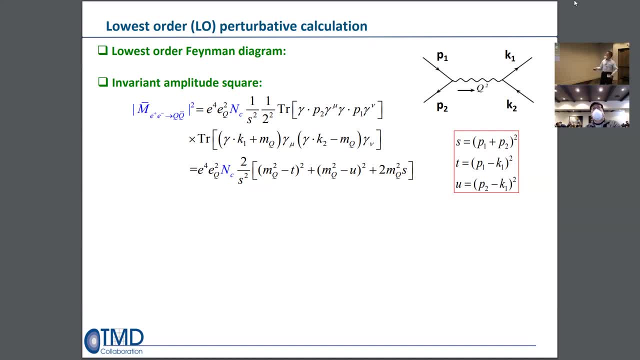 go to E plus, minus or any fermion pair. So you have a trace of this part square of the amplitude and the trace of this part of the square I put, even have a mass of a quark. Imagine this is a quark. 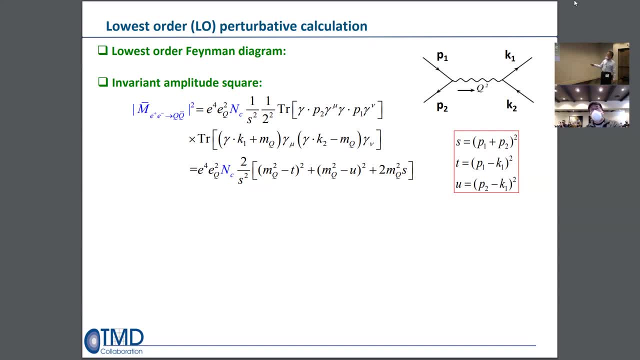 Then I worked about algebra, end up with this matrix, fermion square, depending on mass. Then we're going to calculate cross-section. So when I calculate cross-section- as you know, invariant mass, into the d sigma dt, then they have a proportional to mass square. 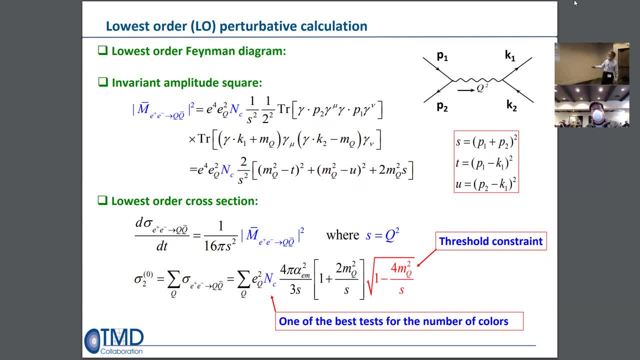 I worked out at this level as to put the sigma. two means out of a square, E, square the coupling constant, square your sum of all the flavor possible to quark, then you end up with a constant factor. then multiply a phase, the threshold constraint. 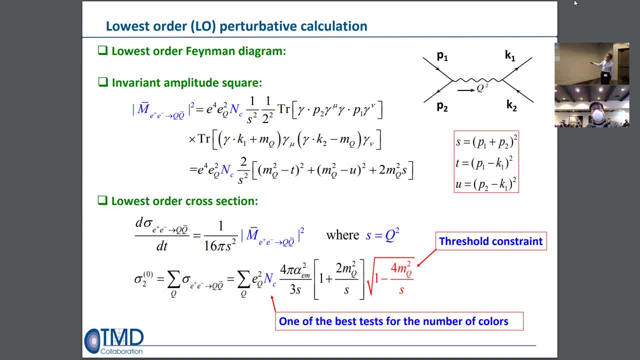 So imagine if this heavy quark, if you do this, total energy you gain is not enough for you to produce heavy quark pair, then they cannot be contributed, right? So then? so that's a threshold constraint Where this lowest order calculation is a complete 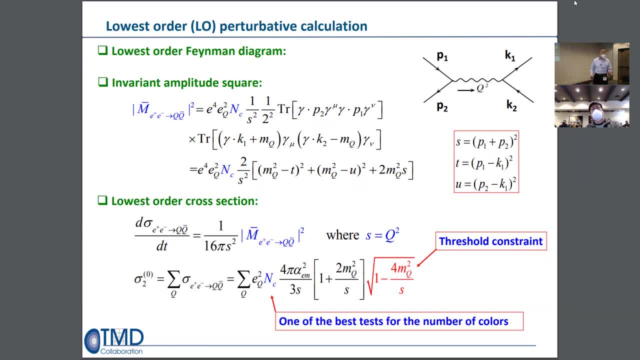 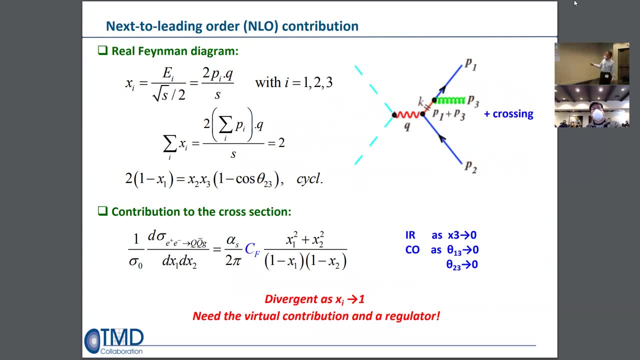 finite, no divergence. What happened? one loop. If you do that, we say, well, I'm going to radiate a group. If I radiate a group, then you notice immediately, as we discussed, if the particle, the mass list, 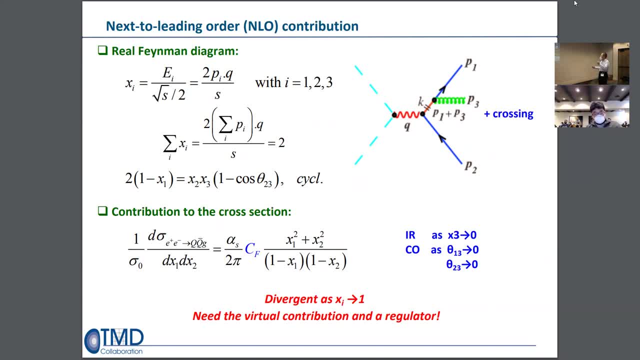 you will have infrared divergent and the collinear divergence How they show up. I put it in a different form. I introduce the energy fraction. XI is the energy of the particle you observe, divided, maximum: the half of it and the half of it. 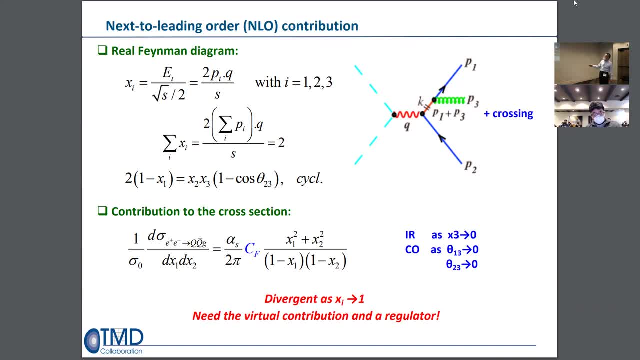 Now you will find out that X, if you have this relation in terms of the angle, the one minus X1,, for example, the proportion of the one minus cosine angle, So immediately you realize situation, you can have a divergence, this amplitude. 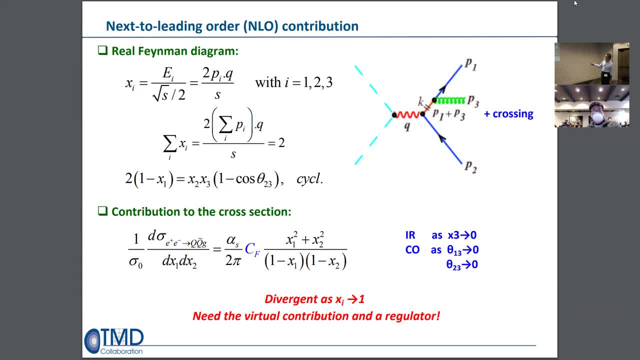 can have an infrared divergence when X3 go to zero, this momentum go to zero, as we discussed, And also they can go to collinear divergence. with this angle go to zero, The radiation can come from this side, you can, when this angle go to zero. 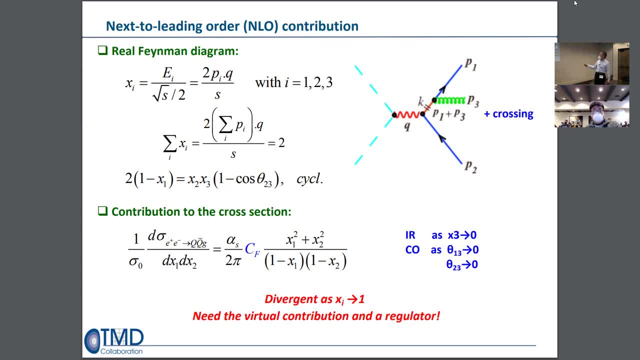 you can have a divergence. So this is at this order. if you only calculate this diagram, square plus the crossing, you get a divergence. Well, that's bad. Well, that's not the only diagram contribute to this total cross-section. 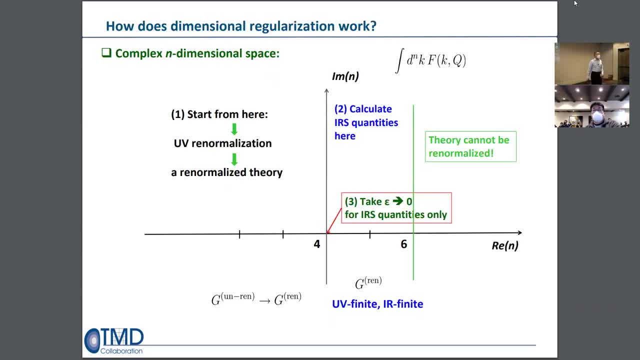 You have to include the virtual diagram. When you include a virtual diagram you know infinity minus infinity it's difficult to deal with. You have to have a regularization. You have to hold the infinity, not to go to infinity. Then you calculate everything, then you complete it. 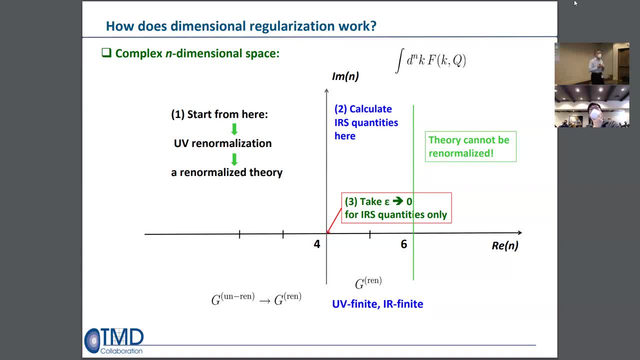 You combine them. So one very important regularization- you will learn a lot, hear a lot- is dimensional regularization. Dimensional regularization is powerful because that they used to prove the renunciability of the gauge theory to hold the development receiving Nobel Prize. But that dimensional regularization in the space-time, 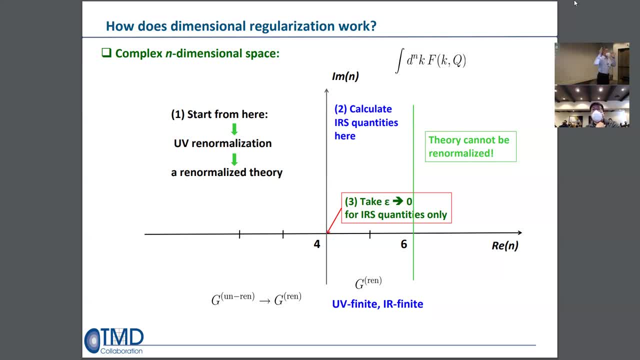 instead full dimension. I'm putting to any dimension a fractional dimension. After I do the calculation, I take the limit, the space dimension go back to four dimensions, But it's not arbitrary. You can try to regularize both ultraviolet and the infrared. 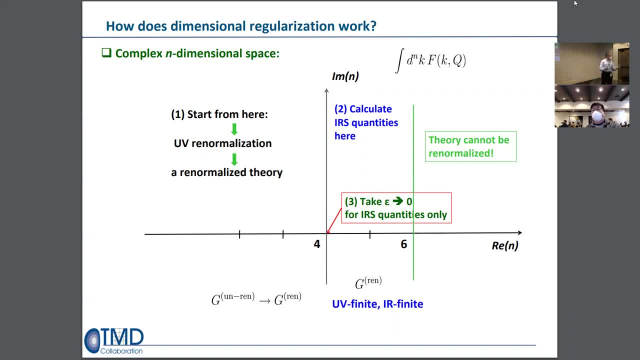 It's powerful. You can regularize both, but it's not the arbitrary way, So there's a particularly good way to do it. This is a slide I want to show. make sure we understand how the dimension regulation work For observable. so remember. 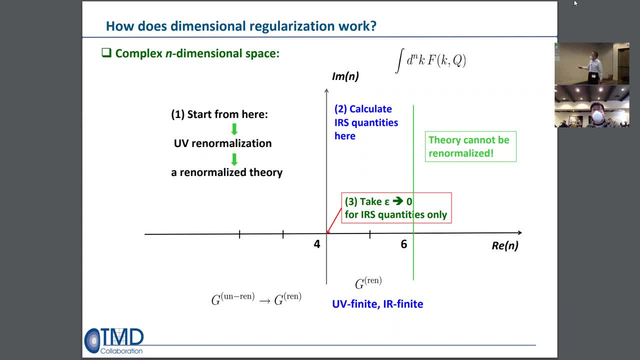 we first have to start from here in the region when the dimension less than four. So we do the UV renormalization. Remember we talk UV the first one, first to deal with it. So you have this: make sure your dimension go to small than four. 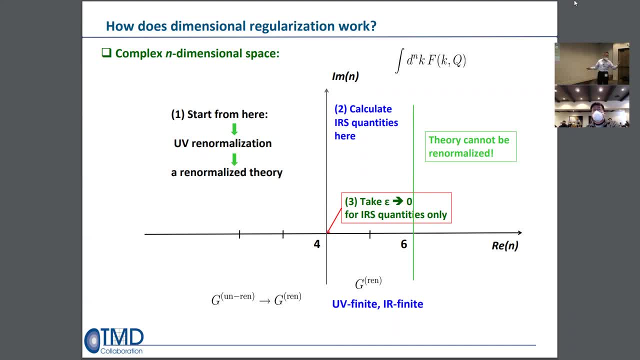 You have unrenormalized Green's function or any observable you try to calculate that lead to the renormalized quantity. But, as I said, I didn't change the theory, I just reorganized my perturbation expansion. So after I expand everything in the renormalized quantity, 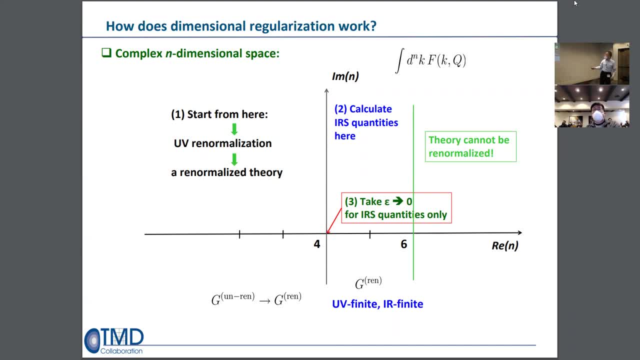 I'm going to analyze it. If I let it continually by dimension, go to the dimension larger than four, then this case only for physical infrared safe quantities. So I calculate this. maybe I have a real diagram of divergence. virtual diagram of divergence. 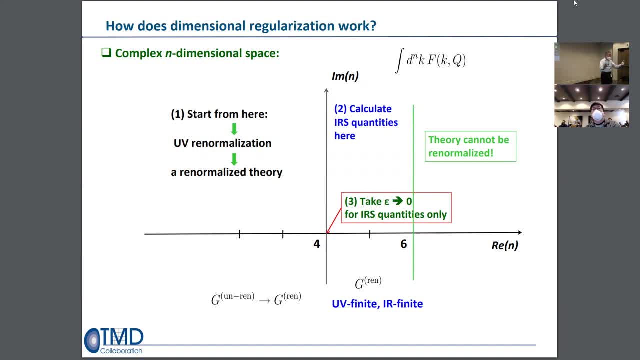 but with the regularization neither of them divergent. When I combine them together the divergent cancel. then I'm safe to go back to the limit. Epsilon is the dimension, you know, physical dimension, minus this arbitrary dimension in dimension regulation. 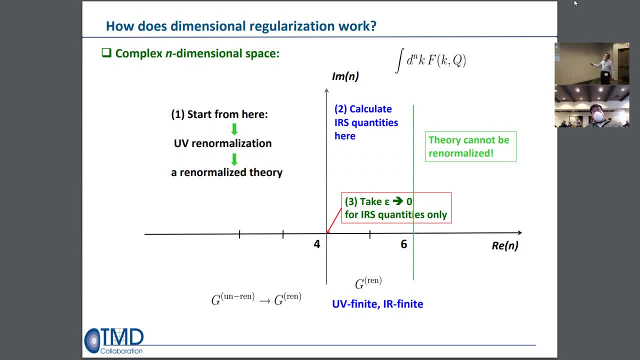 Go back to physical quantities, the physical region, But that's only for infrared safe quantities. But if you also say what if I go into this region, Well, theory have a problem, Then at least we don't have to worry about it for now. 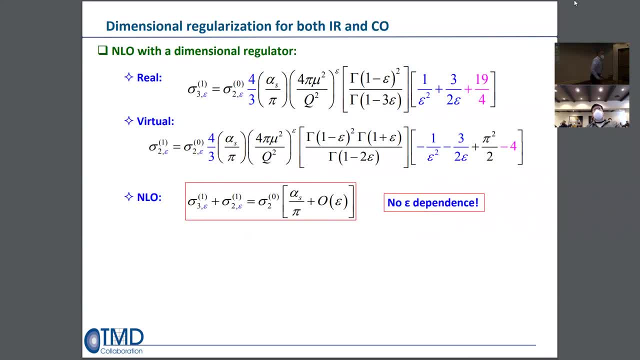 for the QCD. So I gave you example. next, leading order: I told you I did a calculation in a fixed dimension of divergence. real diagram, calculation of divergence. have both infrared and collinear, So where I can calculate in the arbitrary dimension. 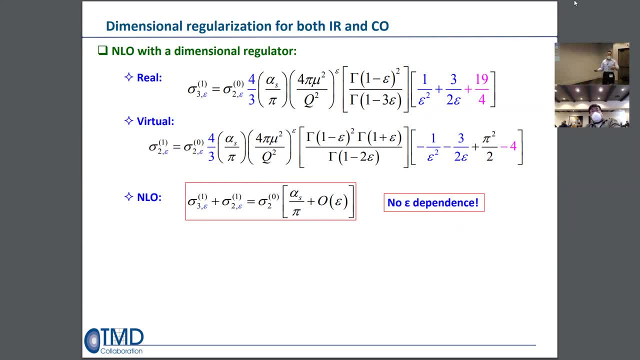 in terms of the epsilon, epsilon is a four minus I use a D dimension equal to four minus two epsilon. So in that case a real diagram is a completely finite but you can see if I take an epsilon go to zero, the real diagram. 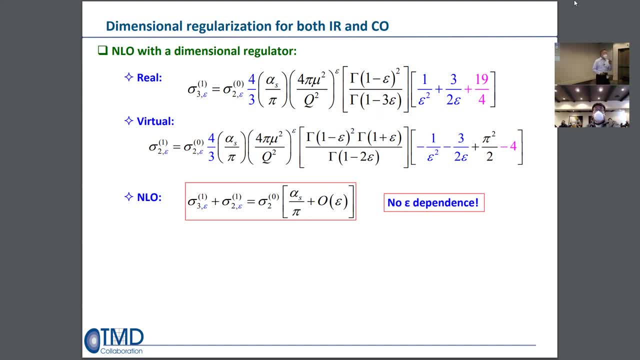 I have the power square divergence, that corresponding to the phase space. you have a both collinear and infrared divergence, So that's why you want the epsilon square. Then you also have term one of epsilon that either come from infrared divergence or collinear divergence. 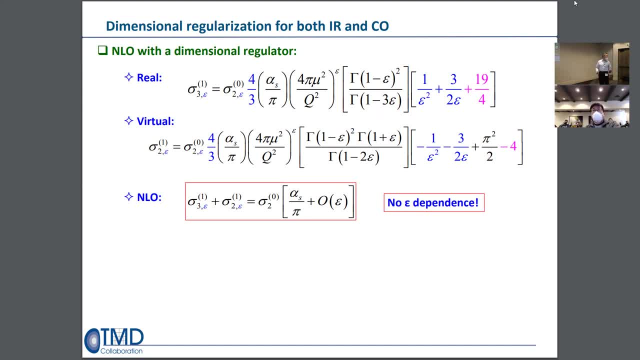 But if you regularize that, everything seems to be finite. I can do the same virtual diagram calculation in the sense of the vertex diagram root. with the root You calculate again. you have this both divergence. Now, before I'm taking dimension, go to four. 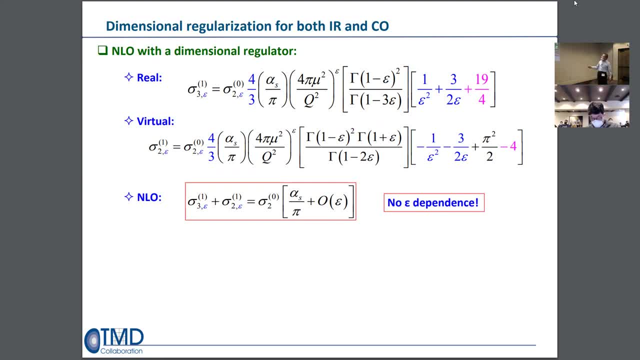 I'm going to combine them first. If I combine this real and the virtual diagram together, these two divergence are all canceled. then everything is a finite plus order, plus order of epsilon. Then this is the impressive quantity. I'm ready to take the dimension go to four. 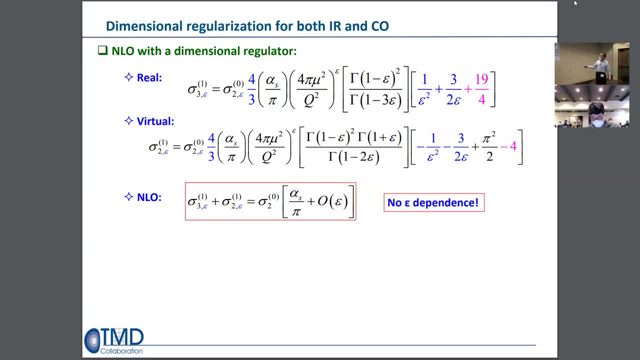 So this term be dropped, So that after the order of next leading order, everything is finite, even though individual diagram is divergent. So the total cross-section will have a leading order. Next leading order will have a leading in the sense, the real diagram. 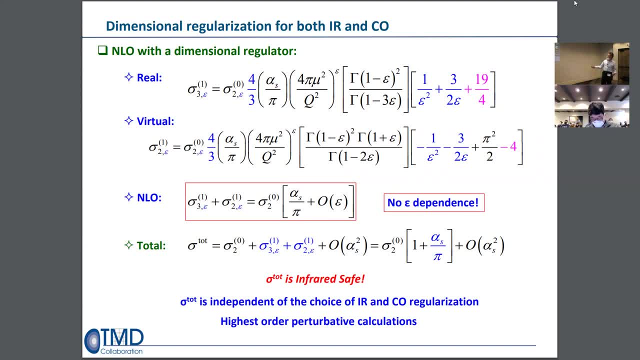 three particle final state. Virtual diagram is the same two particle final state but regularized in terms of the power of epsilon. Then you combine them together, the order of alpha square, then you end up with something completely finite. It's a total cross-section for a safe 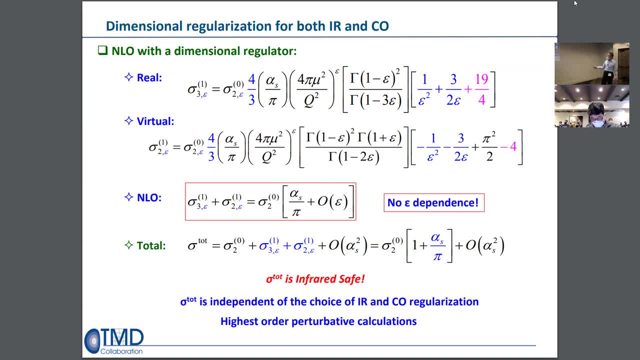 Then also the sigma total is the independent choice of the infrared and the collinear regularization. Then people have been doing this to verify order. Last knowledge, I learned at least the three loops. Then this is just one loop what I did here, But you can do this very quickly. 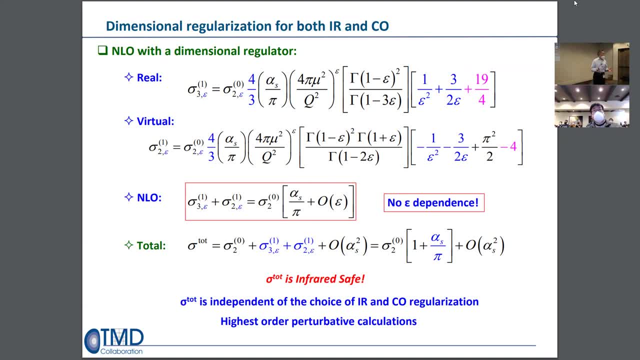 Then people find it. no divergence, everything is finite. So you know the QCD perturbations do you know as an asymptotic theory, they never really convergence. So you start a theory, have a leading order. next leading order you have a big behavior is better. 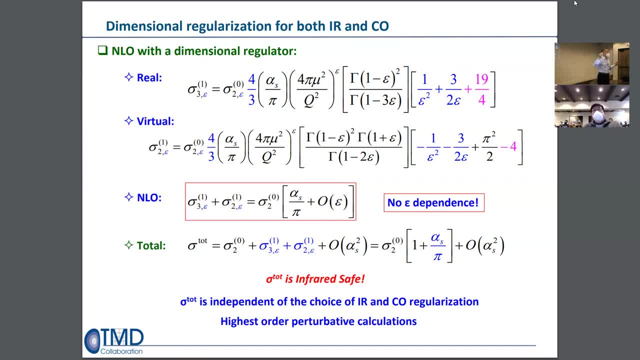 when you change the scale, because physically never know what's the renomination scale yet, So you can change the range of scale. You see, the theory has a prediction of some uncertainty. When you go to certain order you will see that uncertainty getting smaller and smaller. 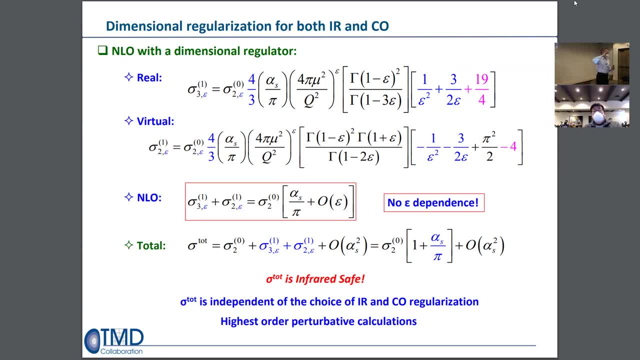 But eventually they were getting bigger. Then the theory go to asymptotic regime. So far I believe the people already go to the highest order, at least three loop, partially fourth loop They have not seen. they maybe have a little bit hint. 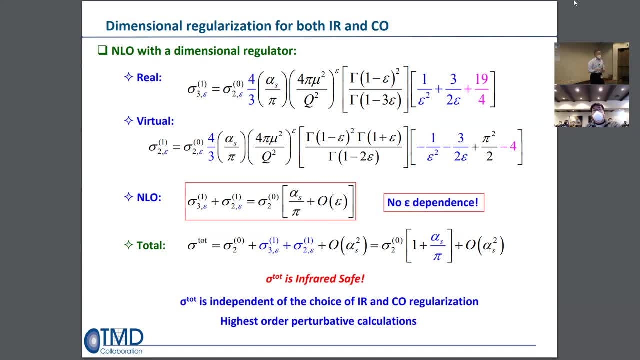 They get coefficient of, next those order become the larger. But that tells you how well behave a QCD, infrared safe quantities in perturbation theory. So that's a quantity we studied without any identified hedons, Even though the cross-section it's the same. 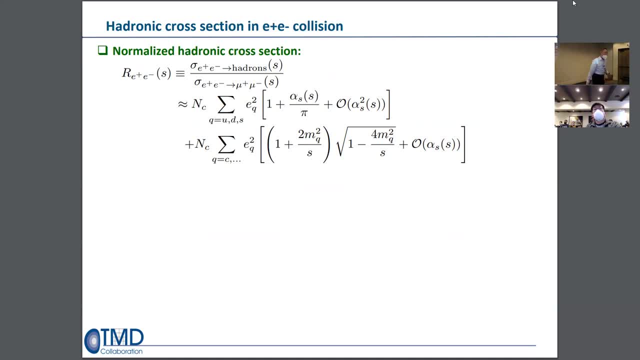 The cross-section goes to all the hedons. So how to test it? Well, I mentioned that you can measure the E plus minus to the old hedon right. Well, sometimes it's good to normalize it. They use, instead of measure, this cross-section. 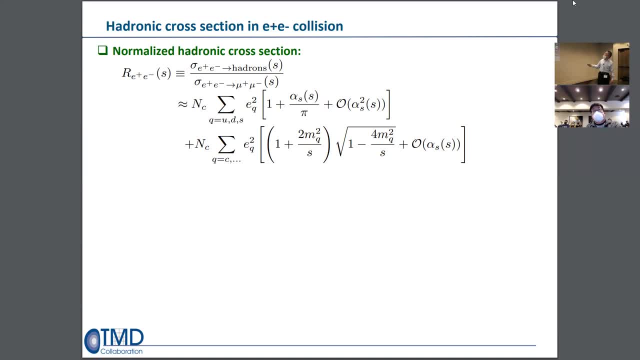 measure the ratio of cross-section E plus minus to E plus minus to mu plus mu minus. That's QED version, So take the lowest order we just calculate is order of alpha S over pi. for light bulb You can include the heavy core. 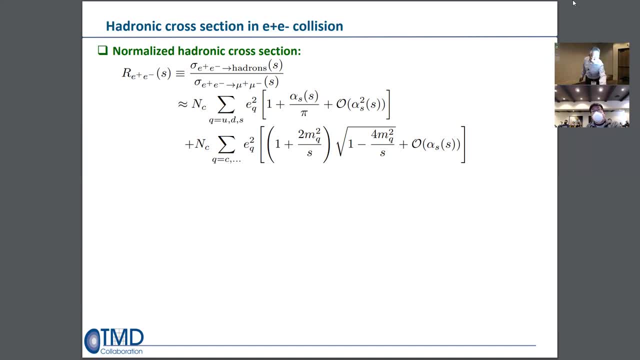 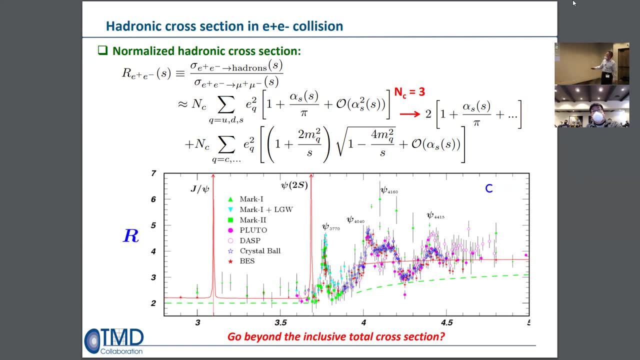 You can include all the high order. What the message is? you can do the experiment. That's what you measure in the ratio, the norm and the R? They. you would find that you can have a low energy. You have some resonance. 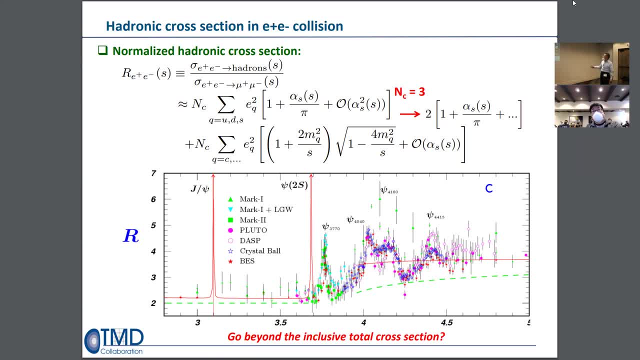 They have almost flat. Then you go to high energy. You have a more resonance than the closely flat. So what tells you is that prediction from QCD is very good. and also this: you notice they strictly proportional to NC because low energy, that's the same problem for you. 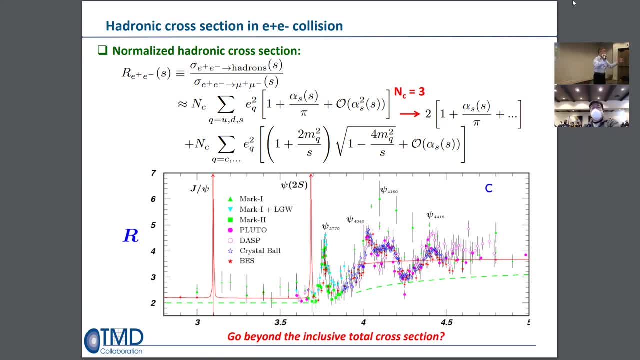 I mean this is a higher energy than the negative lowest order, the E plus minus to the Cucuba pair. You know that in the quantum mechanics cross-section proportion is some of the all, the final quantum number, of final state. 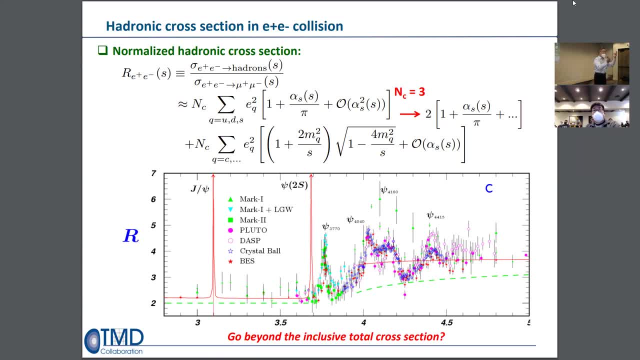 That if you go to Cucuba pair, Cucuba core carry color, they have a three color, But you don't know. imagine you can at least the three, Then experiment. this is actually probably the one of the best measurements still. 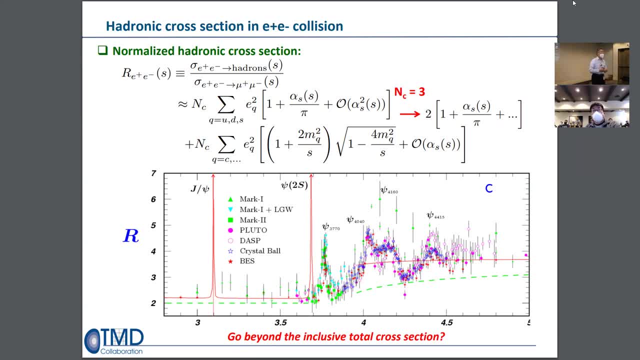 to determine what the color Color. so far from E plus minus this R measurement, the N is a 2.99, something Very good. Of course people measure three jet event, other jet things to try to test the number of colors. 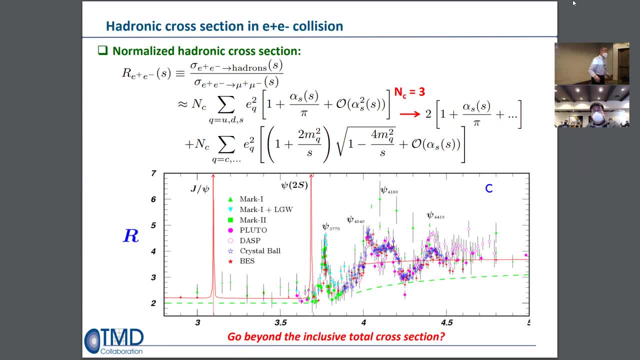 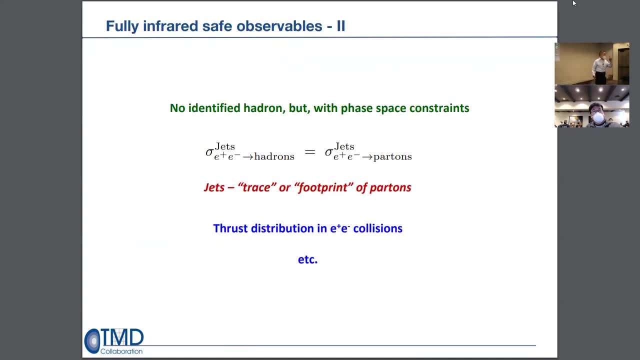 So far we still have not seen a major disagreement with N? C equal to three. With the last 20 minutes, then what I'm going to do? another example: We don't identify hydrons. Before we next lecture, we're dealing with identify hydron. 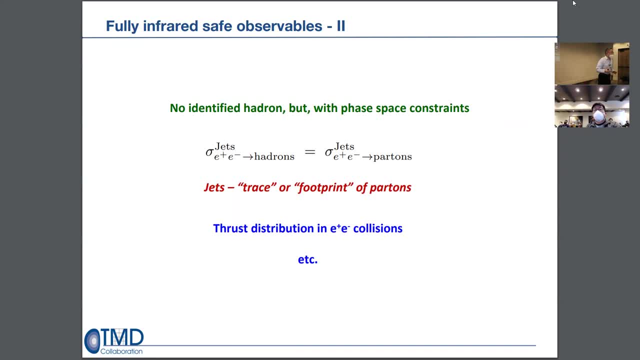 We say, well, total cross-section is good, It's sum over everything. But here I'm going to do a slight different things. So I'm going to limit the phase space. Instead of integral over all the phase space, I'm going to put the constraint of phase space. 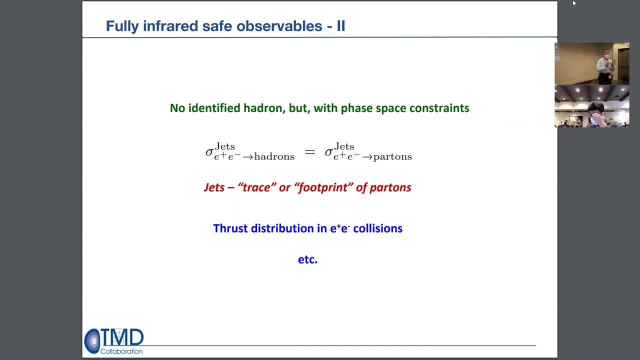 I still don't try to identify the hydrons, But put the constraint of phase space, That's exactly lead to a second example, lead to the very important observable known as a jet. So you heard a lot about jets. I'm going to give you the pictures. very probably, 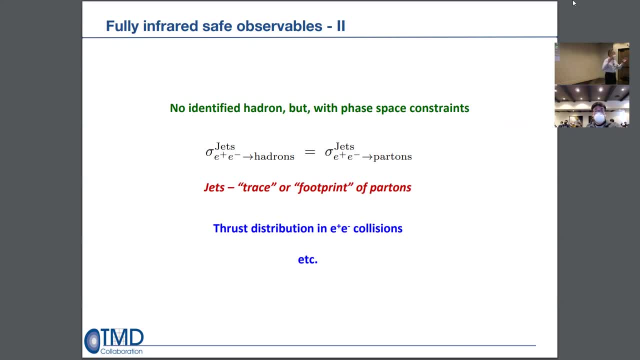 different from what you normally think, But actually it's like a total cross-section where the phase space constraint. So in that case is that jets know And the trace of footprint of pattern. You produce that e plus minus. Imagine you have a high energy collision. 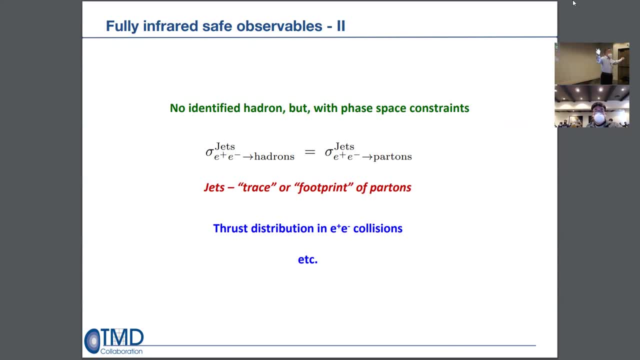 You lead to the kikuba flying away. Kikuba carry color. There must be soft interaction between them to neutralize the color. But without the color soft interaction you don't change the direction of the jet. that much So that means the events look like you. 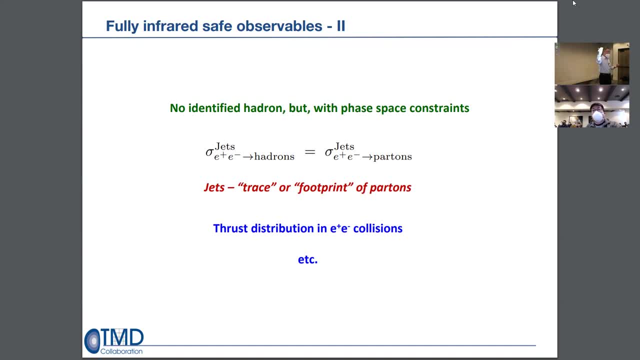 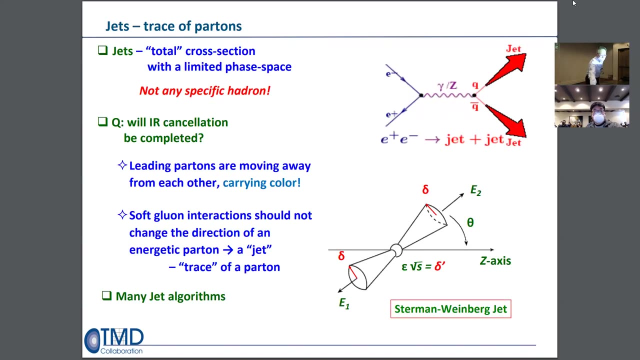 have a beam of a particle going this direction against the beam particle going opposite direction. Those are known as two jet events. Of course you can have a situation with three jets or other jets, But the question is that is this quantity perturbatively equitable, even though you have hydrogen involved? 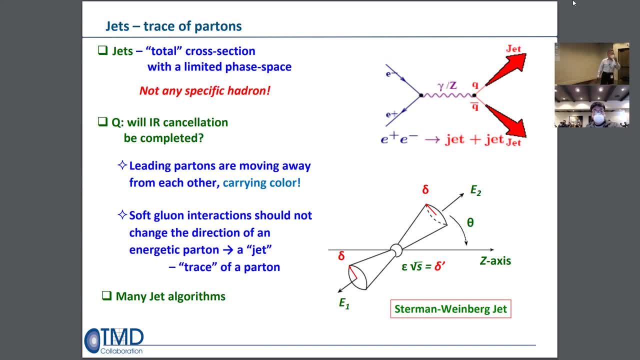 Answer is yes, Then this is not trivial because you have a constraint on the phase space. So in that case, the idea you can have jet, in the sense I define a total cross-section with a limited phase space- Then also the idea that the very first one, 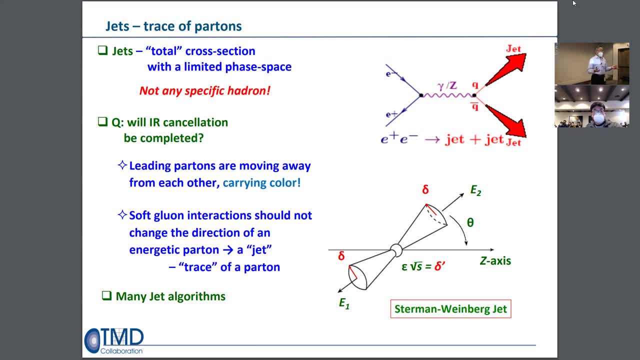 is the diverged cancellation From the last example I showed. if you calculate the total cross-section where the leading order are two particles flying away, that's fine, Everything is finite. But if you go to the next order you have a kikuba plus gruon. 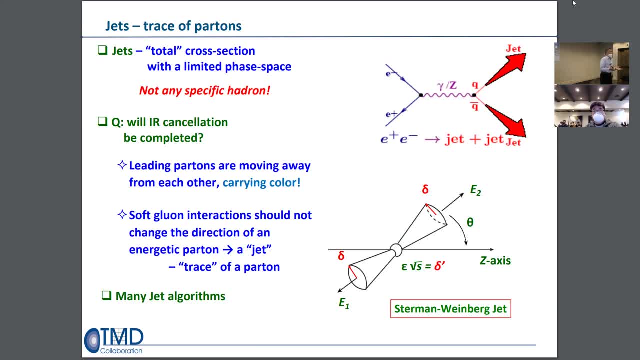 When an integral phase space gruon you notice there's a divergence. Then the divergence tells you you have to have virtual diagram to cancel. But imagine what's a virtual diagram. E plus, minus go to kikuba pair Virtual diagram. 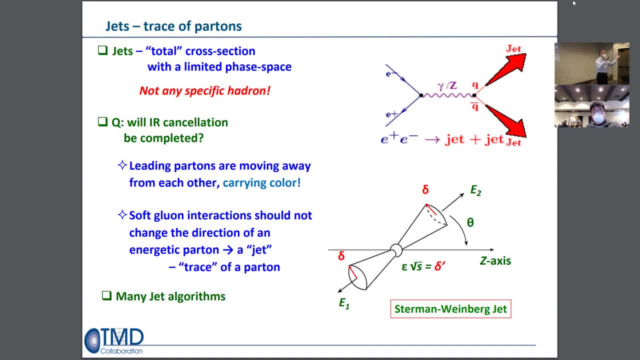 Virtual diagram means a gruon loop. That gruon does not effect by any phase space constraint. They are just like a lost order, Those two quark kikuba, in the final state just a gruon. So you immediately realize when you apply the phase space. 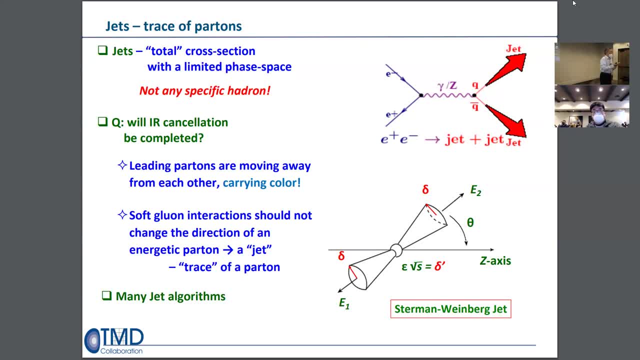 constraint you only impact the real diver Because real diver go this way then another gruon radiate. You always say gruon have to go to along the quark that end up with the jet. So the phase space constraint only effect the real diagram. 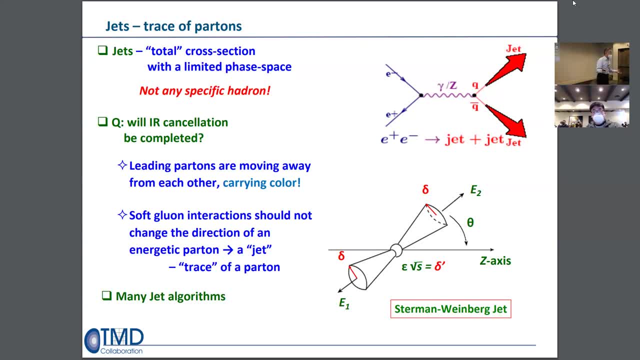 but not the virtual diagram. How can you have that cancellation? That was exactly the debate many, many years ago That led to the famous paper by Sturman and Wamburg known as Sturman-Wamburg jet. So definition of a jet cross-section. 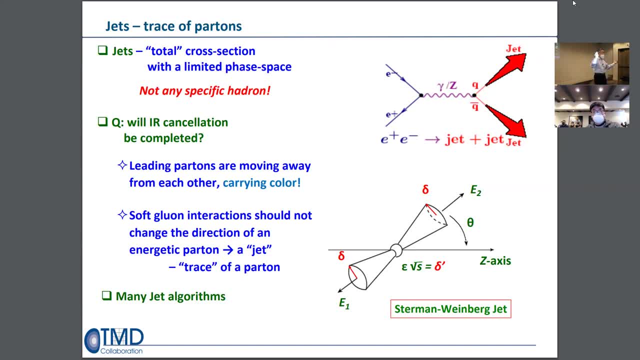 is not just say a two beam of a particle. You have to have a two beam of a particle plus the full beam. You have to have a phase space over the full pie Because it takes the resolution. You never can see the very soft particle in all the full pie. 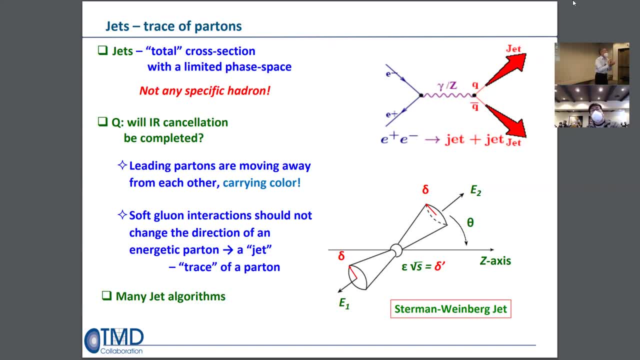 So you have to go over the phase space, that part of the phase space, So you allow, you have cancellation between infrared and the virtual diagram So that paper- a lot of people know the history was first proposed- was rejected by physical review letters. 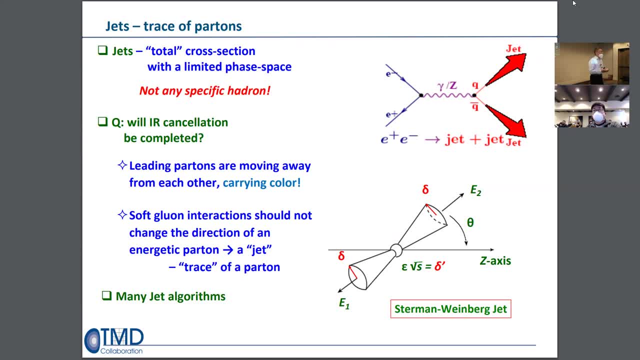 many times. They eventually started with George Sturman. They end up with a. well, it's natural. Then, when George gave a talk, Steve Wamburg got very interested. They worked together, improved the paper, rejected again Because this is nonsense right. 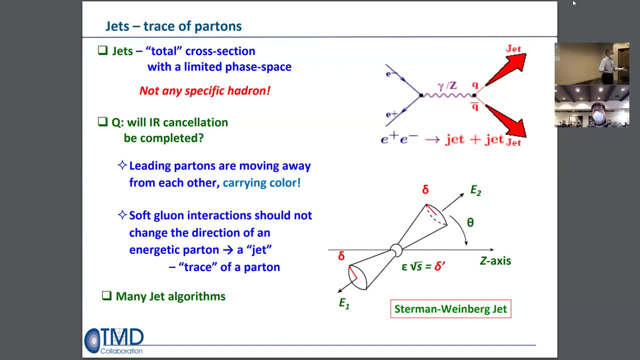 How can you have this kind of phase space constraint? You end up but still claim cancellation take place. Well, eventually the paper got published. It's interesting. Go to website, take a look at that paper So you can calculate those results. 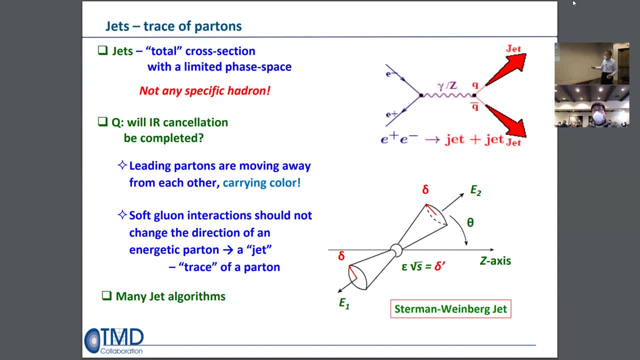 in just a couple of hours You can do it. All the calculations I'll show you for a moment. So this leads to the real life of the whole business of jet physics. They tell you they give you a footprint of quarks. 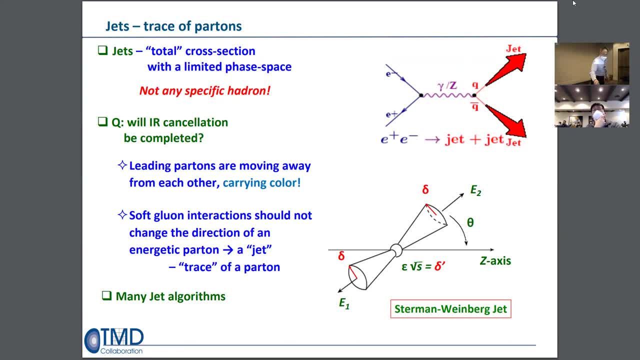 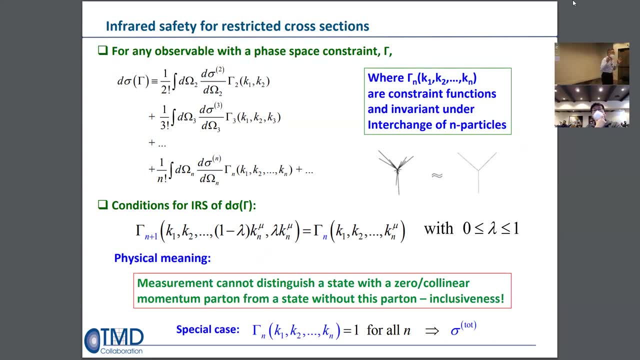 We never see quarks go on real, But from the structure you give you the footprint of the quarks dynamics. But what is the theory behind it? How can this kind of cancellation between real and virtual can take place? to all the information theory? 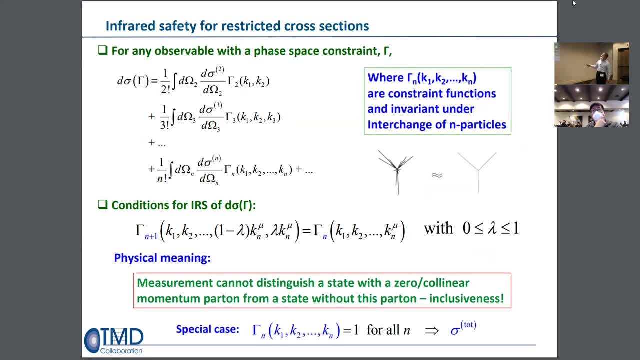 So constraint. then imagine the cross-section is that you have a two particle final state, three particle final state, any number of particles final state. in the QCD You put the constraint function gamma with number of particles. If the constraint function equal to 1, sum all together. 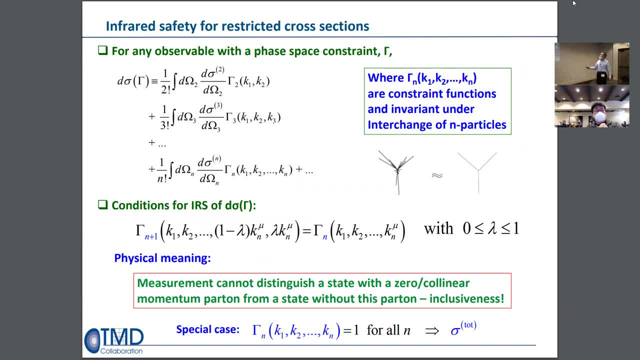 that's total cross-section. That's infrasate. Now you add a constraint function. You have to demonstrate the cancellation still take place. The requirement on this is exactly. you have this gamma 2 particle final state. You have a constraint function adding one more particle. 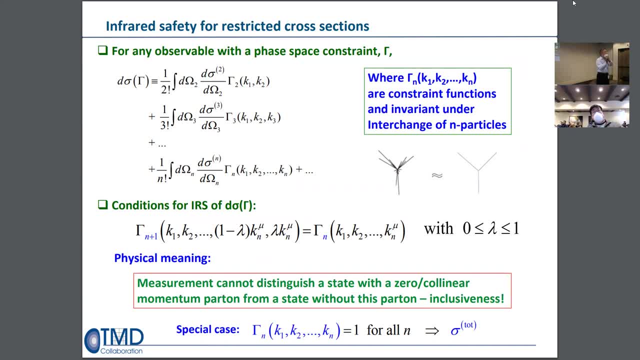 If the one more particle is a polynomial to any one of the early particle or the particle added has zero momentum. that means you could not tell the difference, This situation, the one more particle versus the particle without this actual particle. so that's the exact conditions. 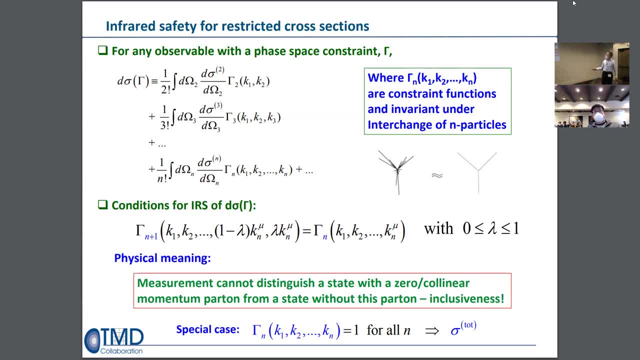 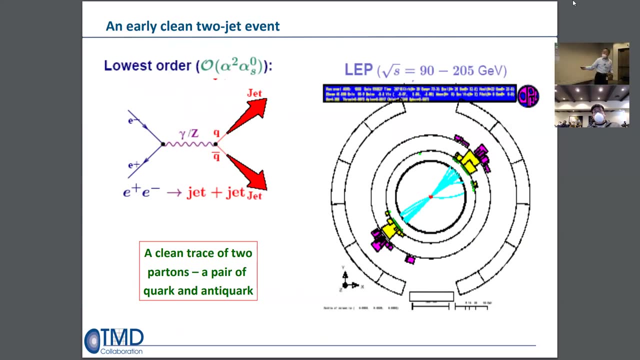 If the constraint function satisfies this condition, then this Observable where the phase space constraint is actually infrasate. So I gave you a quick example. So the two jets, they actually see the experiment. This is very quick. Then, from the left, you can see the two jets. 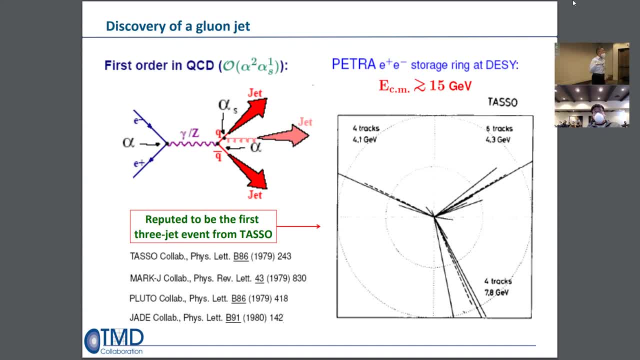 Then you can see the three jets. This particle is very early, no actual claim to be discovery of the gluon, because you see the third jet, the Kq bar plus gluon, Then you can have a higher nature Left 2.. 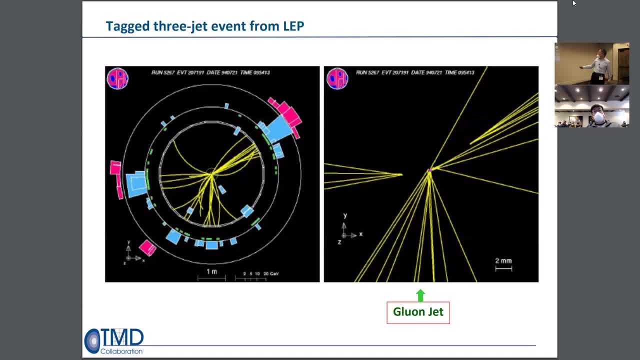 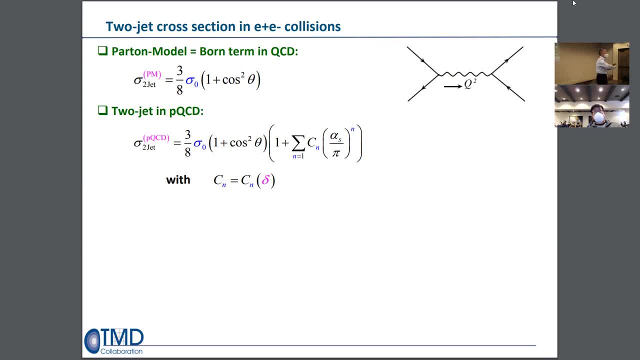 You can see the much more particle in the final state It's still a bigger fat jet, no other gluon jet. Question the calculation Again. let's start lowest order: E plus minus 2, Kq bar pair. You did a calculation before. 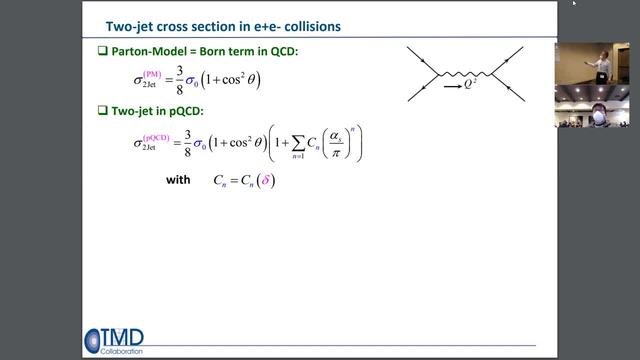 That's fine. It's a part-time model picture. It's finite. It has an angle distribution. So all two jets of the higher order will be correction in the power of s. For total cross-section you have to go to the angle. 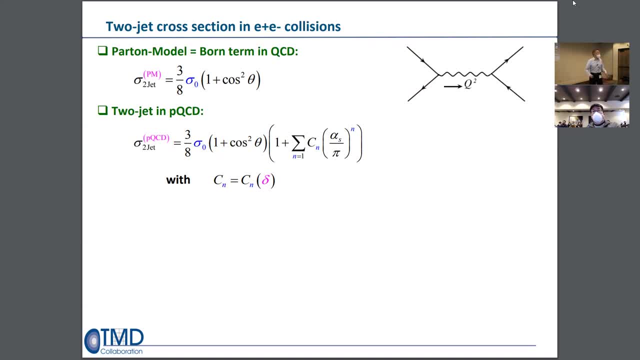 And this is just out of our festival public. But now you have phase space constraint. You really constrain the phase space. What happened? Well, if you do it, the trick George Sturman and Steve Weinberger did, saying, instead of calculate, 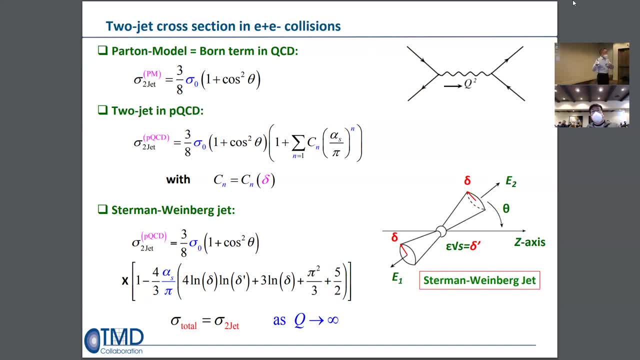 I have a real diagram- momentum go to 0, then virtual diagram. It's complicated, It's hard because you're dealing with infinity. The trick is I define the cross-section as a total cross-section Minus the event, not jet light. 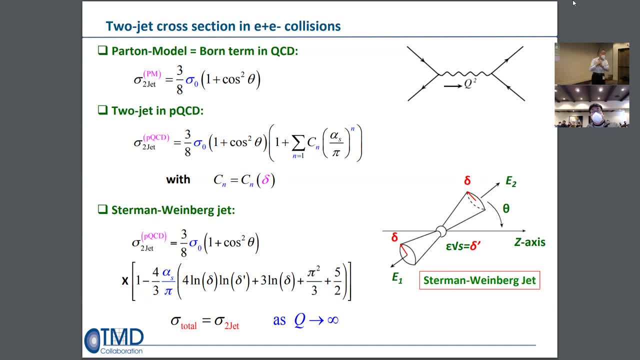 So minus event when the third particle go in the large angle. So that means that calculation is much simpler. So when you do that you eventually find the cross-section. two jet, one loop, correction. The order bias with the angle between. this is the energy. 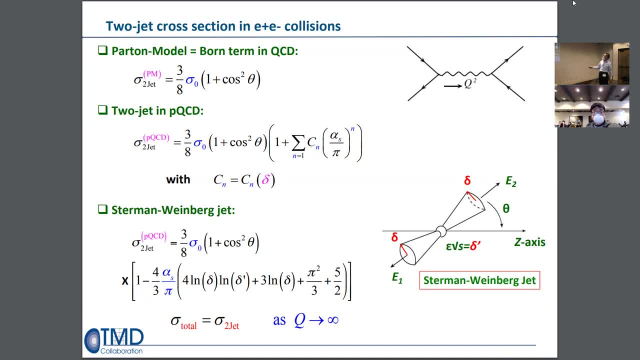 allowed. the detector never see everything. So that's a 4 pi. You needed to cancel the infrared divergence. Then this is the collinear divergence, infrared divergence. This is a 4 pi. You need to cancel the infrared divergence. 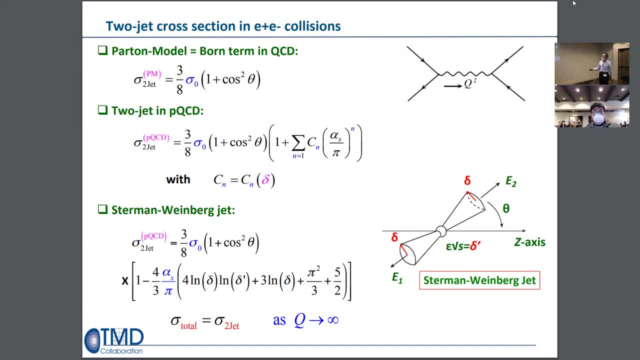 Then this is the collinear divergence, infrared divergence. This is a 4 pi. This is a 4 pi. You need to cancel the collinear divergence. You have finite pi. So that was the calculation. You can do very quickly. 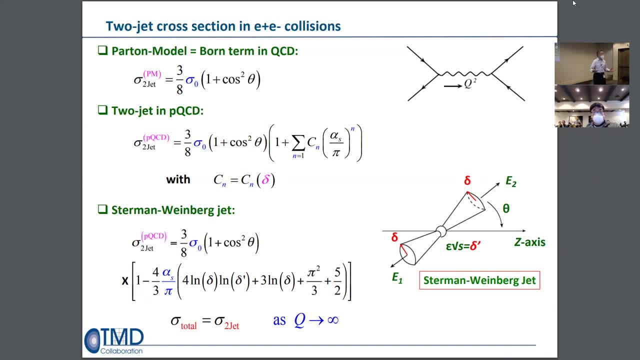 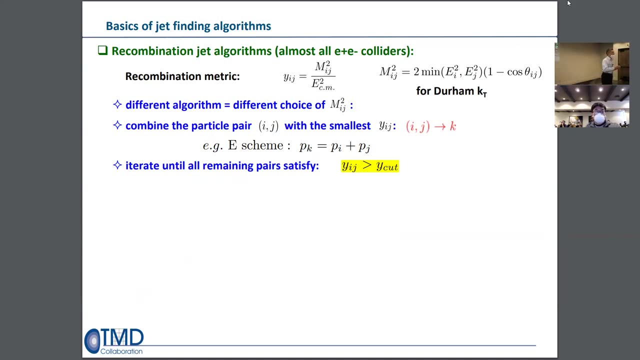 You know the total cross-section already, so you only calculate subtraction term, which you say. the third particle is outside the jet cone definitions. It's a finite calculation. You can do it. So now life becomes the real jet, physics becomes the real important observable at the LHC. 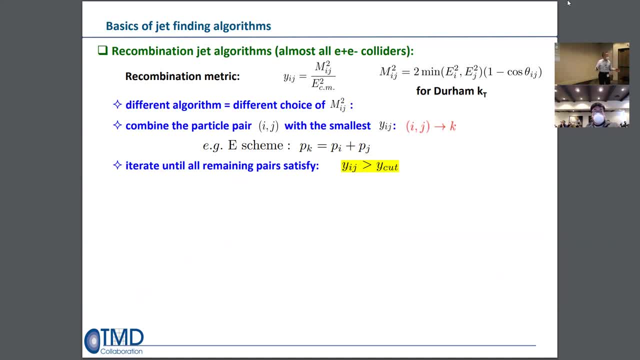 and many other observables. So the example is what the algorithm to define jet? Because experimentally you see a bunch of hydrons, Theories dealing with a bunch of patterns, Now how you link it together, And also you can see plus minus. you start with no hydron. 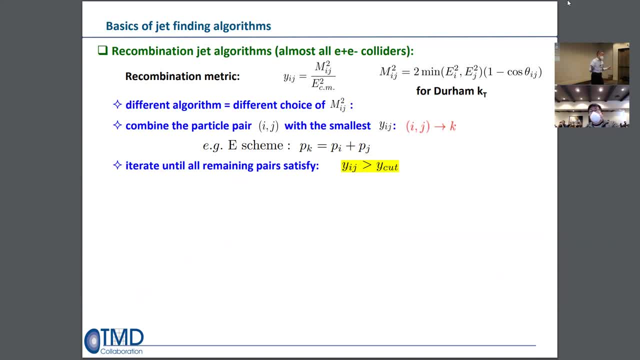 You just tracked all the final state hydron. You organize it into the jet structure. But the hydron hydron like LTC. you cannot do that. You start with a hydron that you know have a bunch of the hydron going to final state. 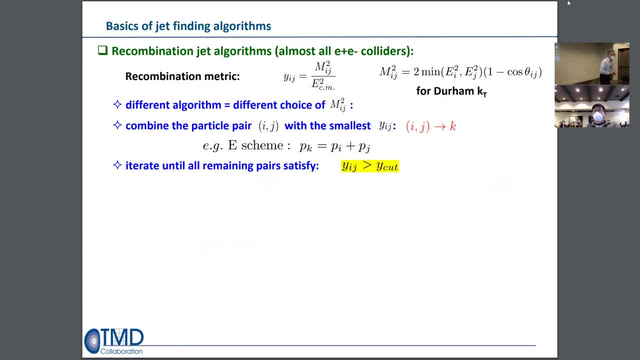 You cannot integral 4 pi to organize your event. So there are two classes of jet algorithms you should know. One is purely from E plus minus. The idea is there is no hydron to start. If I stay in the center mass frame, I have no hydron to start with. 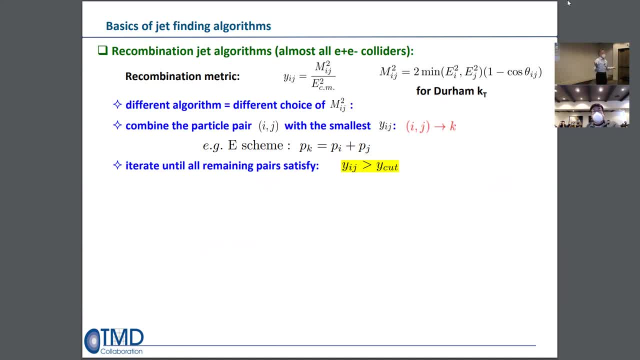 But the final state has lots of hydrons in the 4 pi phase space. What I'm going to do? I combine any two particles together according to a criterion. Add them together. If they're close enough, become the one effective particle. 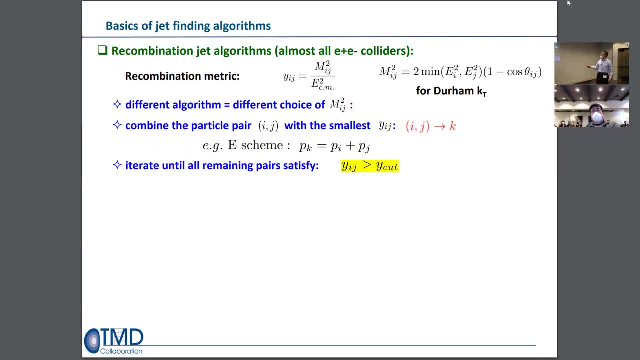 So you keep combining them. Now you end up with, say, if the invariant mass of a 2 is larger than some value you defined by hand early, say Y-cut. So that defines the number. By changing the Y-cut your event could have a 2-jet event or 3-jet event, 4-jet event, depending on how you choose that. 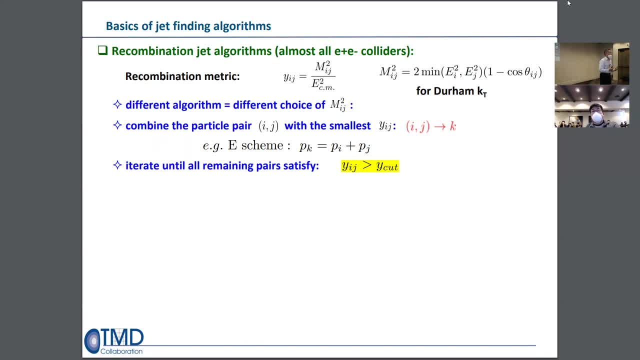 So you can. you see it's ambiguous. Who cares? Well, take advantage of that. You can test your theory. Apply to the event. You can test your theory if the theory is consistent with that. So that's it. 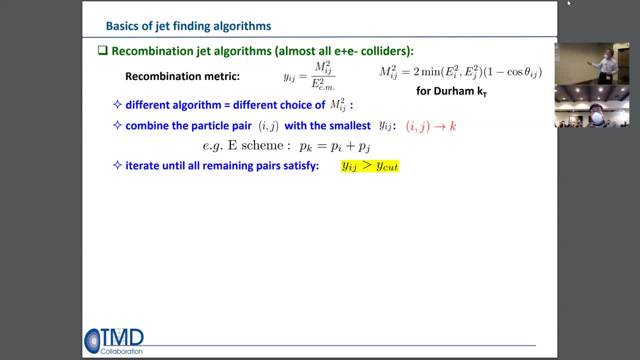 So that's it. So now we're doing the recombination of the jet algorithm, mostly for E plus minus. Then, depending on how you combine, you have different algorithms. I only gave one here, known as Durant algorithm. There are many different type of algorithms in the early days. 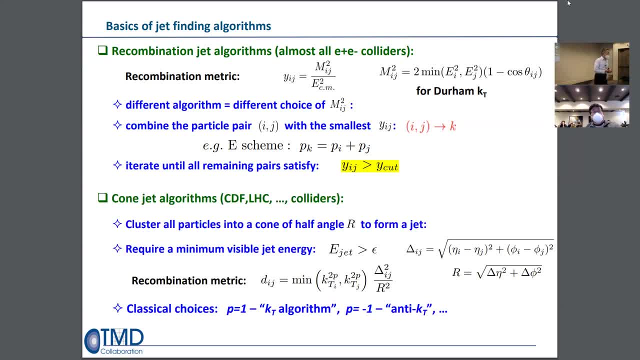 But now we're doing mostly the hydron-hydron collision. In a hydron-hydron collision you don't have 4 pi phase space Because you start with the hydrons. So in that case we often concentrate on the produced particle in the large transverse momentum. 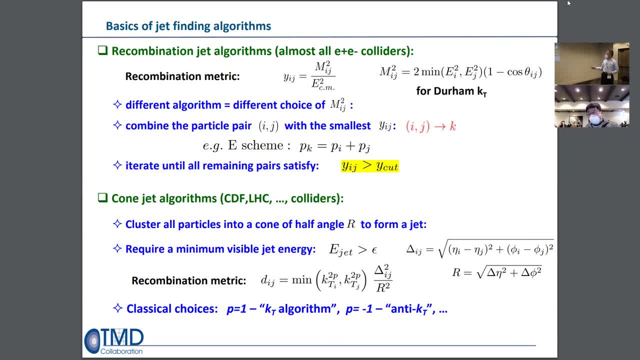 So in that case you define the so-called the combined things in terms of the repetitive difference of two particles, That's longitude, direction and azimuthal angle difference between the two particles. So that's a typical hydronic configuration of particle coming up. 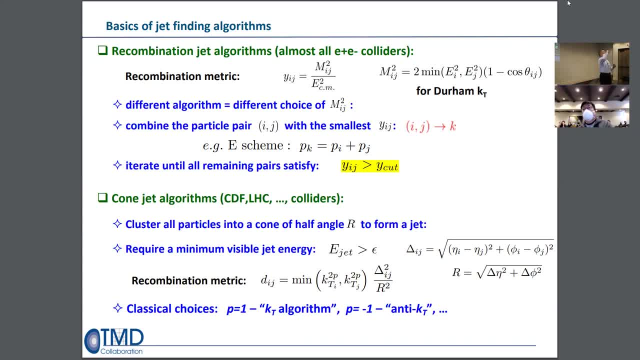 You have a transverse momentum, repetitive longitude momentum, azimuthal angle, So you combine the two if they're close enough. based on this criteria, say, you define R, you define that, So this is the wall of the criterion- and combine with some kind of fractional power- p. 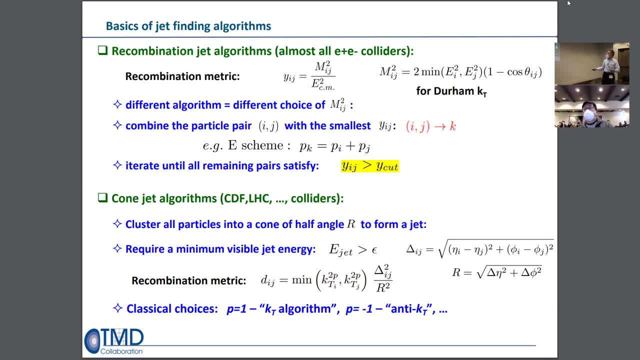 Now, if the p is equal, to choose to be one known as the KT algorithm. if you choose p equal to minus, one is known as the anti-KT algorithm. You heard about it. So basic idea is you produce a lot of particle, a lot of hydron in the final state, but I'm going to construct observable without depend on any specific hydron. 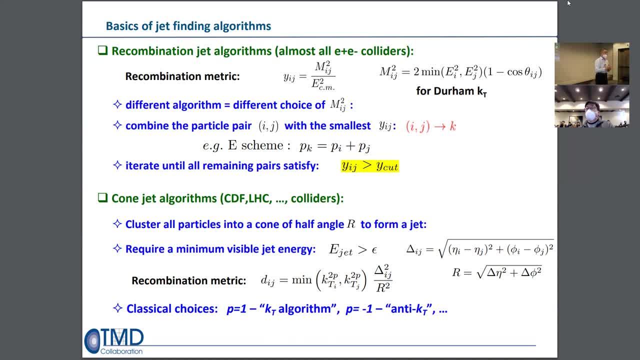 Only thing is I concentrate on some phase space construction- That quantity is perturbative, calculable. So that's the second perturbative calculable quantity I gave to you without introduce any, say, distribution or non-perturbative physics, even though you have a constraint. 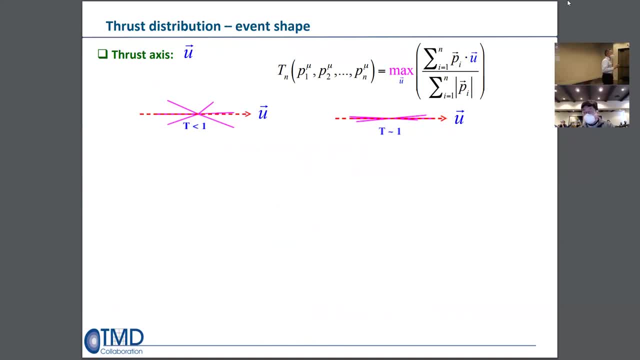 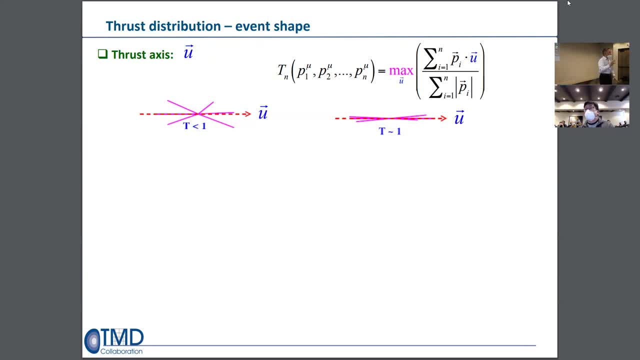 Like a two jet or three jets, But there are also. the part of observable was infra-state. especially in the early days of E plus minus, There was a lot of data. People are not sure. what can we learn from that? So one of the observable is known as thrust. 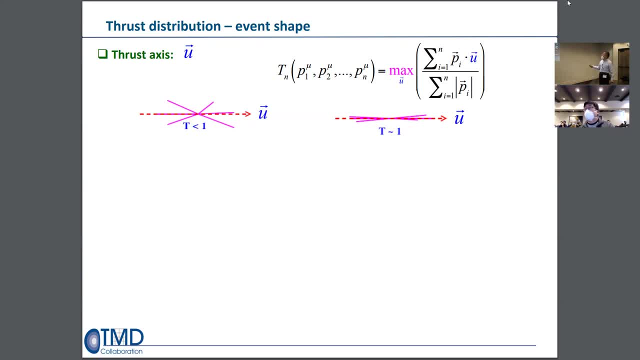 Thrust is a defined as, say. it's a very complicated definition. You have n particle. final state You say: I choose any individual particle. Dot product is a direct. It's a direction Now to maximize this quantity. they, when they knew that the direct T less than one, much less than one, the event look like spherical symmetry. 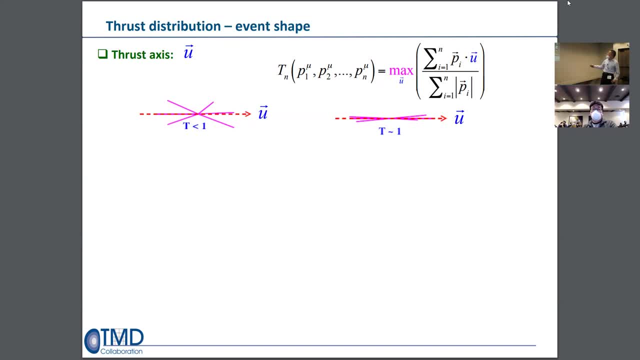 When the T close to one that means the event look like a two jets. So by different choice of T you are manipulating or you're controlling the event shape. The next lecture: Jan Stueck. he actually proposed the jetonism. 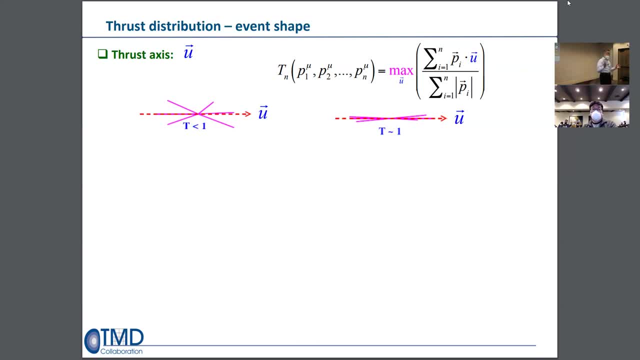 which is another one observable, relate to event shape. so those are the third example i gave to you know, as event shape. so, but here is a homework, just i'm done. yeah, okay, the homework. then this line i given here to prove, with this constraint function you define constraint function. 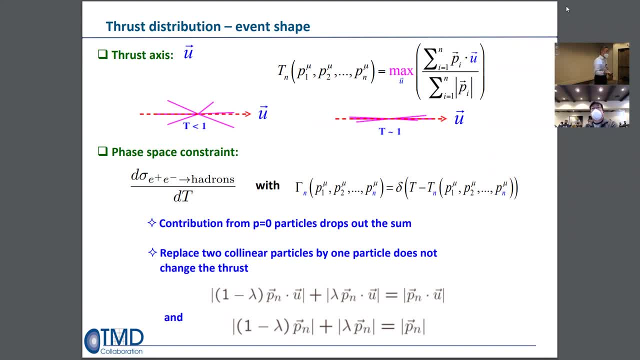 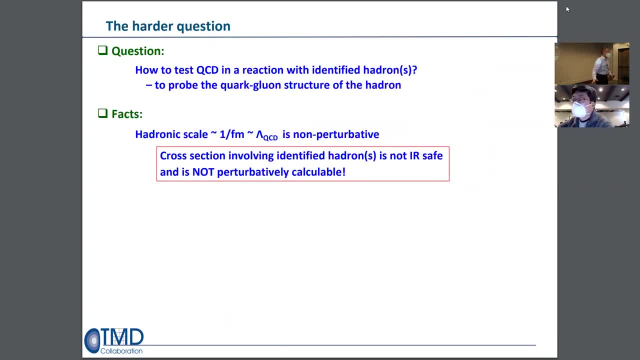 i'll give you a criteria before what the observable infrared say. with this constraint function, you can easily prove that thrust is impressive. well, after all, the example of the hydra observed: hydronic observable without identify hydrons. you see a lot of hydrons but we don't know any detail of the head. but if we want to understand, 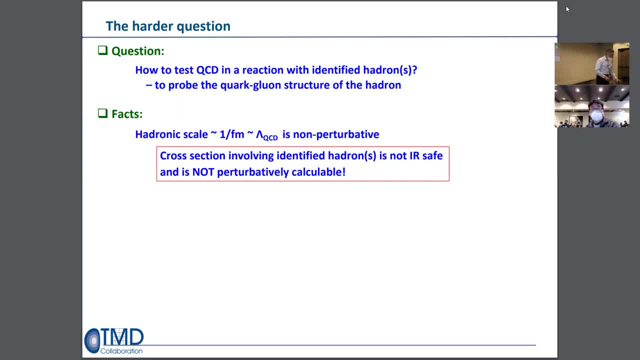 the physics or structure of a hydron. we'd like to learn more at that. so that's exactly the question i'm going to ask. the whole further questions is how to test the qcd in a reaction with identifying hydrons. that will give you a chance to understand the internal structure of hydrons. 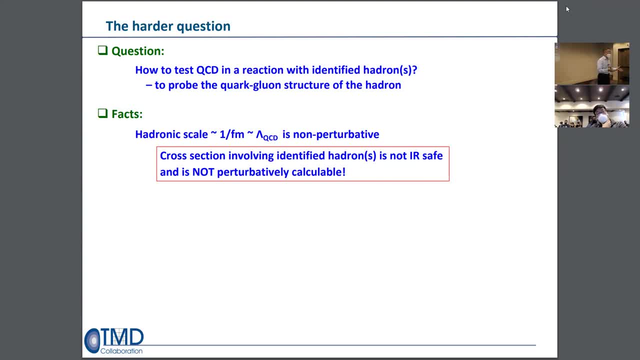 so far those are observable, wonderful. you test the qc dynamics but you don't learn anything about details inside hydra. so we want to do that. so that's the challenge. and i told you anything with the identity hydron is not particularly categorable directly. so the 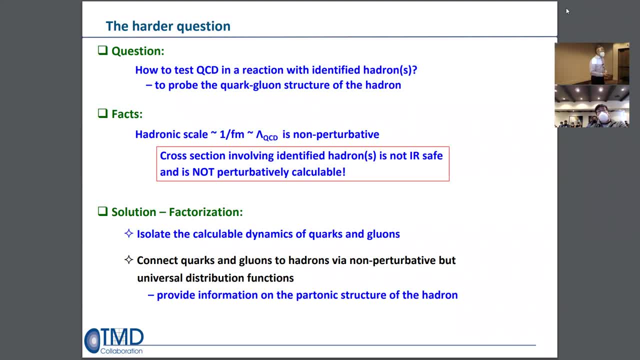 solution is the factorization. that's why we do next lectures. let me stop here for this lecture. thank you, this is a real big introduction. if you're in the room and have a question, uh, you're welcome. all right, you might need to move closer to this microphone, so the people on zoom will take care of you. the people on zoom will like. 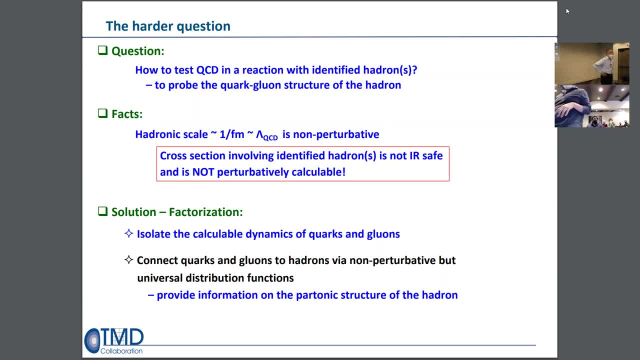 to ask questions. uh, i'll give you an opportunity a moment. let's type the question in the chat questions. you might be just, there's an echo between. so i had a question about, like the very beginning when you were talking about, uh, how you could simultaneously diagonalize two of the generators in su3. my question was: can you? 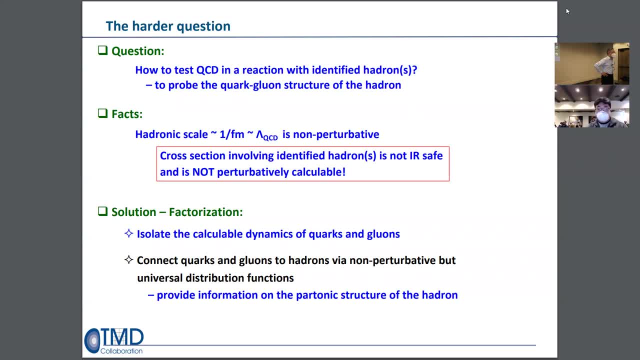 prove that without taking a specific representation first? uh, in principle, yes, there is two independent diagonal. uh, onders in del sigma global system of the ideal scale elements. when i say matrix, in that case, yes, we can discuss in detail how to prove that. two for sq3: okay, yeah, but those are the very convenient a choice, those representation. 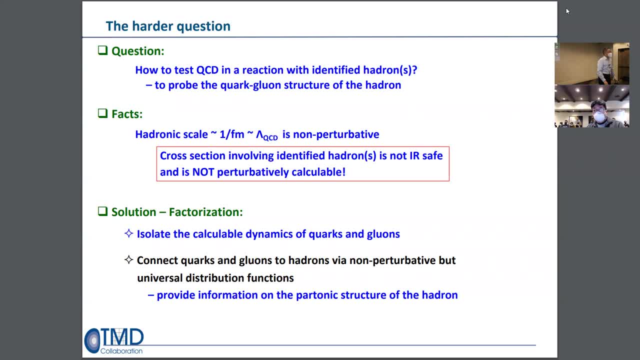 corresponding my state is o 1001. that means that there's no, at least for if you assume su3 or the particles behave in some representation of su3, then there's not going to be any wildcards where you couldn't simultaneously measure isospin and i�. 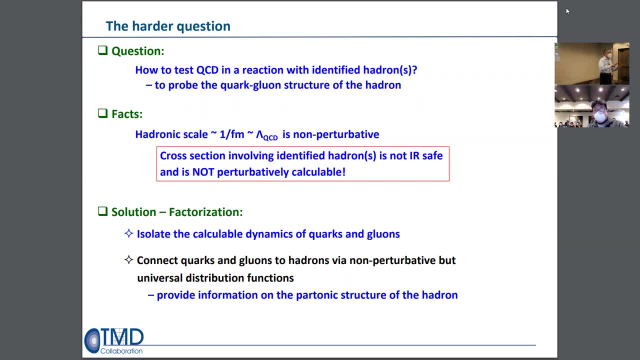 charge at the same time it's. it's all over the. the states labeled by two quantum numbers, whether it's a hypercharge or the isospin, or superposition of those two. that's fine, they're too independent, but they happen. the isospin and hypercharge is very. 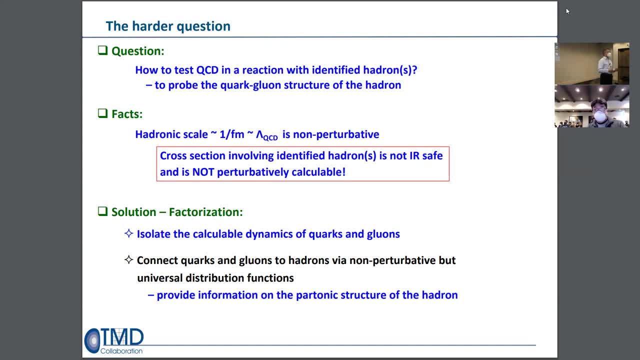 convenient, especially isospin, because you can separate your state, the proton, neutron, in the different isospin state. that has a great advantage. you choose isospin as your quantum number, okay, yeah, i have a question too. i don't know if they can hear me from here. 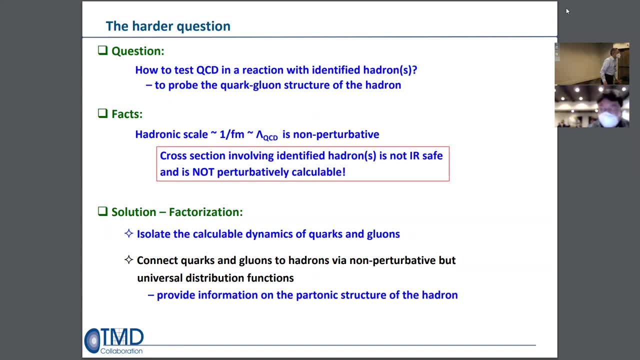 okay, yeah, when you were talking about the two- yes, cross section in plus t minus. uh, you were talking about how we have, like this c coefficient depending on delta for the judge functions and my question is: we can understand the equation as a matching coefficient between the. i don't know. 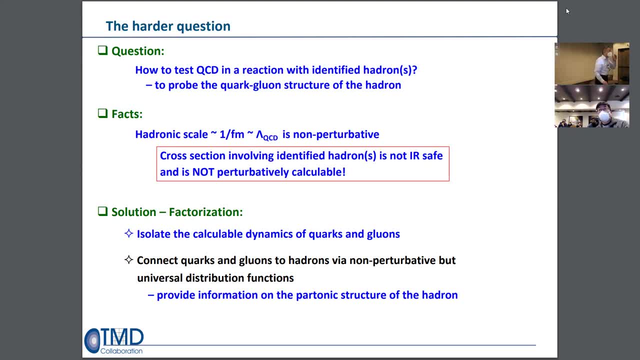 oh, i, i actually honestly i didn't hear exactly clear, because maybe mascara didn't hear very clearly. so let me say, you say that two primates have to have. yeah, in that, define the one, the stoneman when they were jet, yeah, the physics behind that. i have to choose the one parameter. 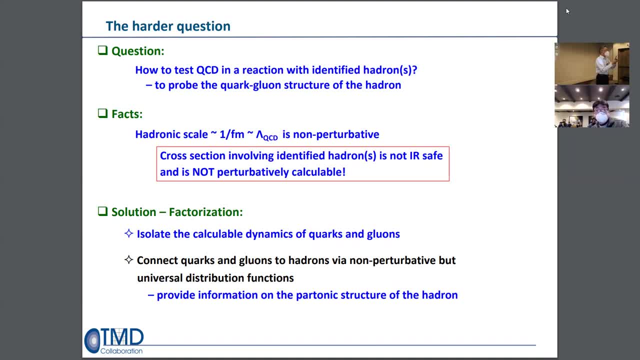 means i have to have sufficient cone size. so that means the collinear divergence will be inclusive, yeah, integrate over within the cone size. so then then cancel the collinear division. third one is the energy resolution of the all the four pi. a second one that tells you because. 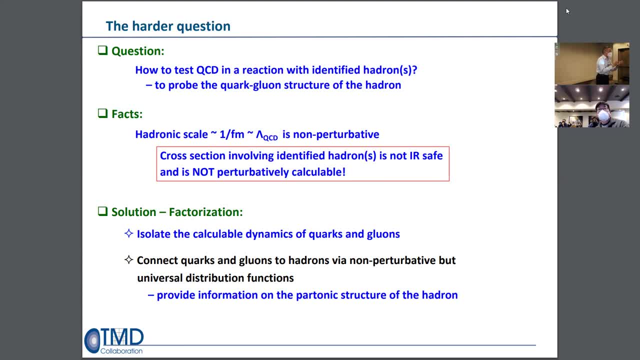 my detector i cannot see any particle below. they have gv. so when you calculate the in a feminine diagram within that region- not whether the collinear or the real diagram, radiation or the virtual diagram- you have to integrate the four pi so they can cancel the infrared divergence. 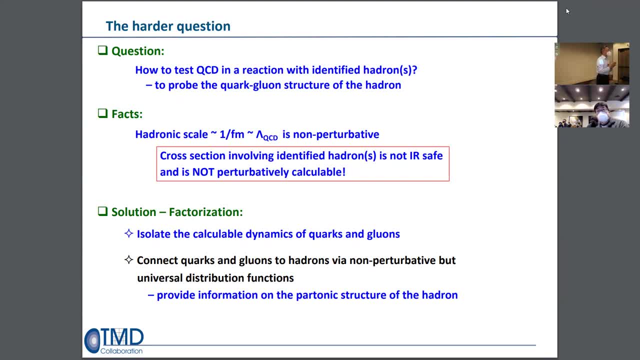 so those two parameters needed is exactly to help you to cancel the infrared divergence and the community divergence. the physics, that for total cross-section- because inclusive enough you never see sufficient detail- the real collinear they just all canceled. it's a, it's a unitarity, but 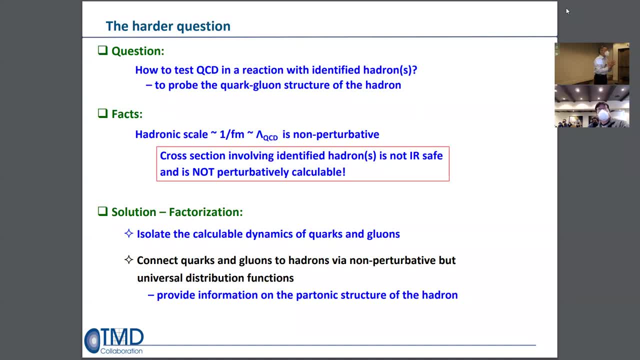 if you do that with the phase space constraint- but i make sure my constraint is not tight enough so that in the collinear region and the infrared region still inclusive enough because i can resolve, cannot resolve them- you have to integrate all the phase space so they cancel. yeah, so that's a physics behind it, okay, okay, yeah, thank you. any questions from anyone on? 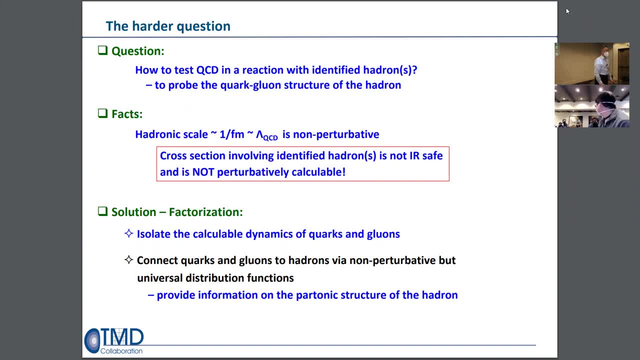 zoom or andrew asked another question. um, yes, um, my other question tried to do with when you were defining dimensional regularization and you were, uh, you combined two separate like partial cross sections and then you showed that the epsilon is canceled and then you let that go to zero. it looked like some of 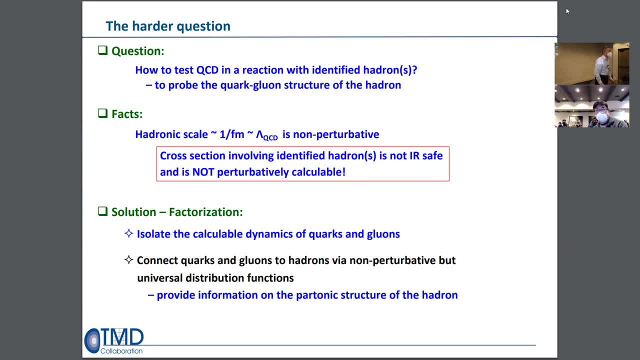 the finite pieces were gone as well. is that just uh around your like subtraction scheme or did they cancel and i missed it? no, finest finite piece is important. that's your order of our rfs corrections. it could be possible the finite piece equal to zero in whatever scheme you choose. you just have a. 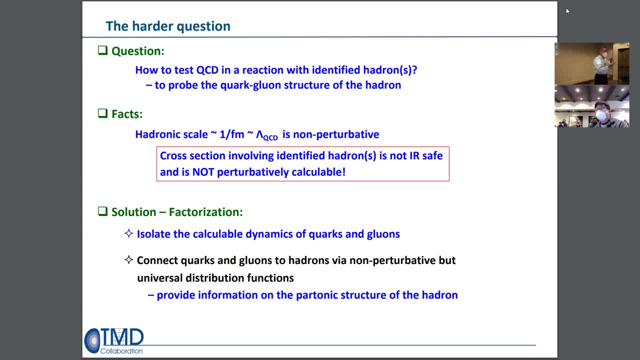 perturbation theory, you don't have the next linear correction. but if the finite piece is not zero, that means that's your factory, the finite correction to your leading to your total cross-section. then also, if you continue, i say the finite piece is so big, like uh instead of r.